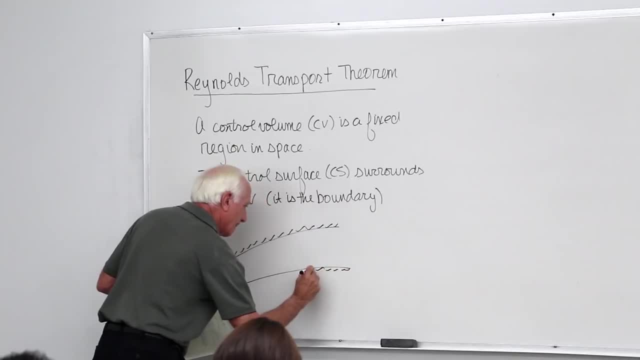 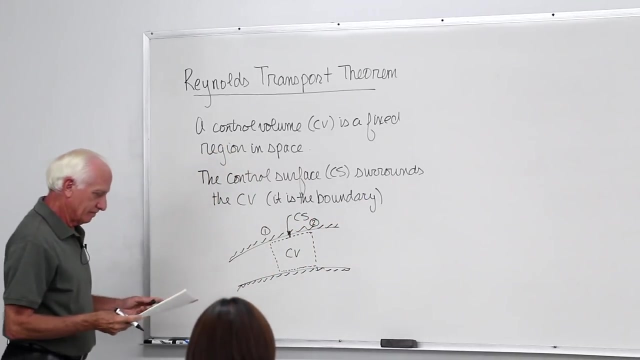 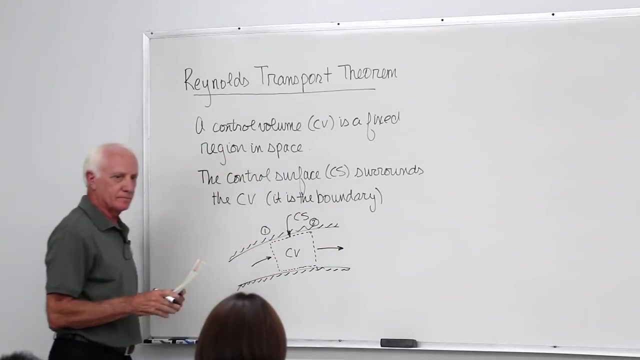 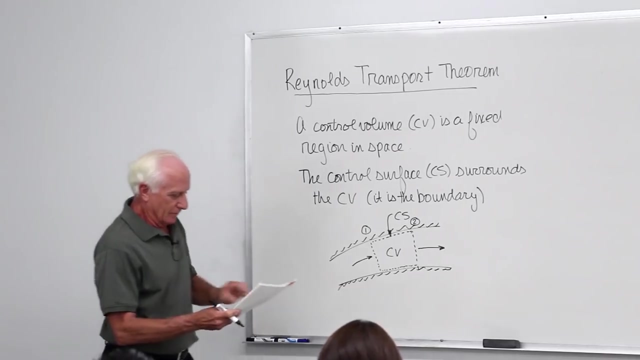 on both sides And we'll identify by a dash line a control volume. The control surface is the boundary. We could call this, for instance, point one and this point two, And maybe flow enters at one and flow comes out at two, And we could also draw that like this: Take that control line. 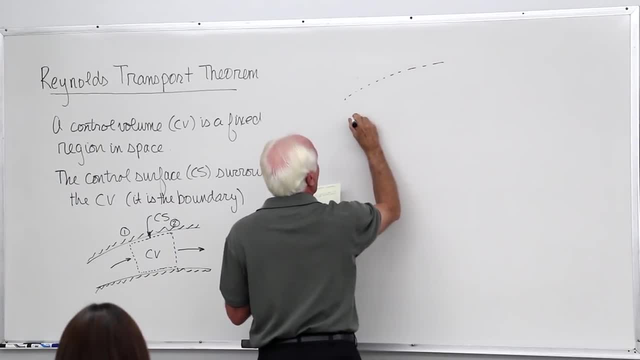 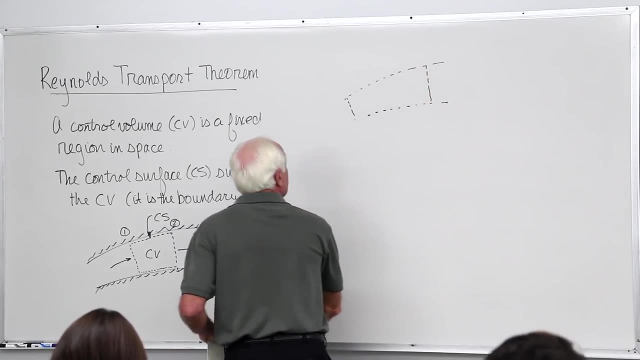 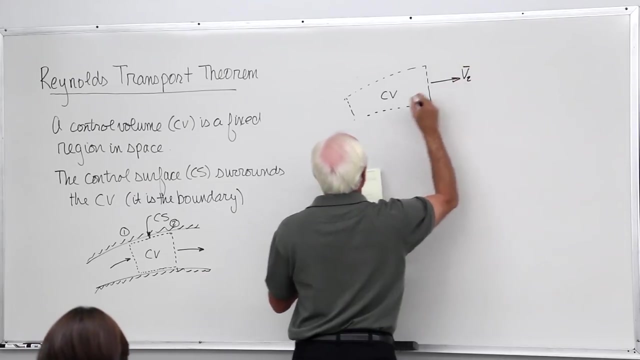 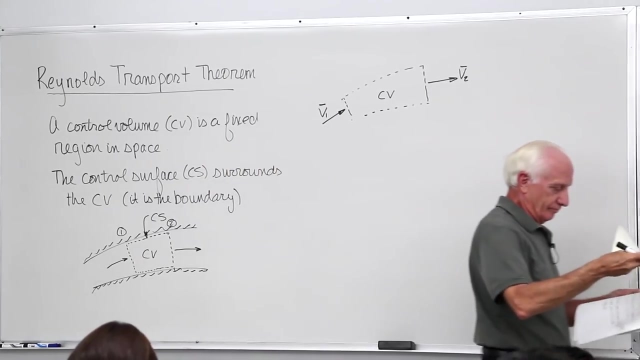 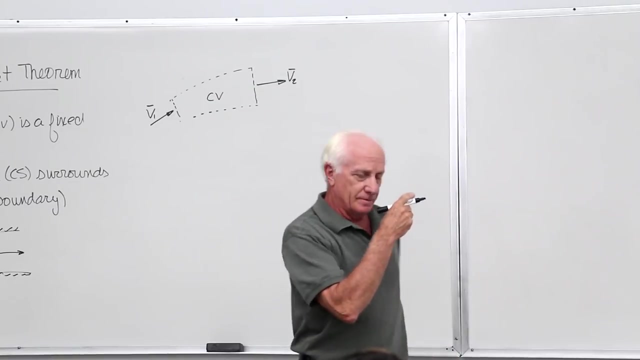 out and draw it like this Or it might look something like this: So this is our control volume And we could have velocity coming out here. This would be V2.. This would be V1.. I'll do a side calculation over here just to. I'm going to use that calculation. 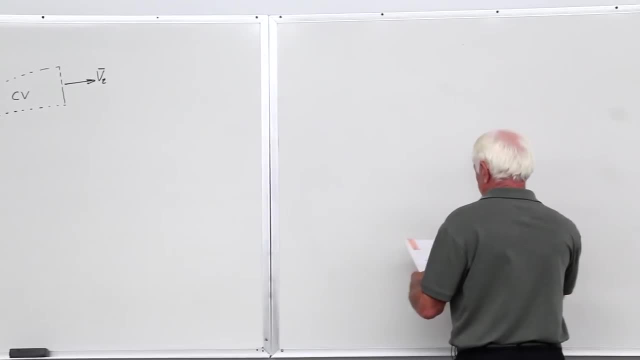 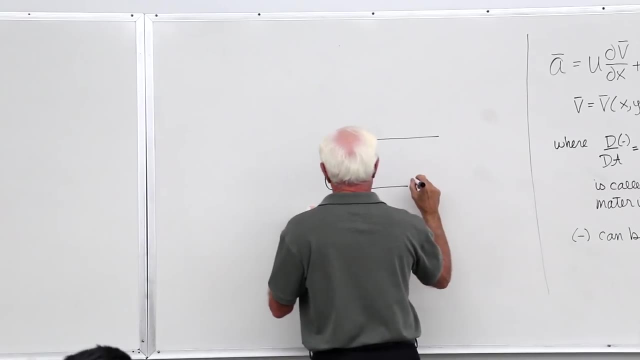 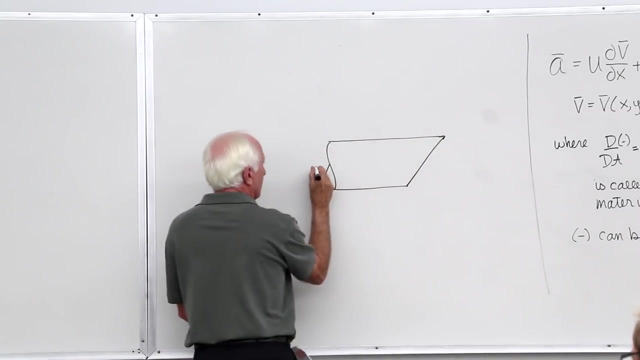 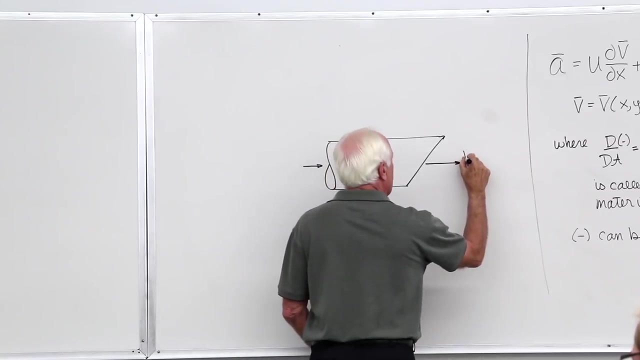 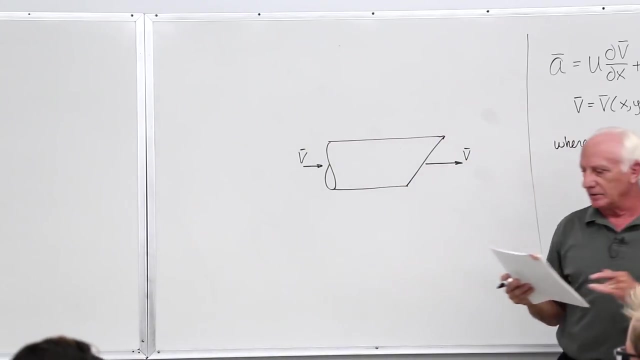 in this derivation over here. So let's look at this real quick so you get an idea of what we're doing there. Let's say there's a pipe here and we have flow coming in and flow going out, And we'll just label that V. The pipe's cut at an angle, The angle that it makes. 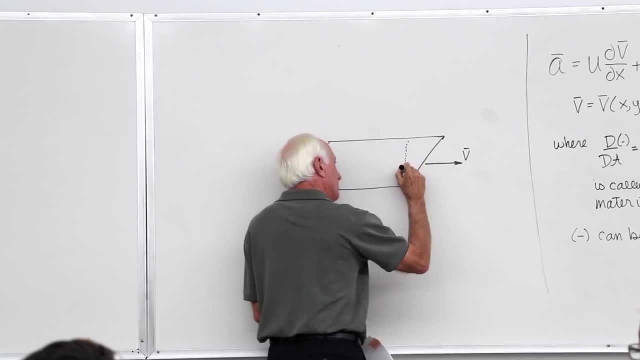 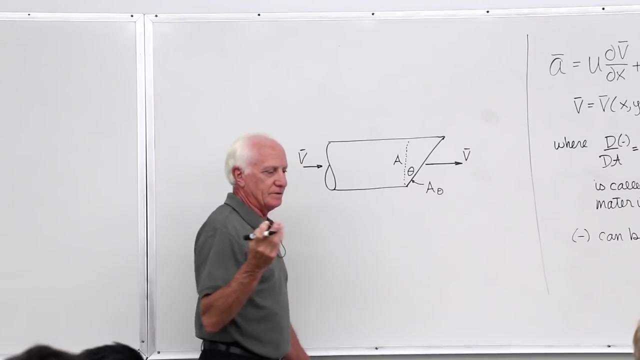 with this is theta. We're going to call this area right here A And we're going to call this inclined area A. theta A is the cross section area of the pipe. So if you took a piece of PVC pipe, cut it at a 45 degree angle and let water run through it, The water's 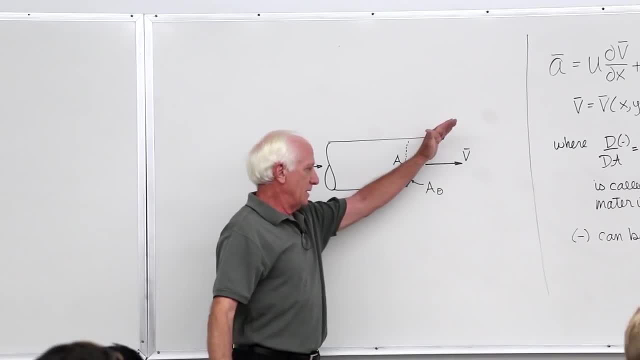 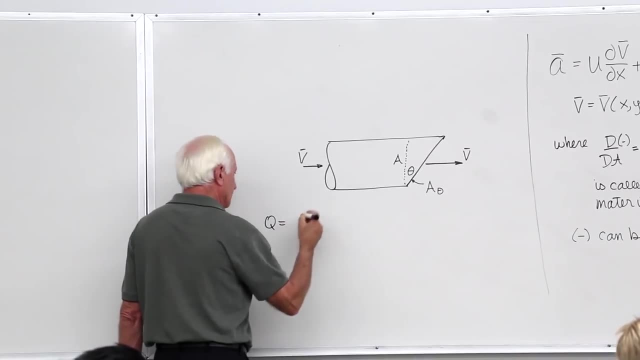 going to come out just like this, But the area's at the diagonal. like that. The flow rate for this Q would be equal to V times A Cross-sectional area Velocity. We mentioned this back way. you know we had Q equal V times A M dot. 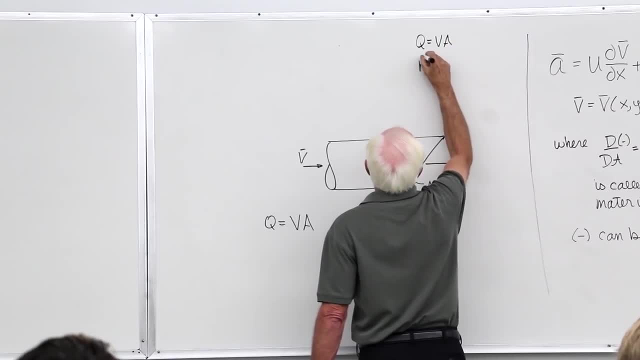 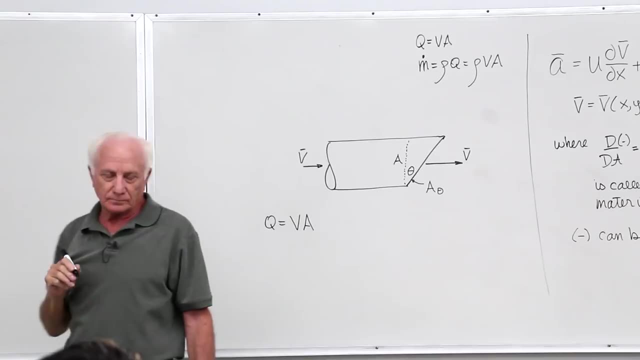 equal O times Q. We had R minus A but you have to balance both of these in and you would say if we set that to time that would be going to be V times A, But you times Q equal rho VA. So we've talked about that earlier in class. So the 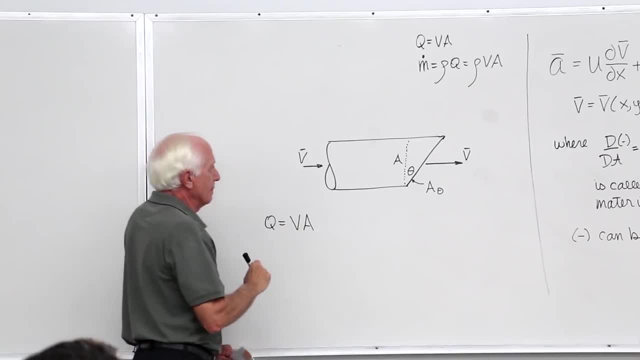 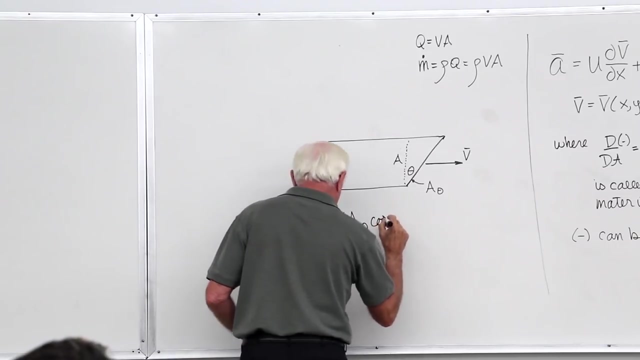 volume of the flow rate Q equal the average velocity times the area. Okay, let's rewrite this thing a little bit. Write it in terms of A theta, Get rid of A theta, So A theta times the cosine of theta- Same thing, Same thing. I'll do a. 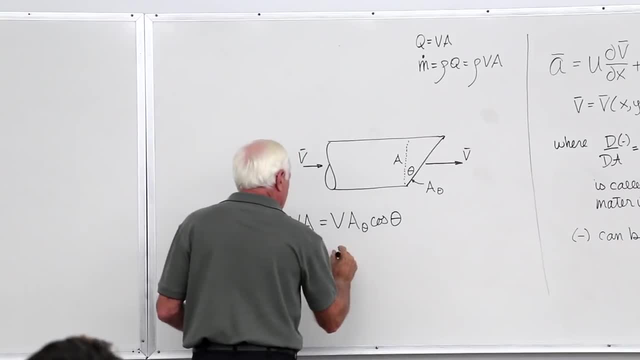 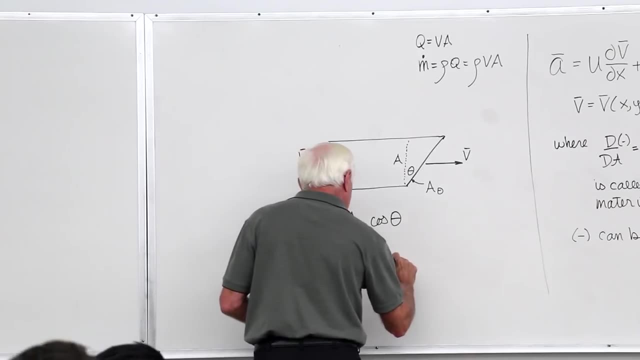 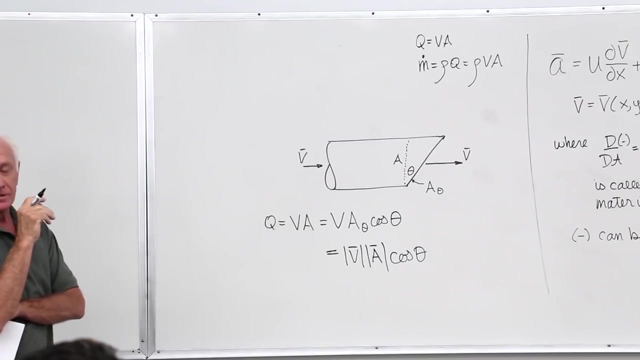 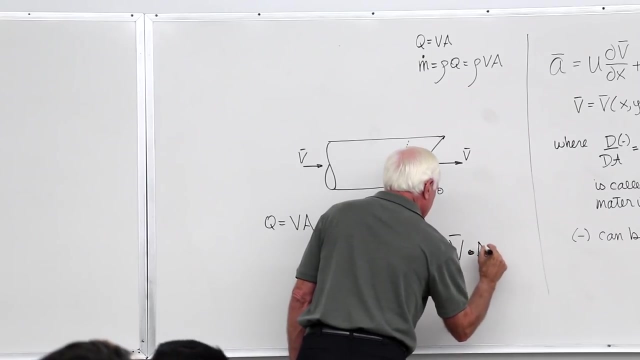 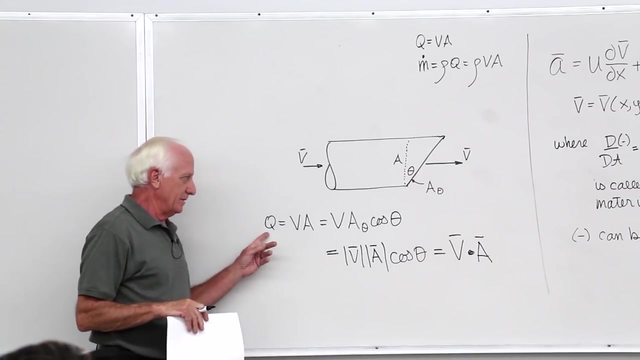 little right triangle there. This guy right here looks something like this: Magnitude B, magnitude A times the cosine of theta. That looks like the dot product. Okay. So if we want to deal with the flow rate Q, it's the. 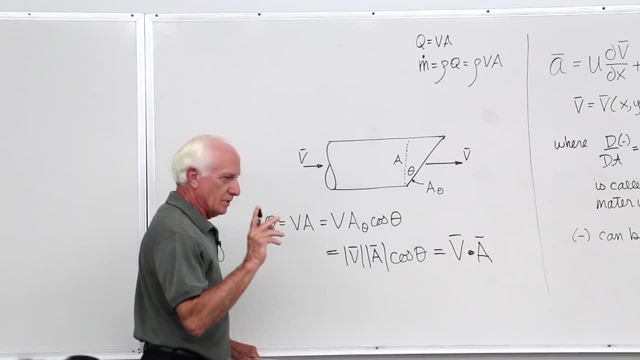 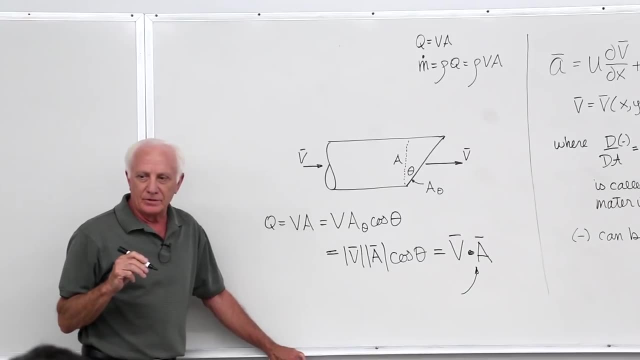 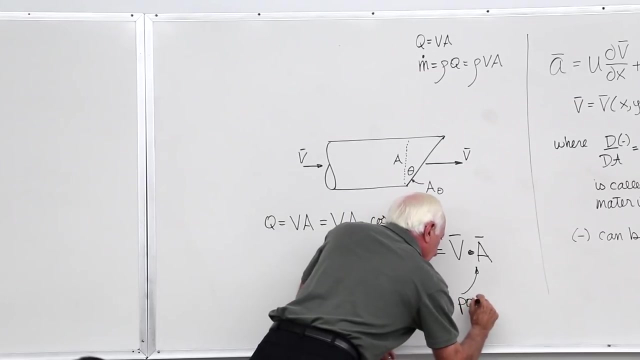 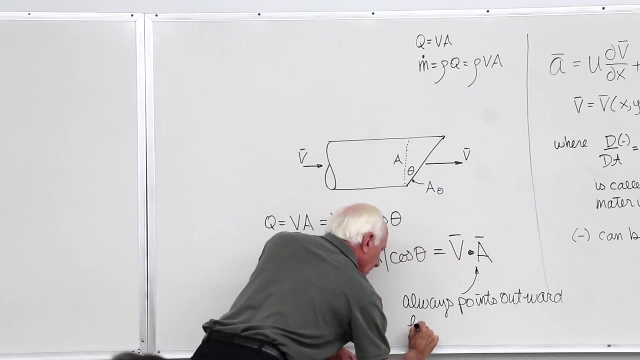 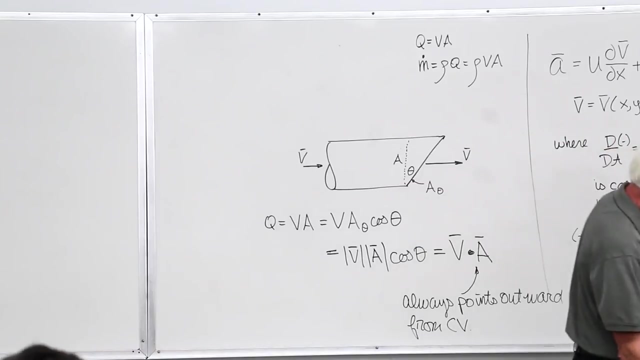 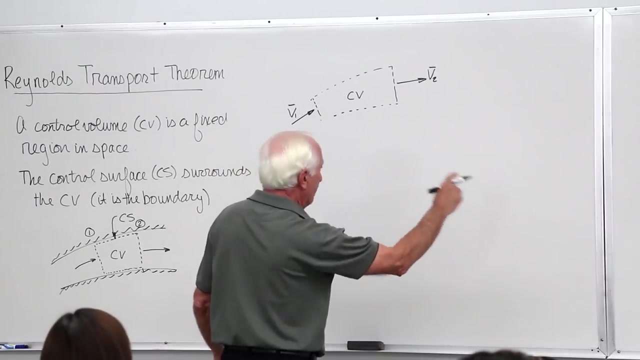 velocity vector dotted with the area vector. Just one thing, so you know This area vector always points outward from the control volume. My convention Always points outward from the control volume. Okay, we'll use that over that derivation. So if we were to find Q over here, it's equal to V dot A. 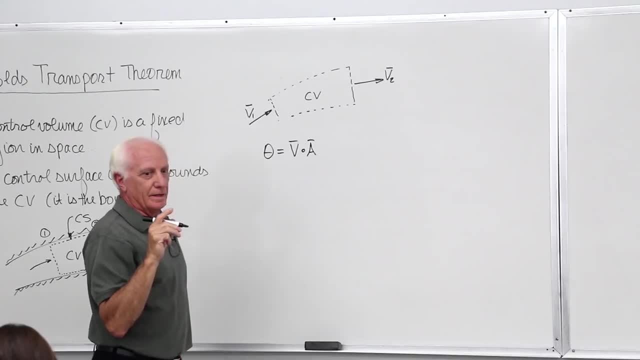 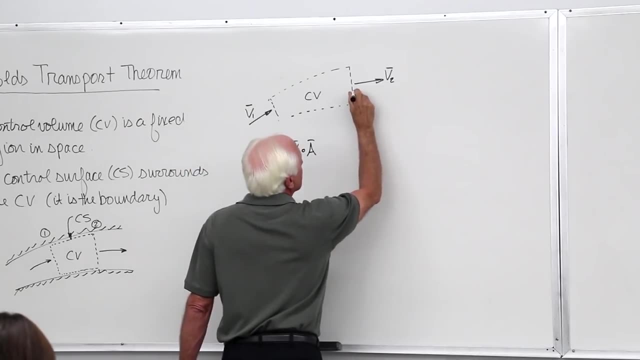 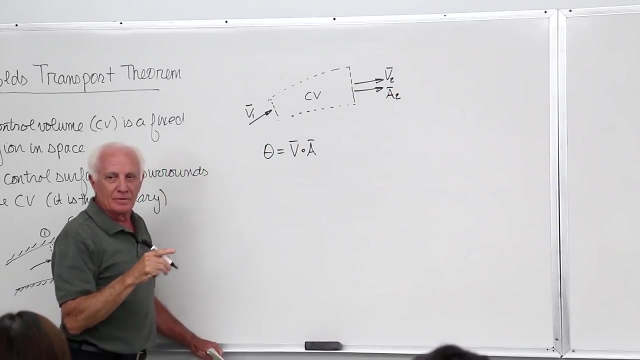 Okay, Okay, Okay, Okay, Okay, Okay, Okay, Don't forget: the area vector always points outward from the control line At 2,. the area vector points outward from the control line At 1,. the area vector points outward from the control line. 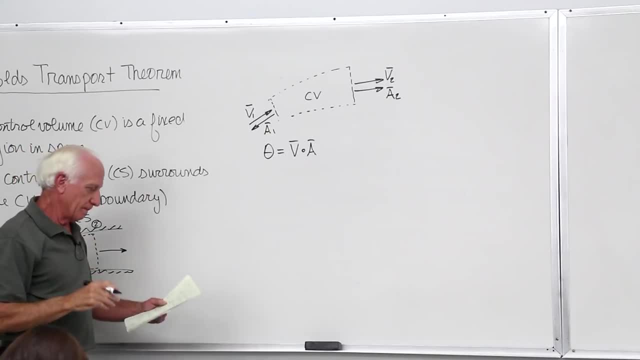 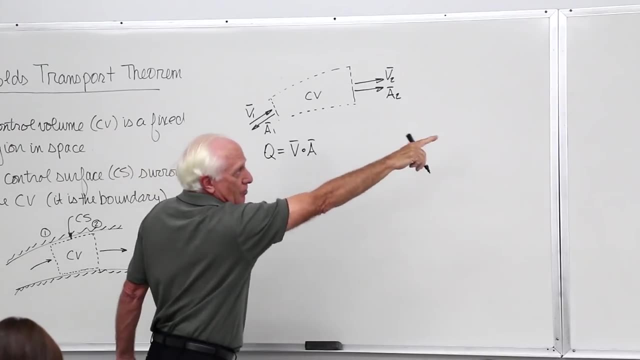 Okay, that's how you set it up that way. Now, oh, that's not, pardon me. that's cute. If you want m dot, I can put it on the board over there. m dot equals 0 times q. 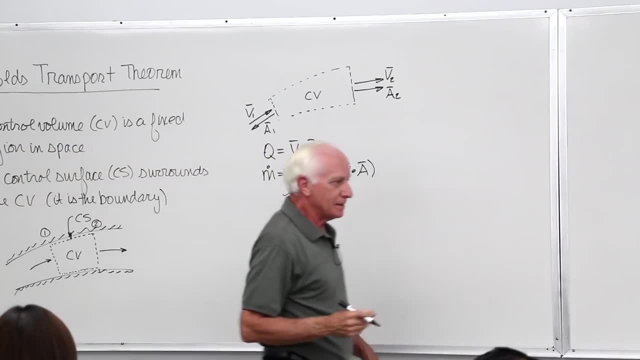 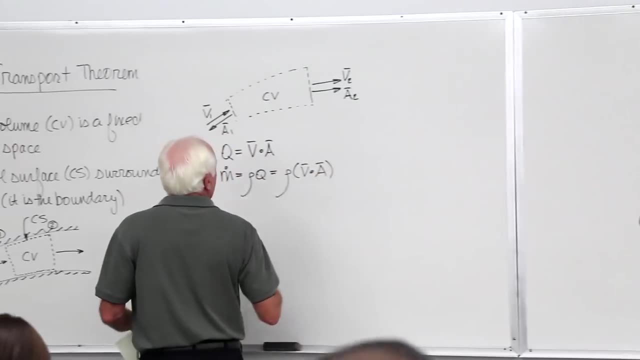 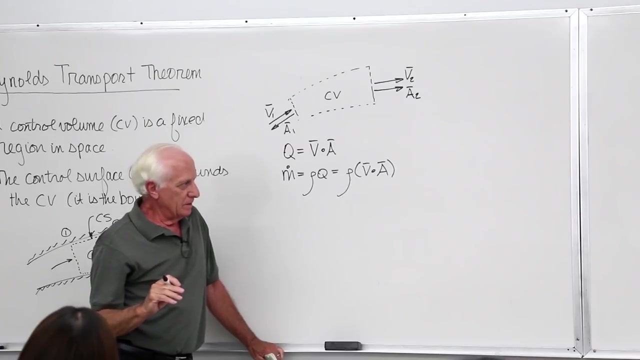 Okay, I guess I better put it down. let's see here, Okay, Those vectors. They're going to point in the same direction. The angle between them is 0 degrees. They're coincident collinear. Okay, The angle between them is 0.. 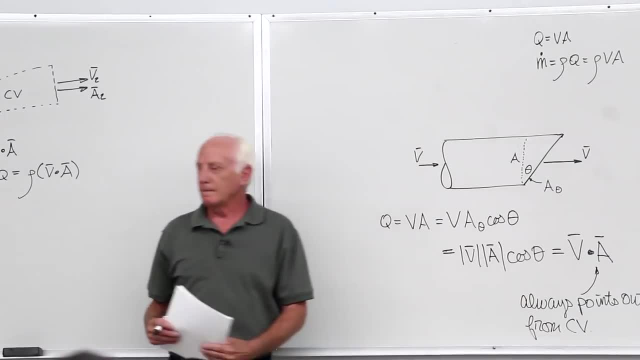 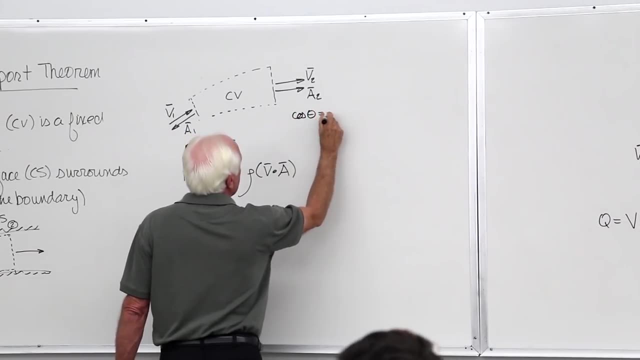 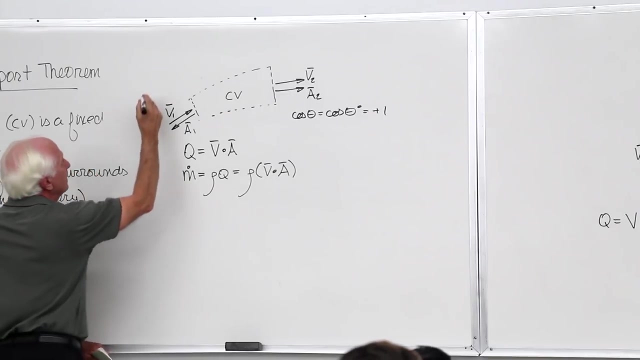 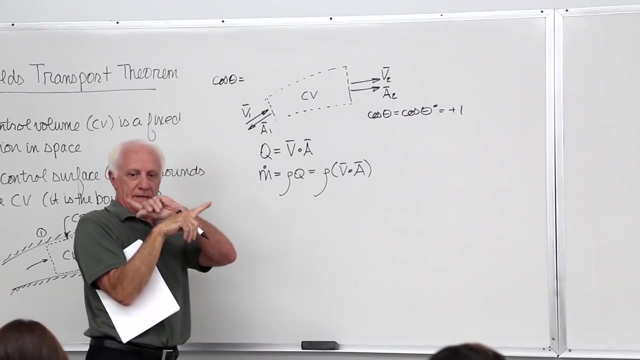 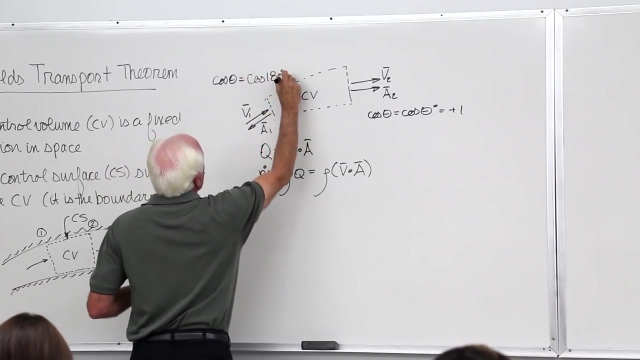 Cosine of 0 is plus 1.. So this sign: here: cosine theta equals cosine 0, equals plus 1. Over here cosine theta equals 2. vectors are pointing opposite The angle, 180.. Minus 1.. 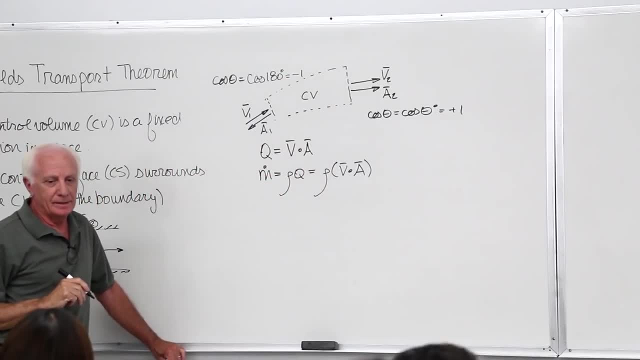 So the dot product has a sign. If the flow comes in, it's negative. If the flow goes out, it's negative. If the flow goes out, it's negative. So the dot product has a sign. If the flow comes in, it's negative. 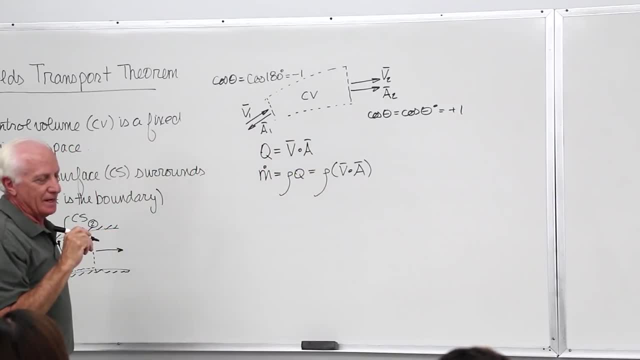 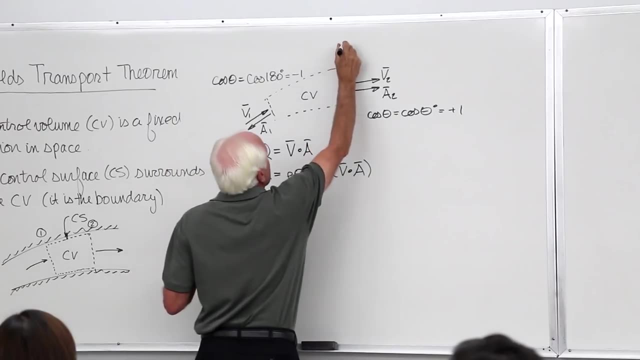 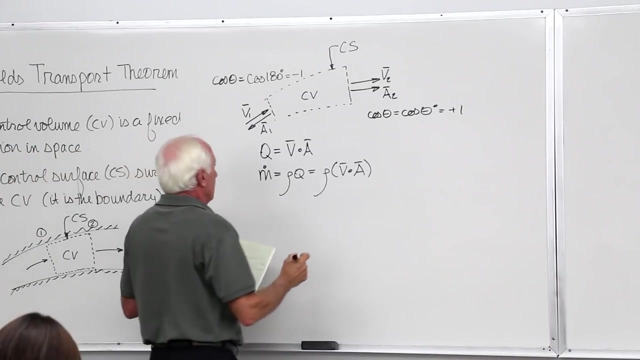 If the flow goes out, it's negative. If the flow goes out, it's positive. The area vector always points outward from the control volume. If you want to label this again, we'll be real precise now: control surface. All right. 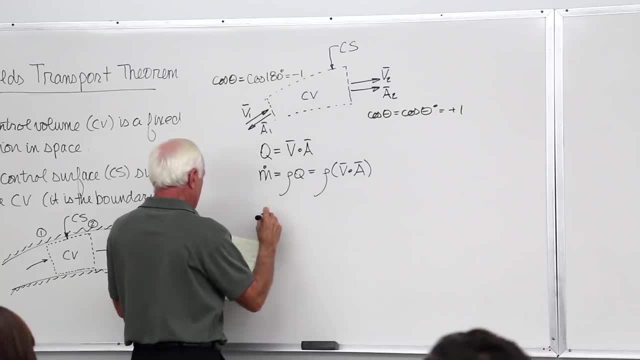 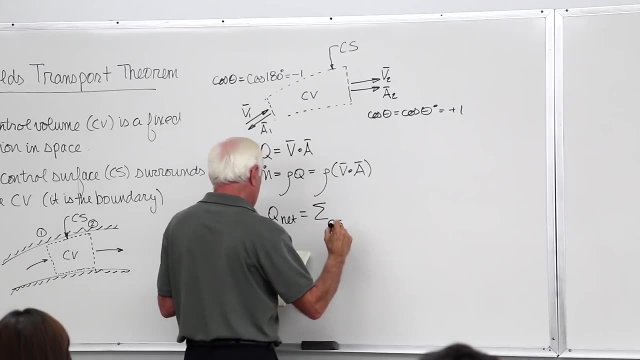 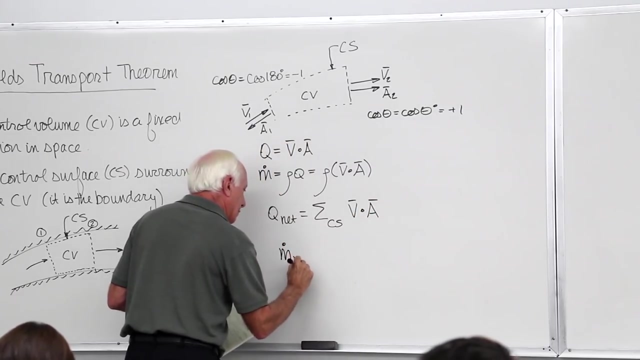 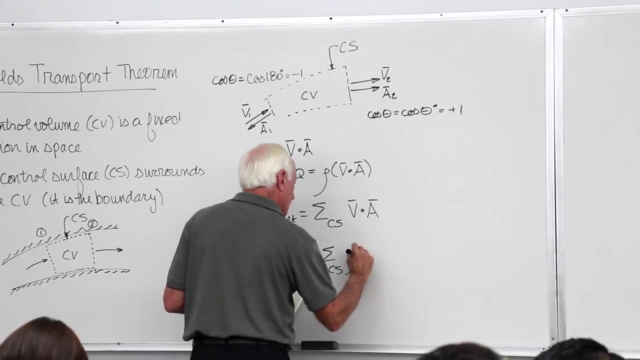 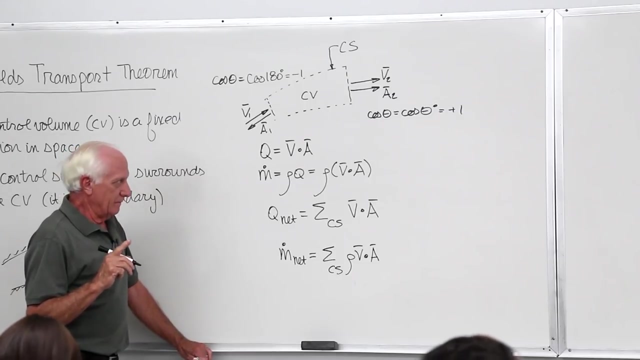 So m dot is that. And then q net equals the sum over the control surface of b dot. So m dot equals m dot Of b dot a and m dot net, equal sum over the control surface. rho v dot a. Now, don't forget, v dot a is positive if stuff goes out. 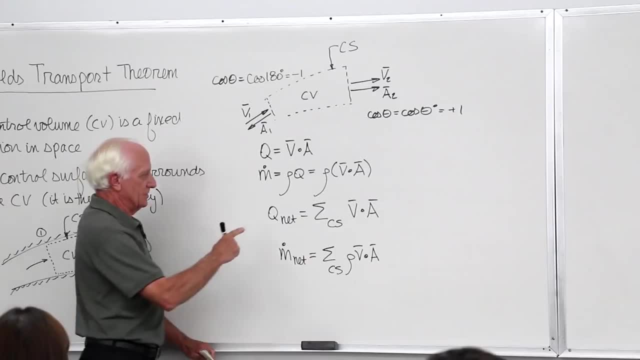 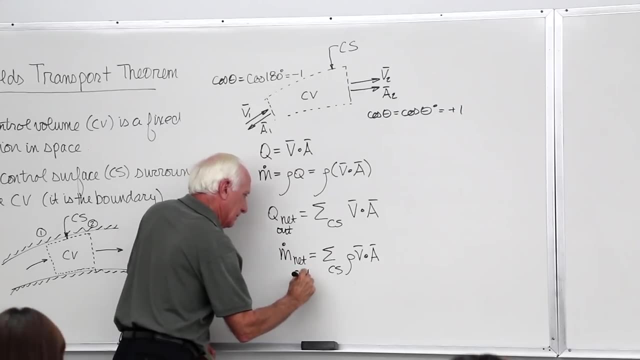 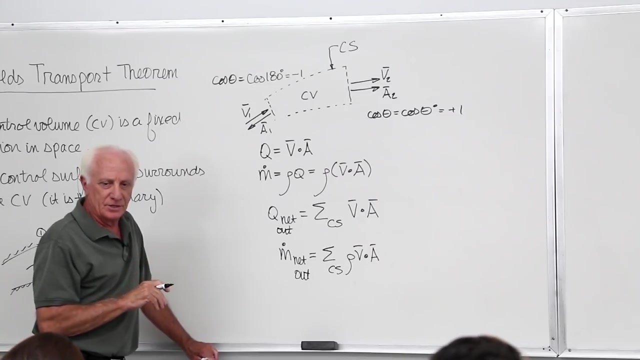 V dot a is negative if stuff comes in. So this is the net output. So this is the net out flow: m dot, net out. What does net mean? Subtract something. The word net means subtract something, The net balance in your checkbook. 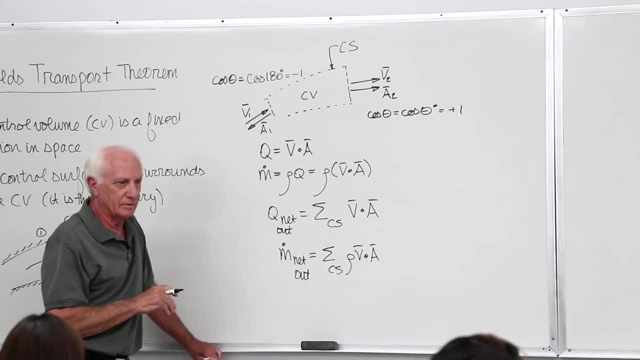 Yeah, subtract something: What came in minus what goes out. In this case it's what goes out minus what comes in. So q net out then in that case would mean the flow rate leaving minus the flow rate entering. The flow rate leaving minus the flow rate entering. 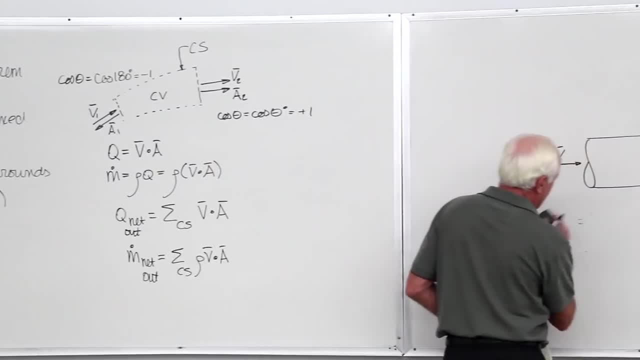 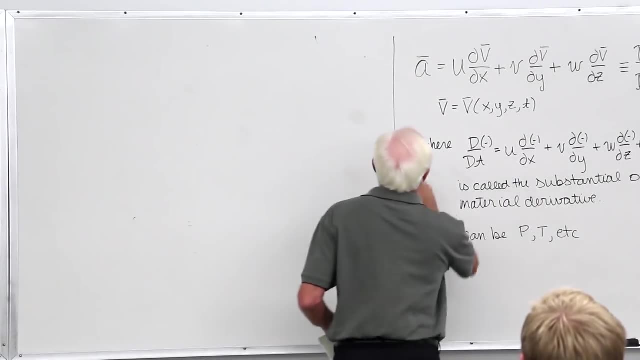 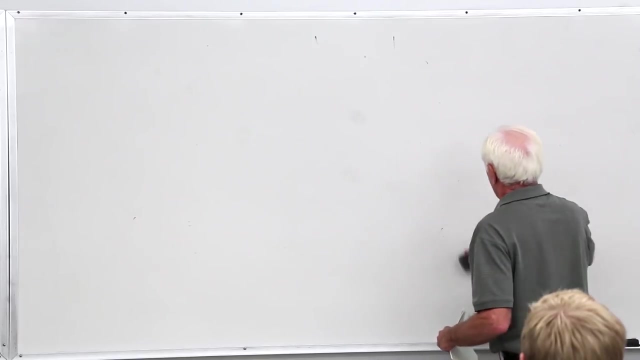 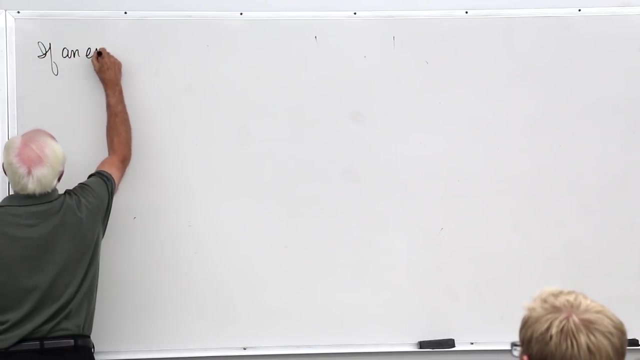 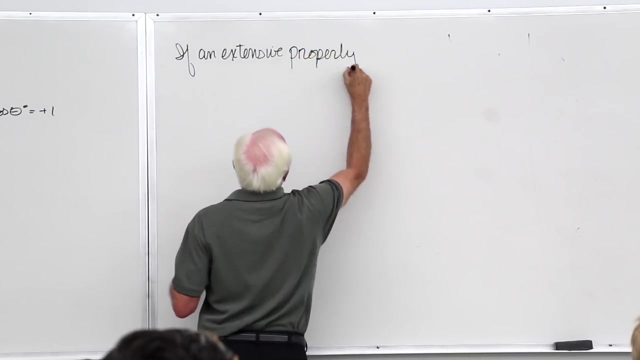 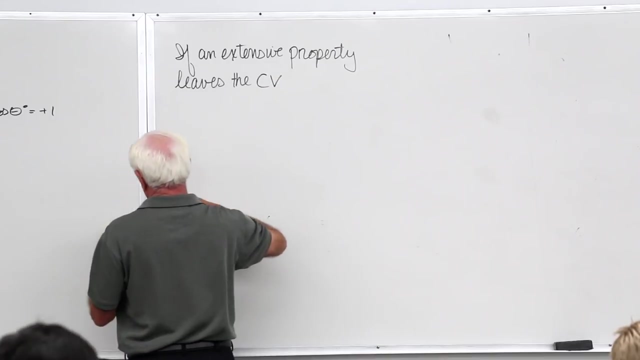 Okay So that's just some background that we'll need for that. Okay So, let's go on. Okay So, let's go on. So if a vector of a specific property leaves the control volume, the dot means with respect. 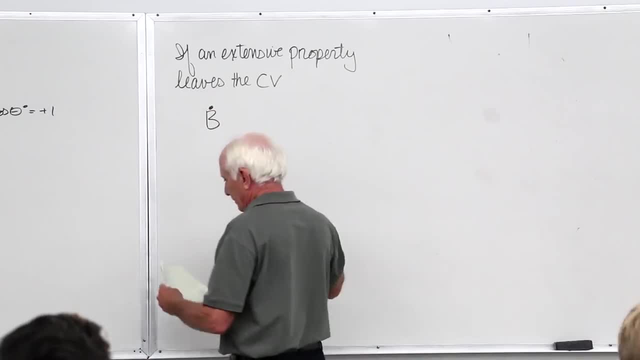 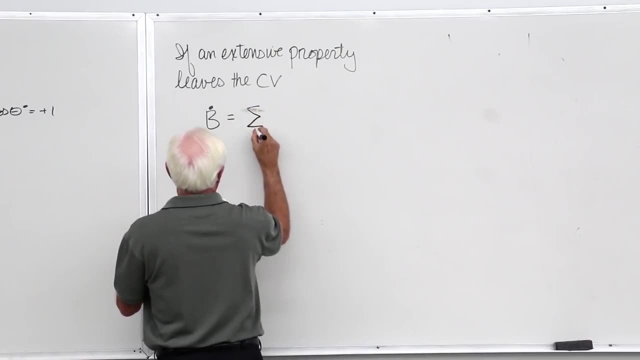 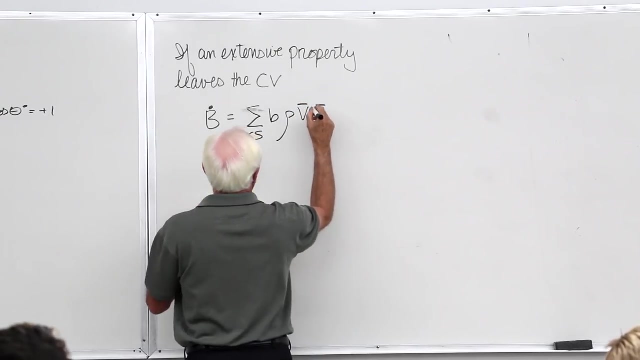 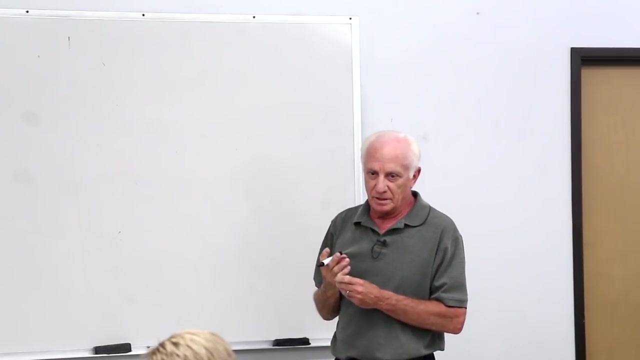 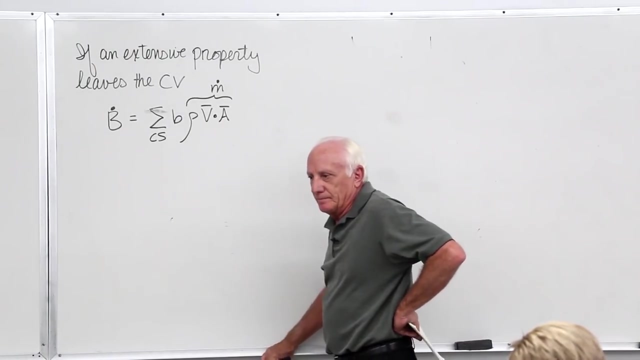 to time. The rate of change of v with respect to time. v dot Okay, Okay Okay. V can be different variables. One of the most common ones is energy. We're going to get in about two days energy, So maybe capital B means energy, Little b is. 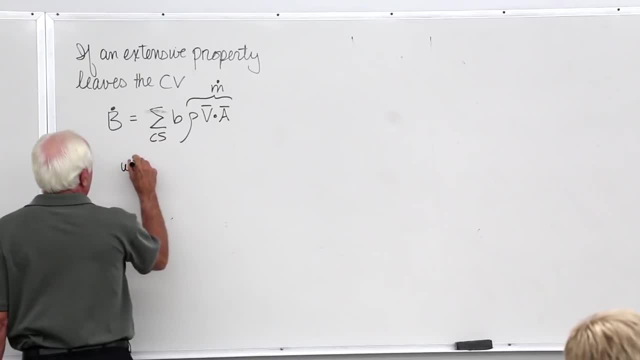 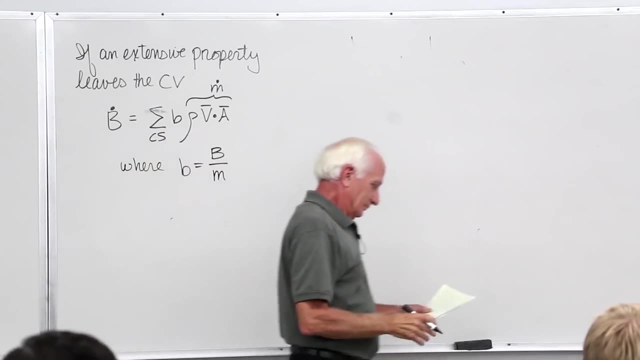 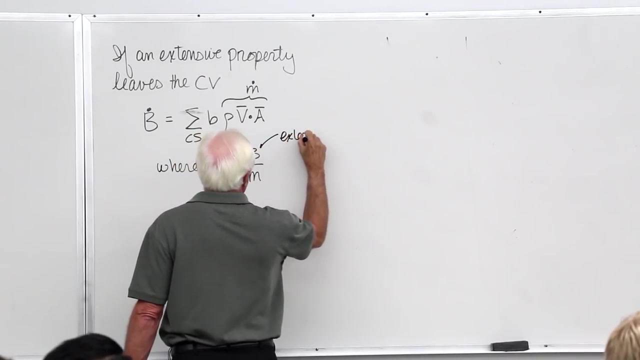 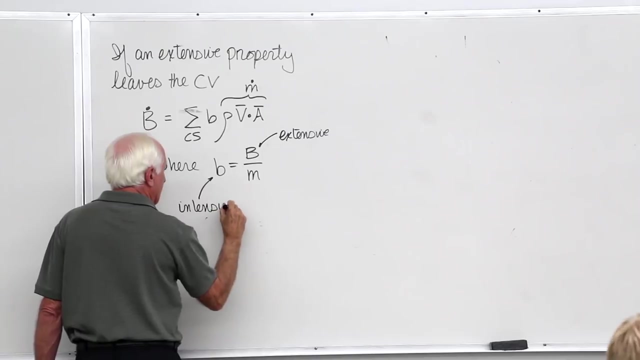 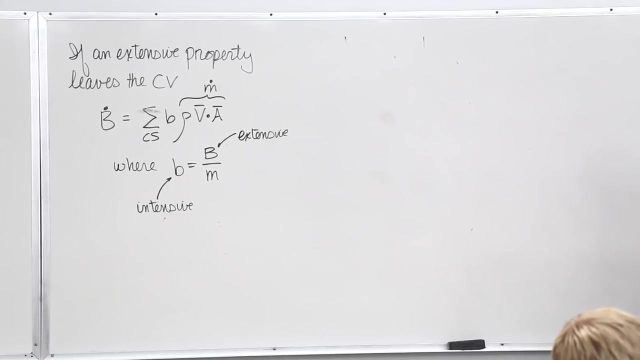 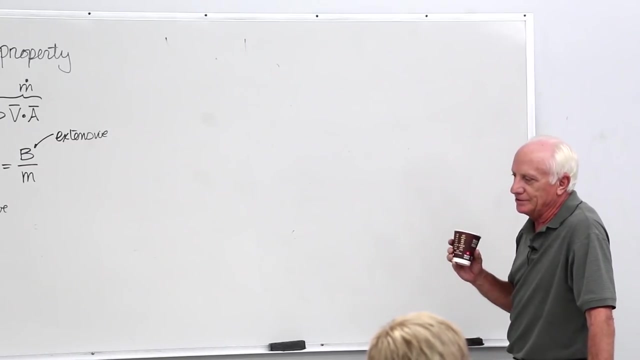 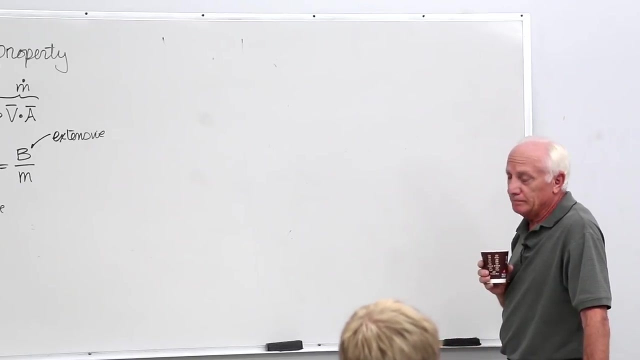 big B divided by mass. Capital B is extensive, Little b is intensive. So let's, just for the sake of giving some kind of name, let's say capital B is energy in SI joules. Little b is in joules per kilogram. 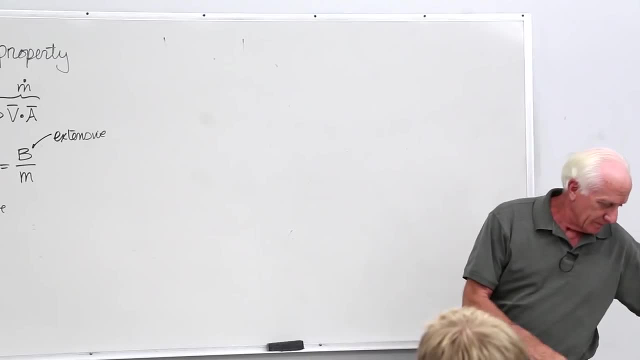 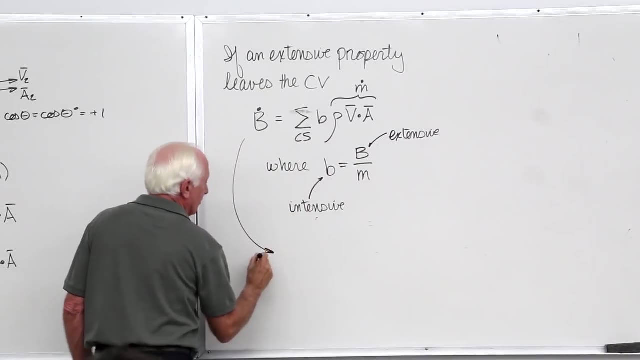 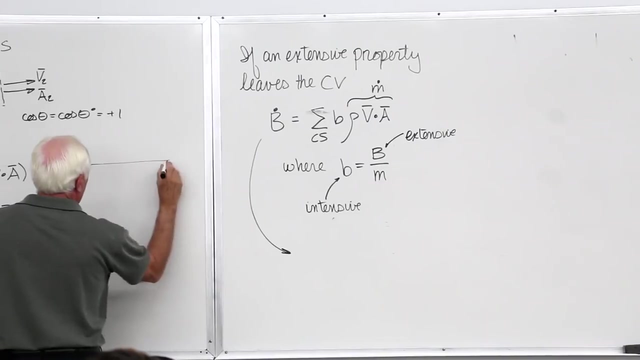 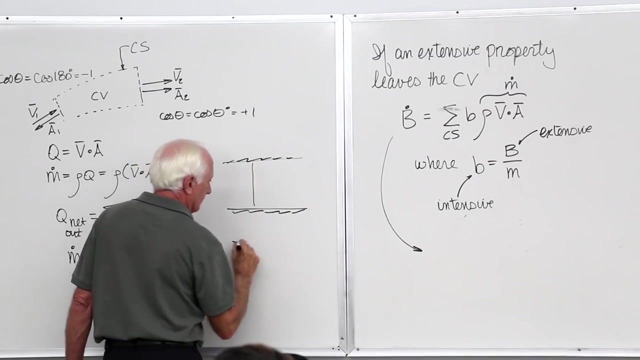 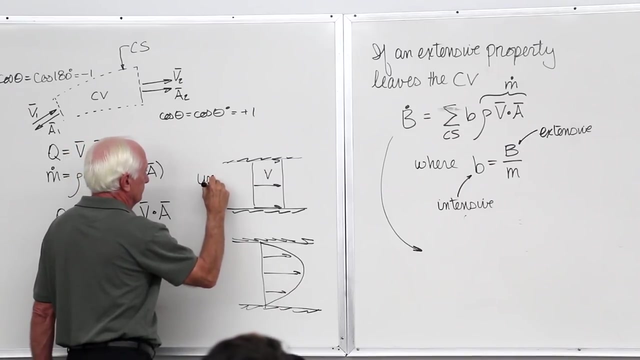 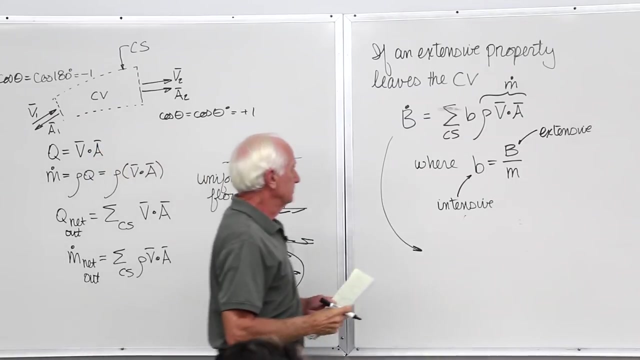 So that's what we mean by that. And if you want to be real official, and if it's not a uniform flow across the inlet and outlet, if it's not uniform flow, okay, that's uniform flow, That's not uniform flow, Not uniform flow, You can. 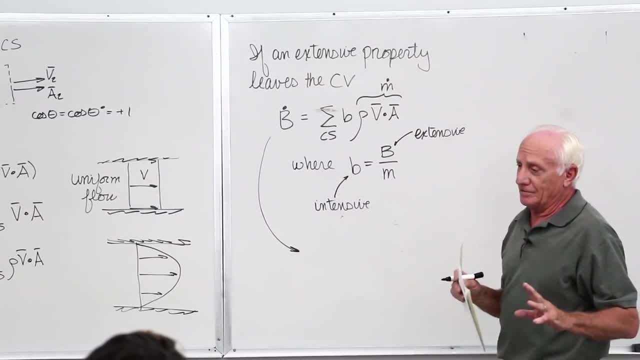 use a summation. If the velocity profile is varying across the flow area, you can use a summation. If the velocity profile is varying across the flow area, you can use a summation. If the velocity profile is varying across the flow area, you can. 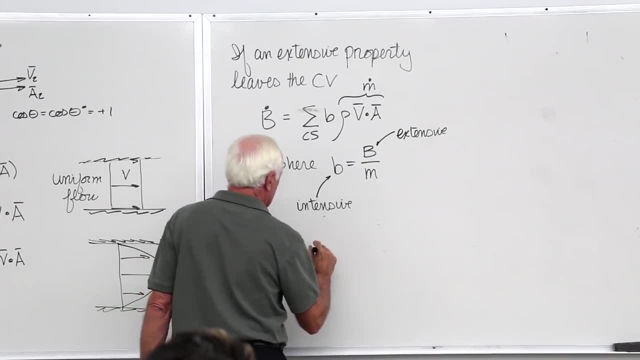 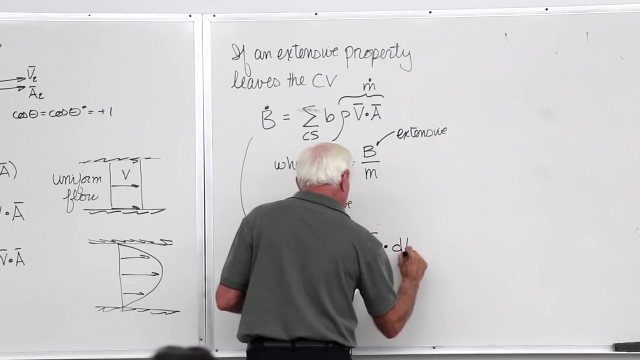 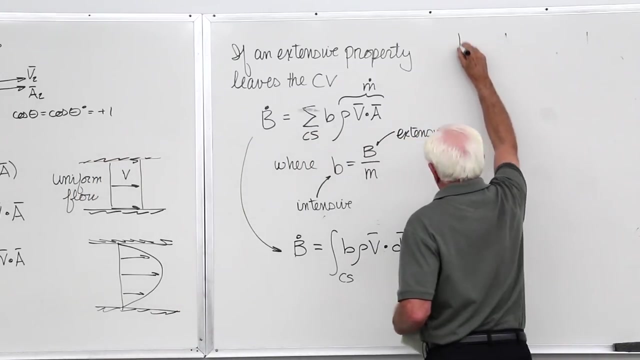 use a summation, But then you have to be more official and use the integral definition, Because then B is going to depend on A, DA. Okay, so two possible forms of it, One for uniform flow, One for nonuniform flow, And we pretty much. 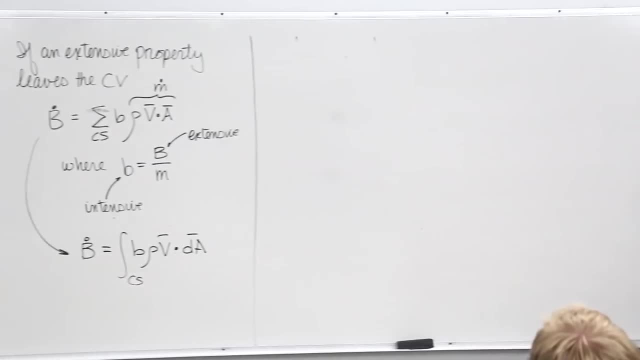 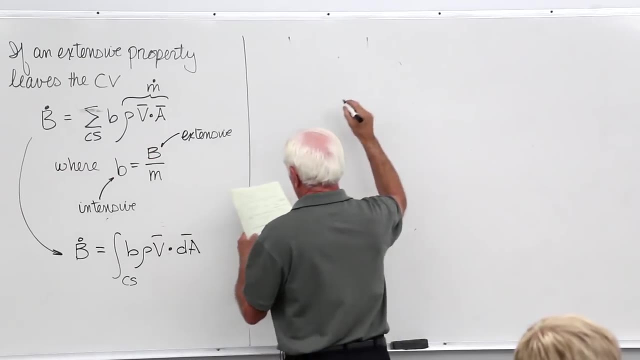 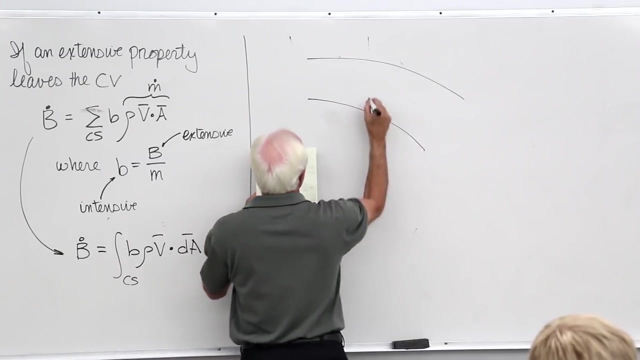 deal with uniform flow. uniform flow for a while, So it's going to be uniform flow that we're looking at. All right, let's draw our picture one more time. I'll change it a little bit. It won't pass it away. I'll draw the solid line now. 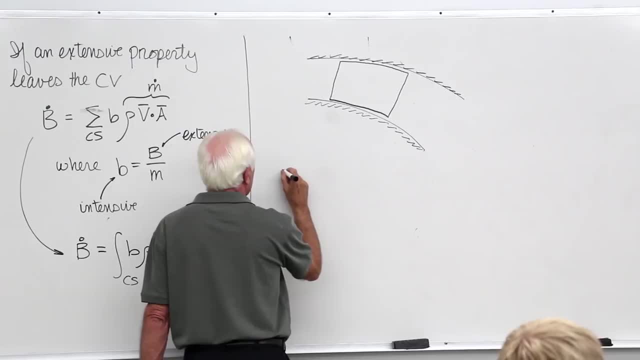 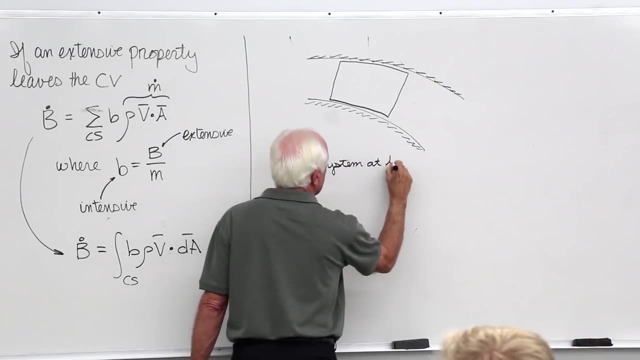 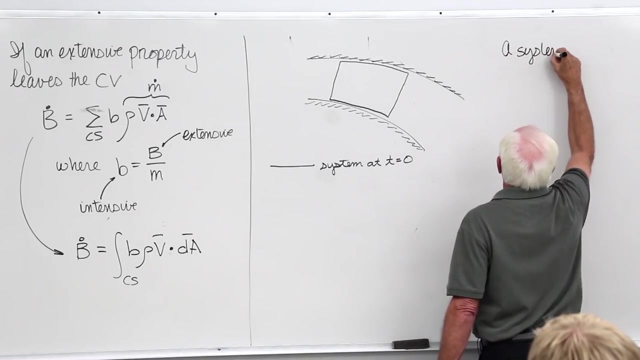 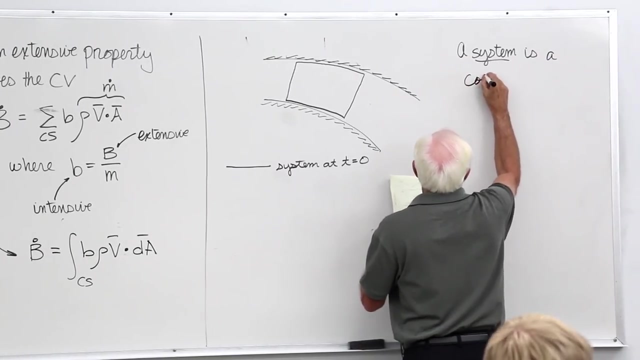 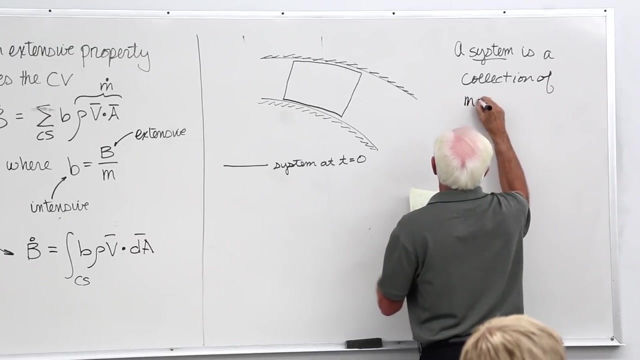 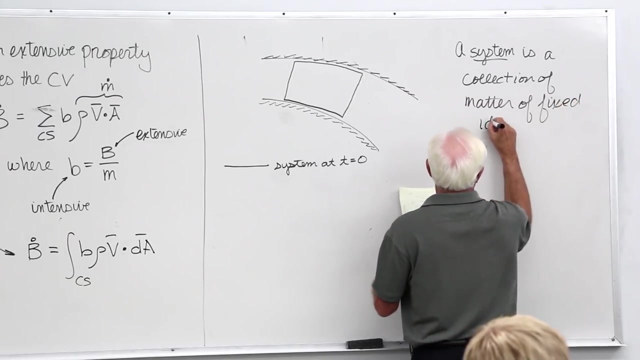 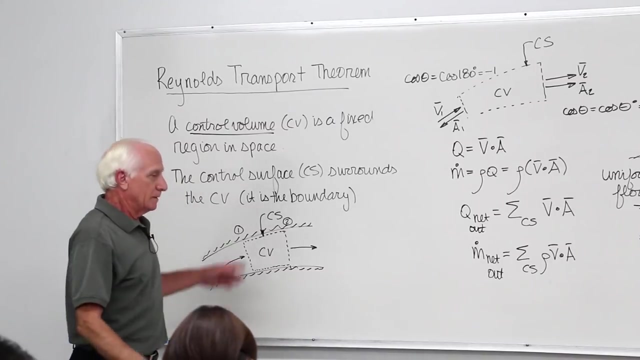 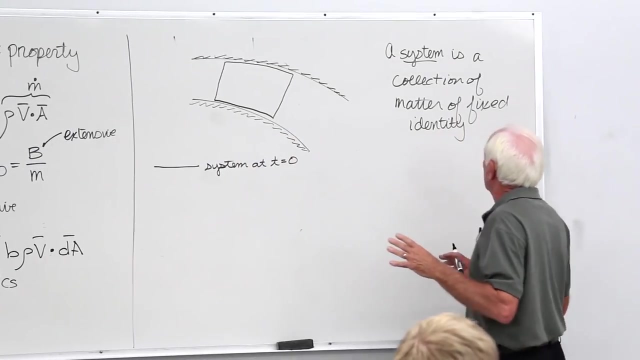 What's inside the solid line? Solid line is system. at time t equals zero, That's a system. This is a control volume. Control volume: a fixed region of space, A system, a collection of matter, a bunch of molecules, A fixed identity. 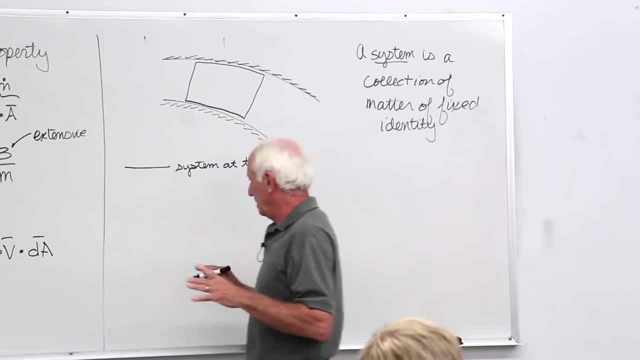 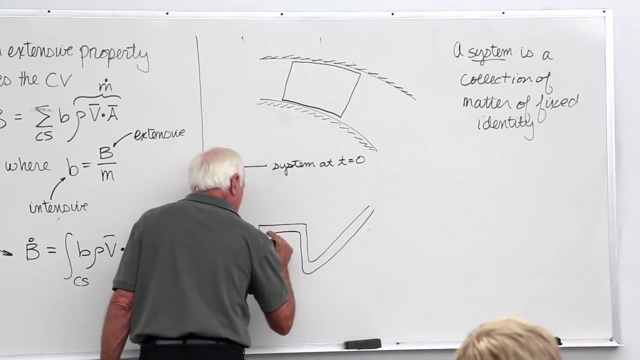 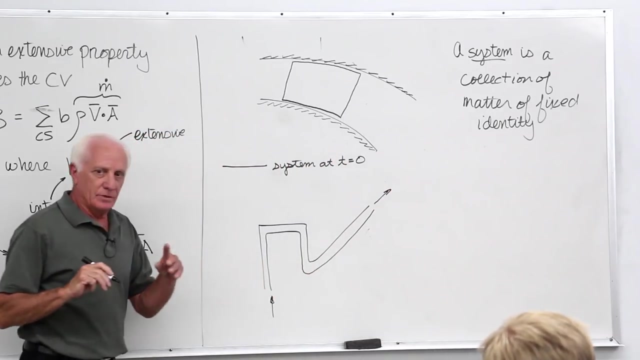 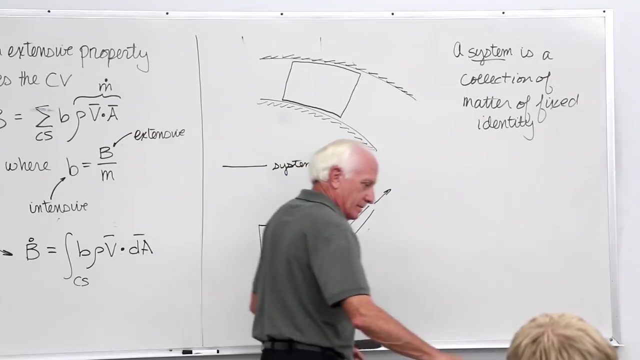 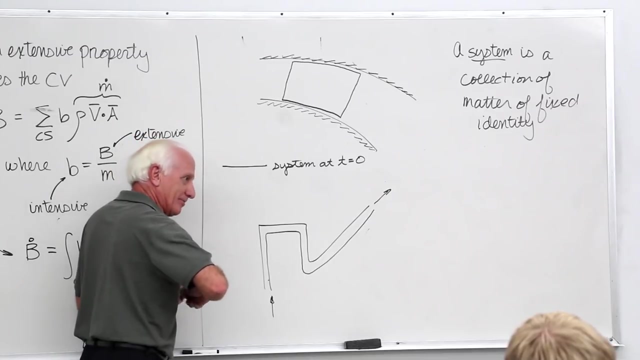 So if I had a pipe system like this, where the flow comes in here and the flow goes out up here somewhere, If I want to do a system, I'll say, okay, I'm going to take these particles and I'm going to spray paint them- maybe, I don't know- cream. 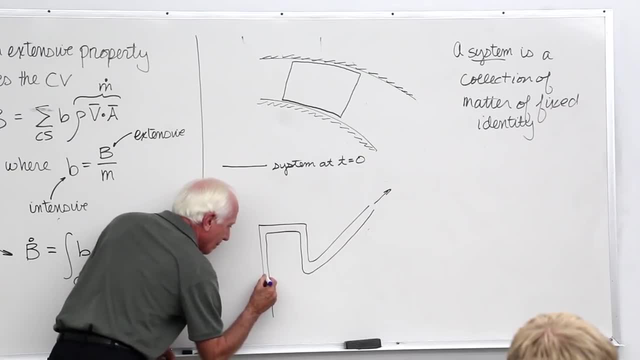 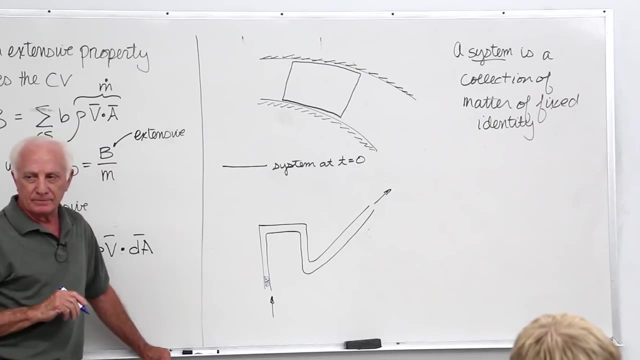 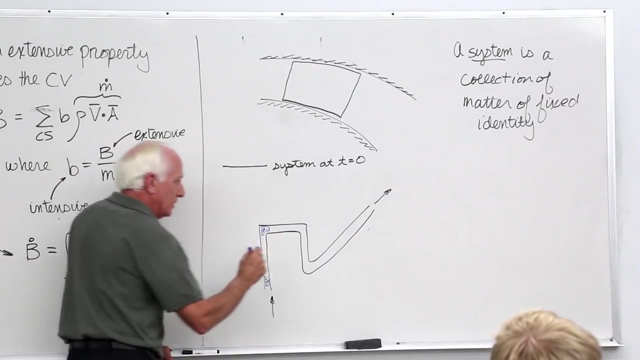 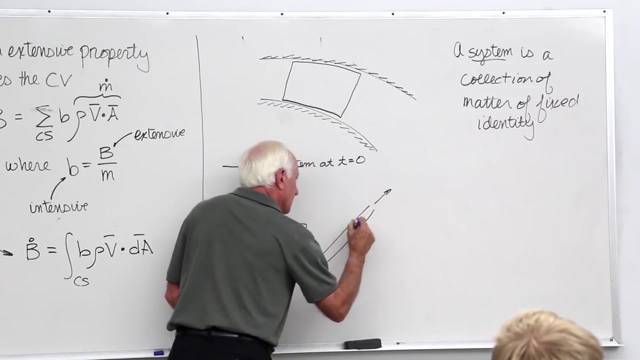 There we go. So here is a system. at time, t equals zero. This is water and pipeline. Wait 15 seconds. It's up there now. Wait 30 seconds. It's down here now. Wait a minute and a half. It's up here now. 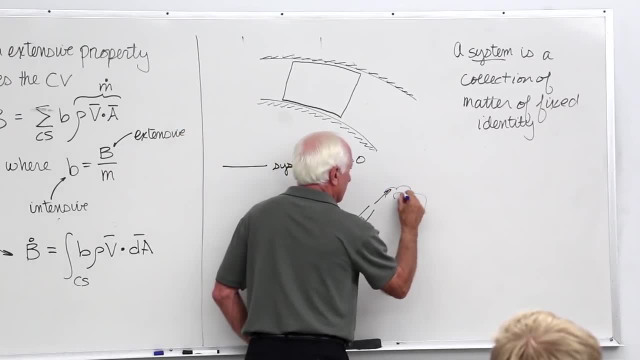 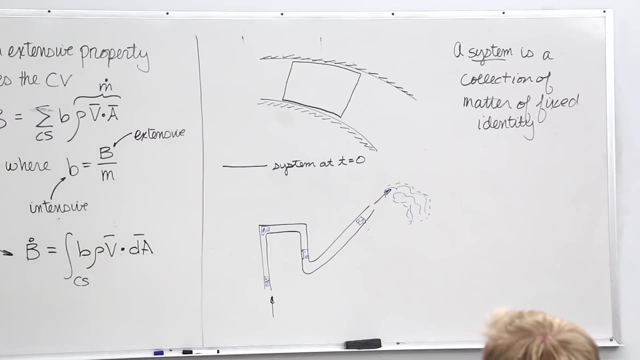 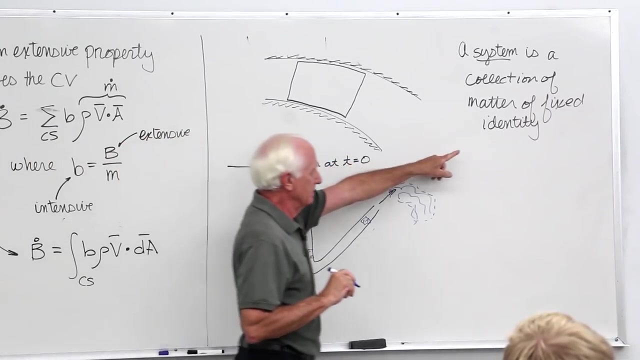 Wait a minute and three quarters It comes out of here. There it is. Identify: Every particle has a number and a name: Particle A1,, B2, C10.. Everyone's tag name: Fixed identity. We don't do that generally in engineering. 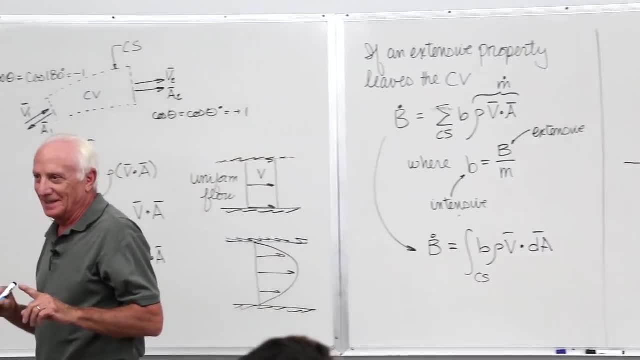 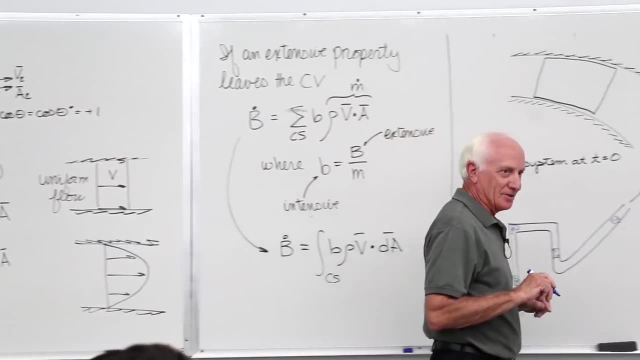 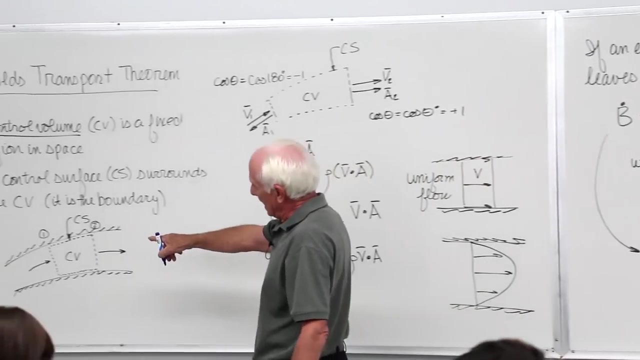 If I'm analyzing my hot water heater in my garage, I'm not going to watch the water molecule come from the city water supply, go in that water heater, get heated and end up going out the faucet in the kitchen. No, I'm going to draw a system boundary around that hot water heater and I'm going to analyze. 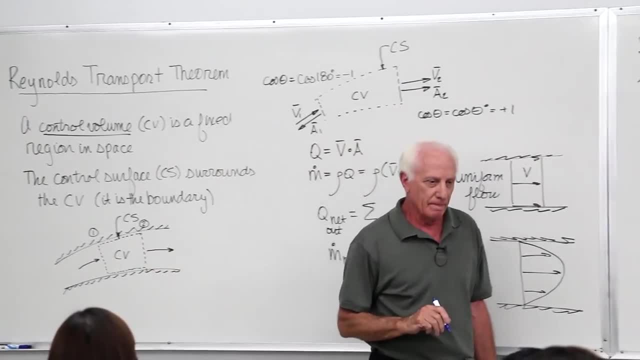 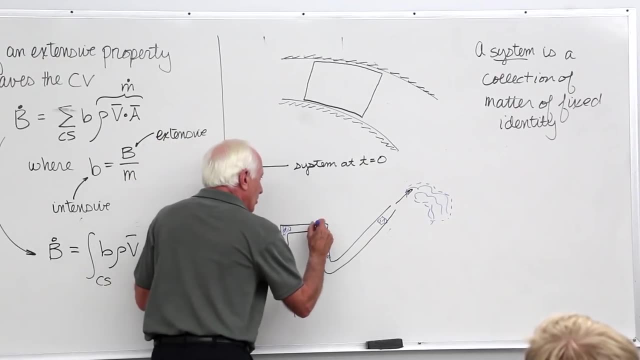 what comes in cold water and what goes out hot water. Now, over here, if I want to draw a control line, I might say I'm going to look at this pipe fitting. It's called an elbow, a 90 degree elbow. 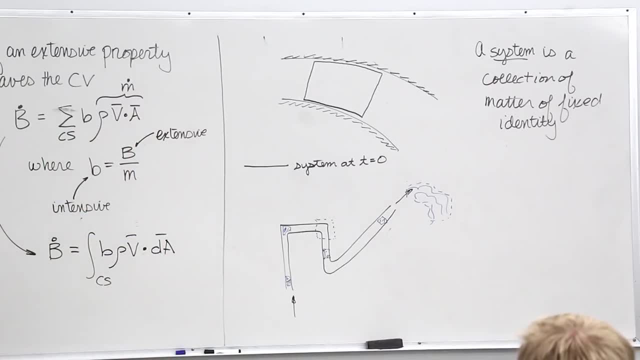 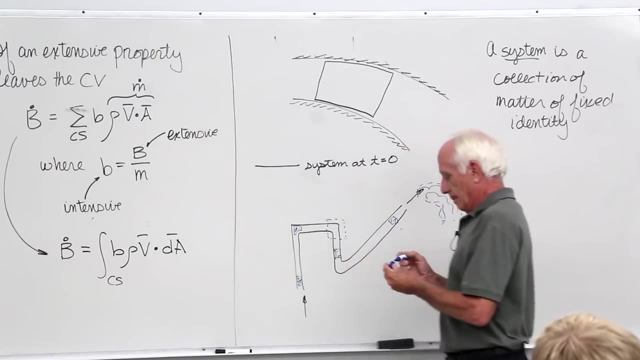 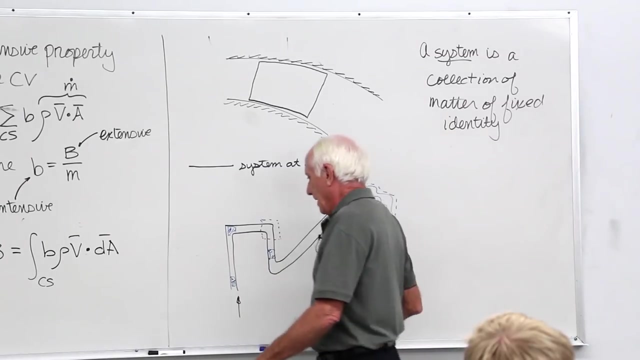 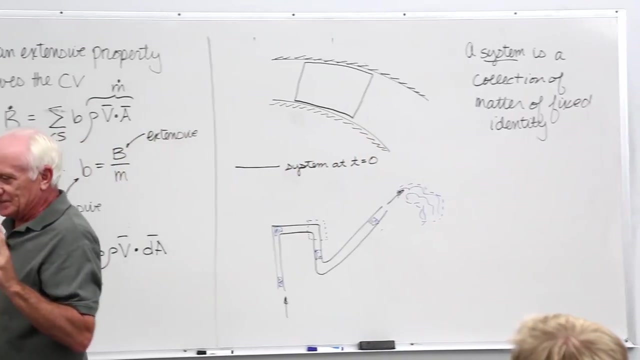 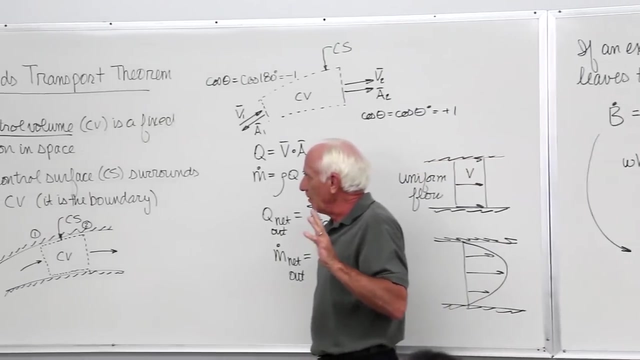 I'm going to analyze that 90 degree elbow. That now becomes a control line. Okay, Back to here again. That's like this. I'm going to follow those particles, But the Reynolds transport theorem is a missing link. type equation: Most of the laws in science, physics and so on are written for a system. 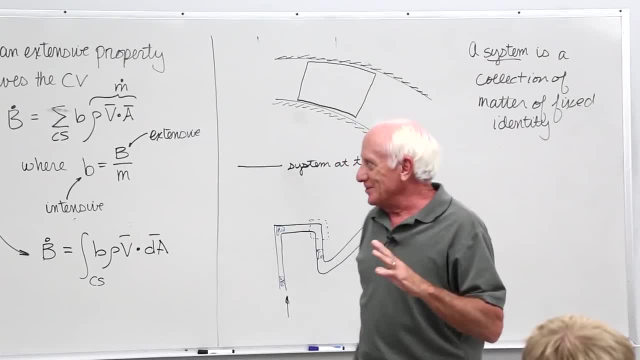 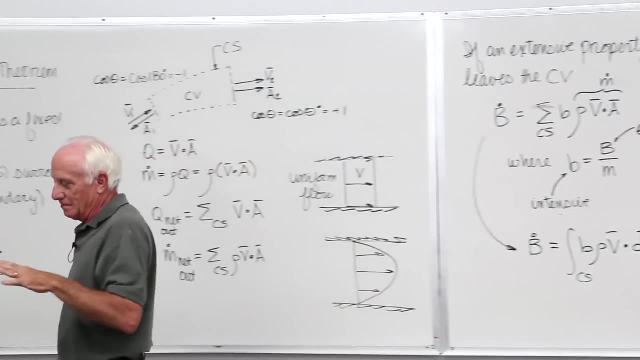 Okay, In engineering, though, we do a lot of control line studies, So this theorem allows us to take basic laws written for a system and convert them to one more useful to us, the engineers, which are in control line form. Okay, 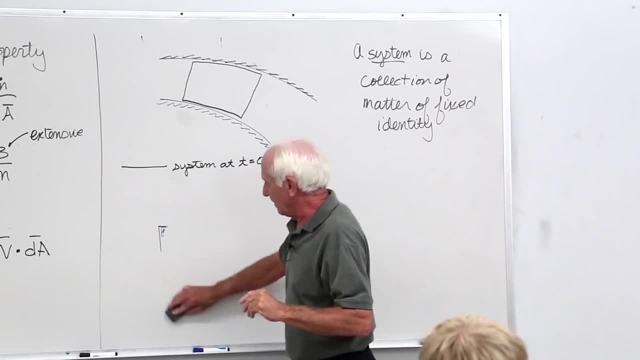 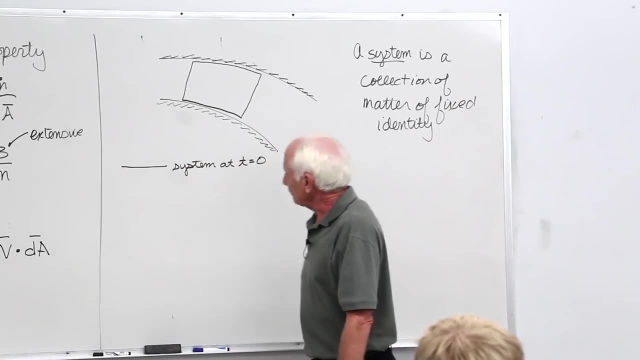 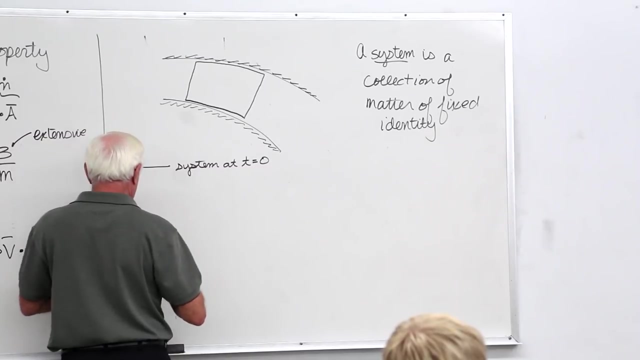 So what I'm going to do now is I'm going to try and relate the control line to the system. All right, I'm going to call that same volume at time, zero, my control volume. Okay, So here's my control volume. 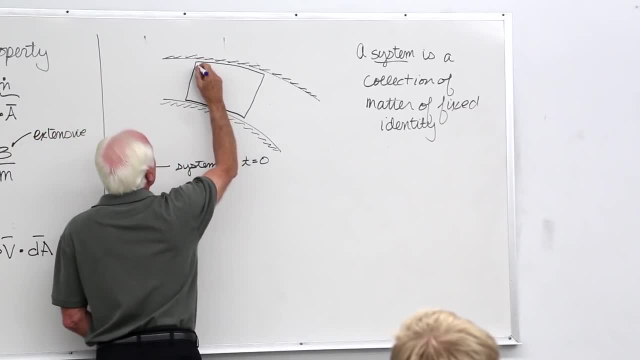 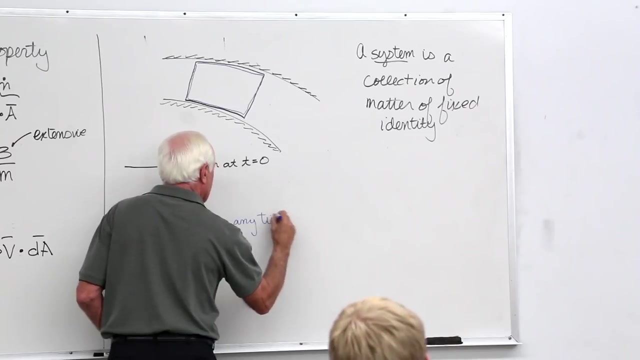 Okay, That is also going to be my control volume. This is the control volume for any time. Remember what it said: control volume Fixed in space, Not moving in space Fixed. So that's the control volume. I choose to make a coincidence at time: zero. 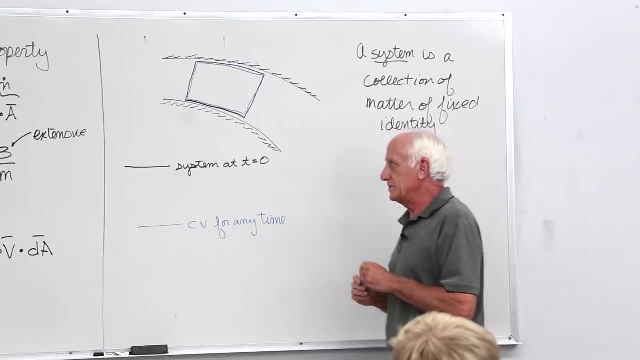 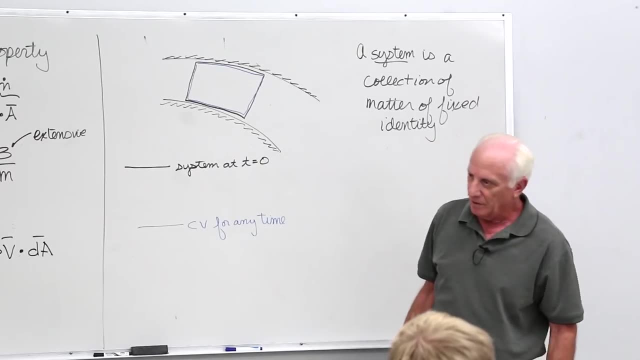 Okay, Wait 30 seconds. Does the control volume move? No, Say it again, It's in space. Does the system move? Yeah, I just showed you. Now the system moves to a new location Down that way, Because the velocity is here. 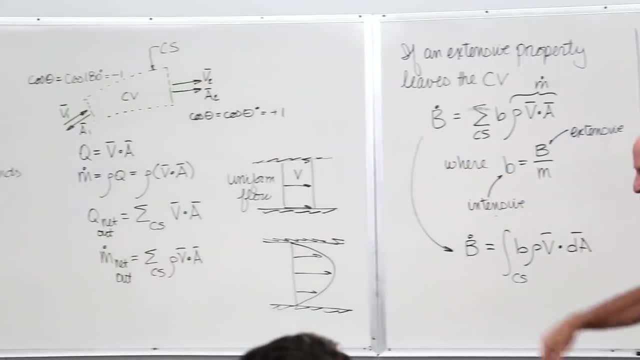 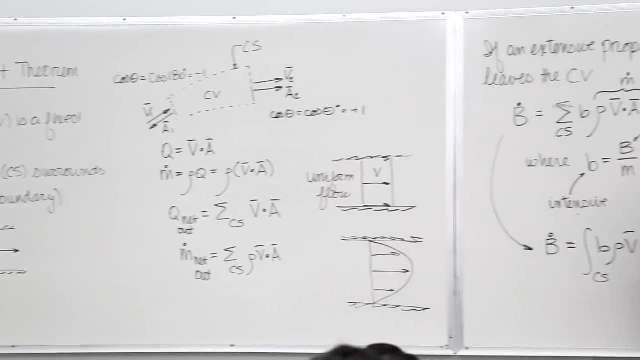 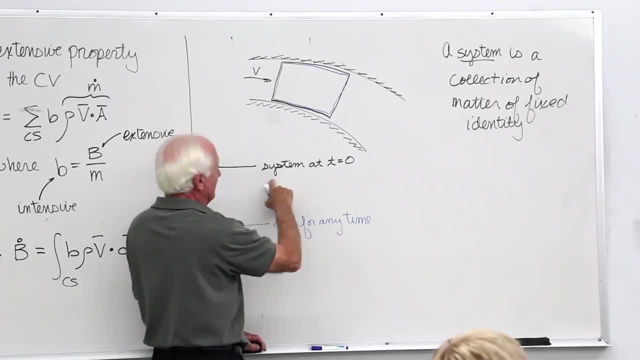 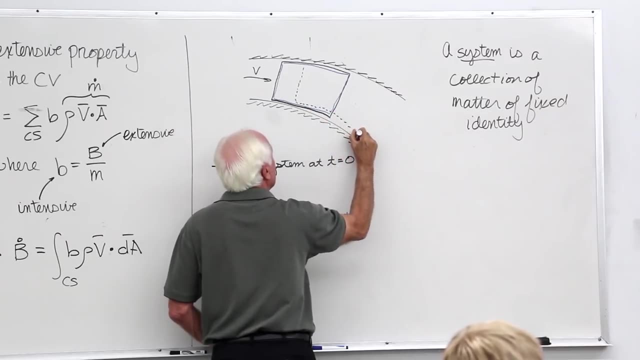 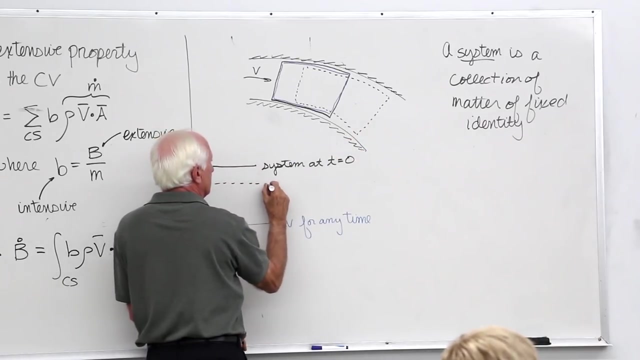 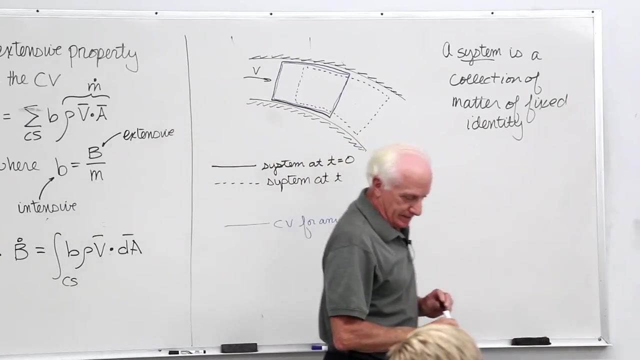 It's moving. It's moving. Okay, Now, where is it now? Okay, That was a solid line. Now it's going to be a dash line. Dash line system at time t. I think I'll call that one just Dt. 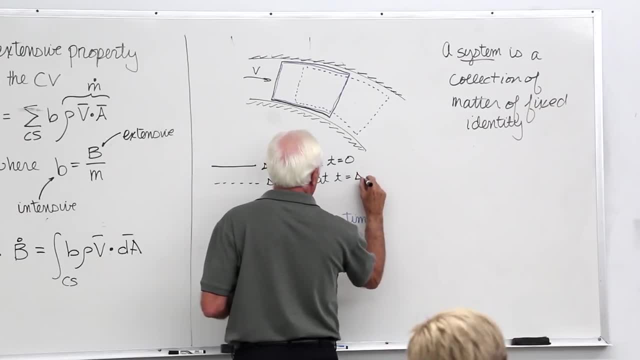 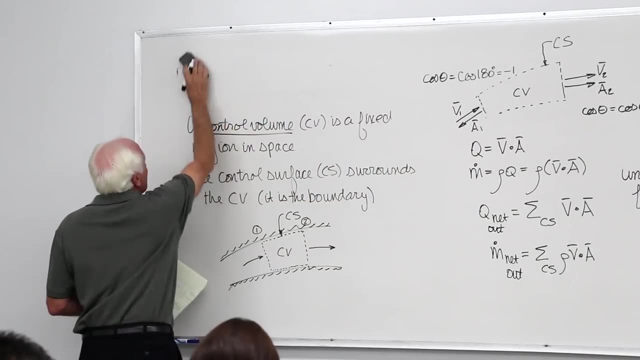 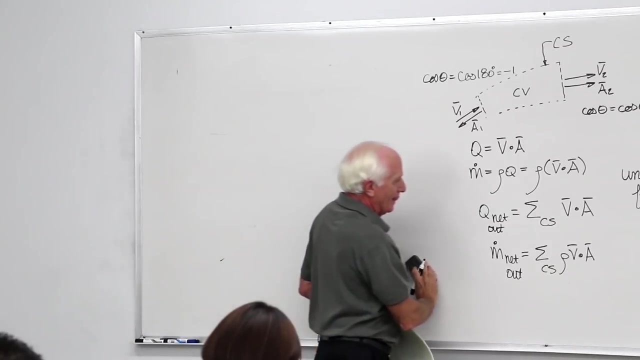 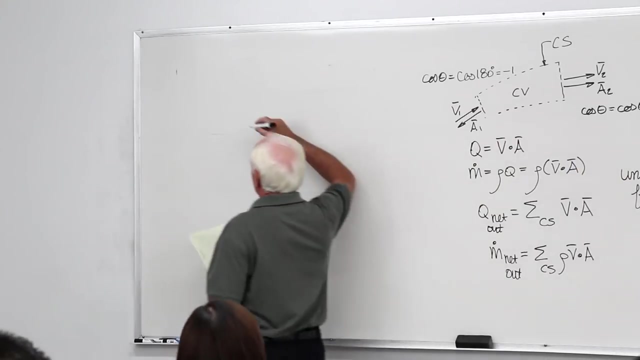 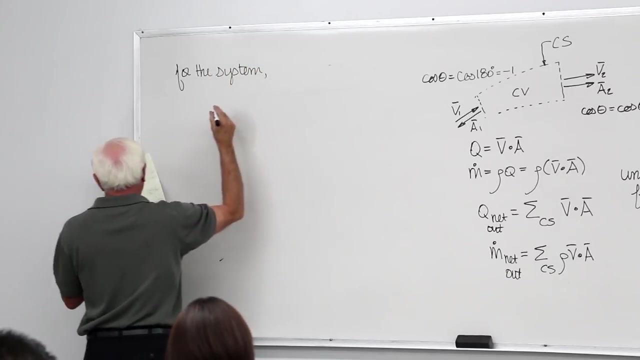 Yeah, delta t. Okay, I'm going to go way back over here. Alright, next step for the system: D, B, D, T. in the system, The amount of B. how does the amount of B change with respect to time in the system? 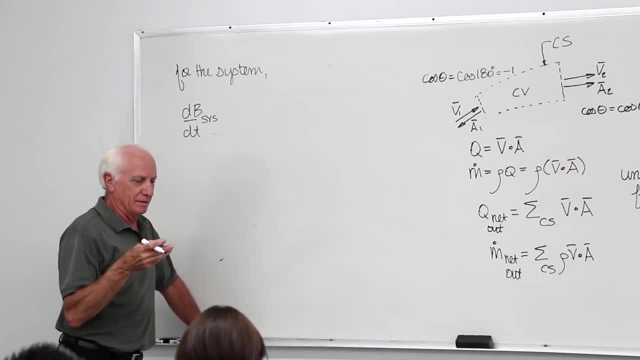 Don't forget. if you get confused, just say to yourself: energy, Okay, energy. If you watch a cubic inch of water come into your cold water pipe and hot water heater and you watch it go through the hot water heater, it's going to change the energy. 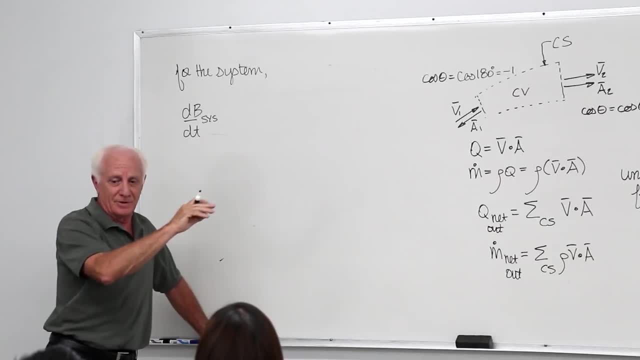 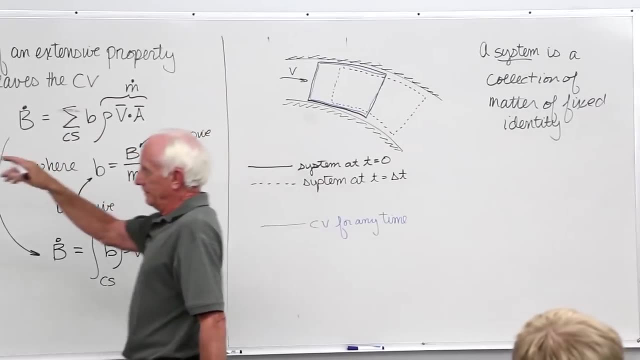 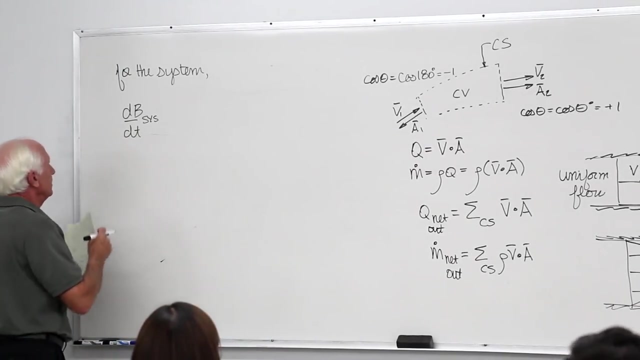 Oh yeah, Why? Because you're adding heat from the natural gas burner. Yeah, as it moves through the hot water heater, it's going to change its energy. Well, B is like energy. B can be various properties: energy, momentum, mass. 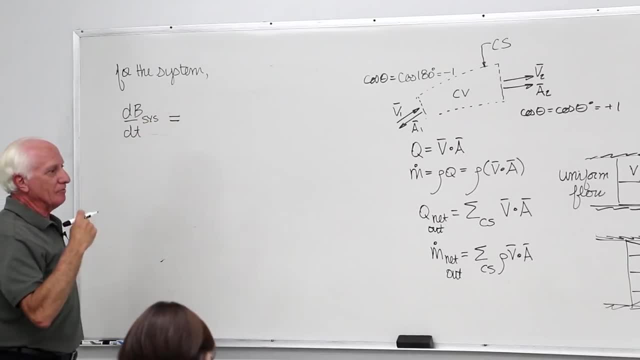 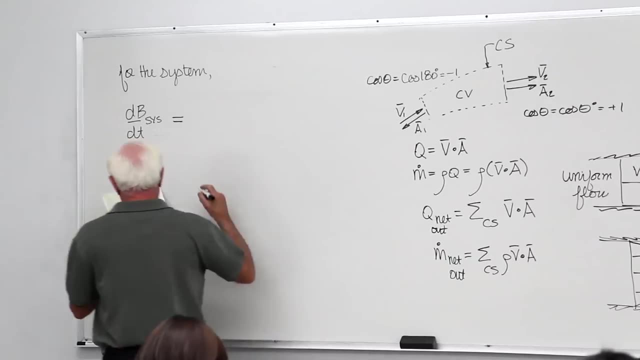 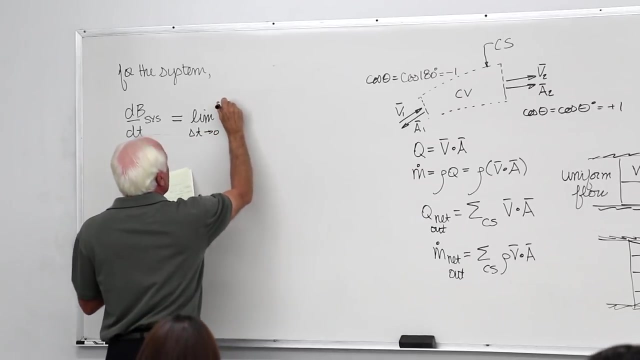 So this is the time rate of change of the amount of B in the system. Start off basic definition. What is a derivative Limit? as delta T approaches zero, Of the amount of B in there at time? T plus delta T minus the amount of B in there at time T equals zero. 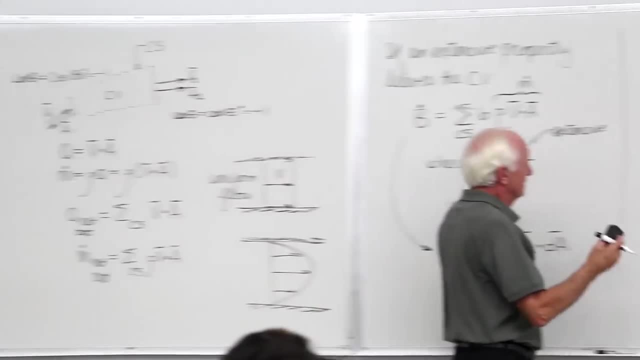 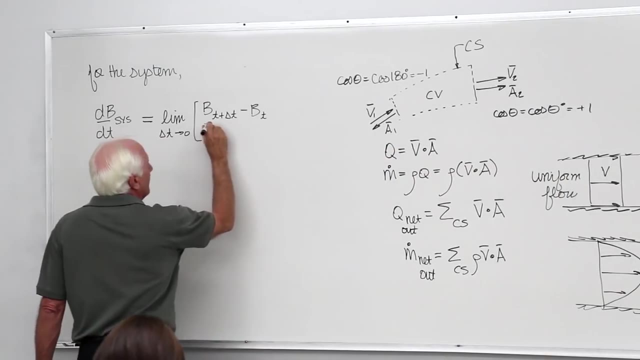 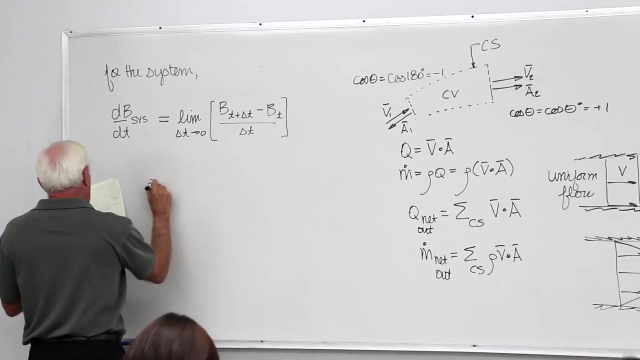 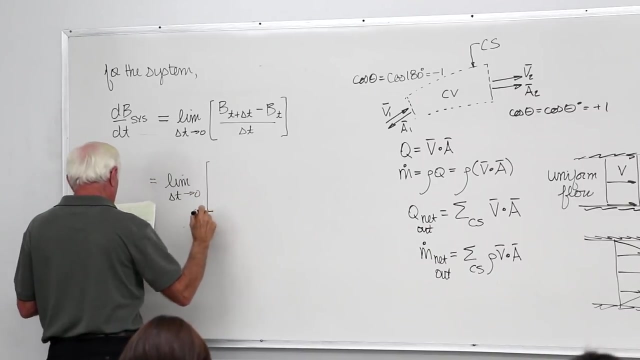 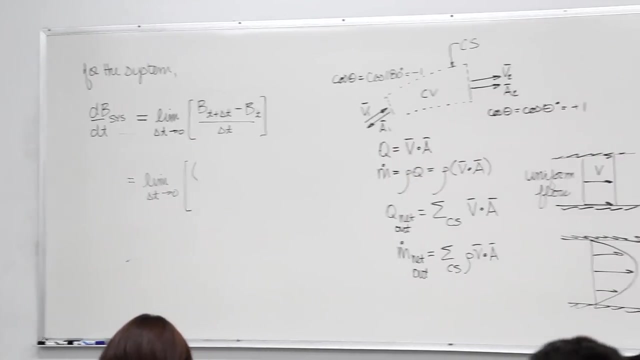 T equals T. We won't call that zero, We won't use a zero, Just call it time T Divided by what was the time change, Delta T Equals, Okay, The amount of B in there at time T plus delta T. 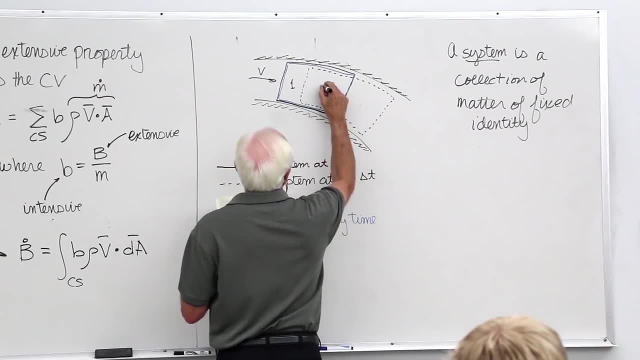 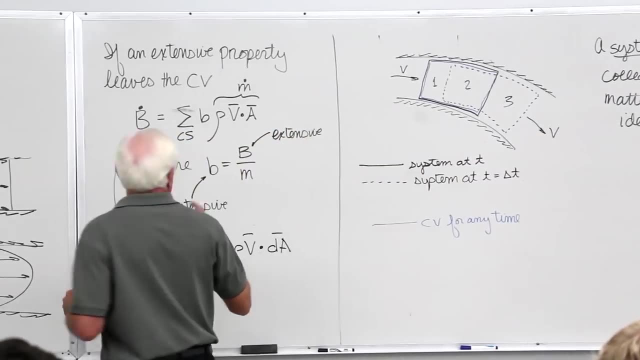 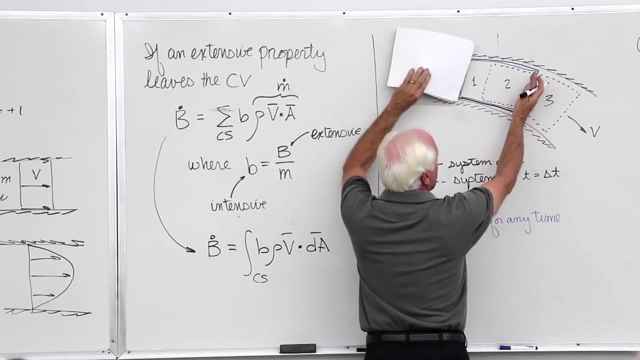 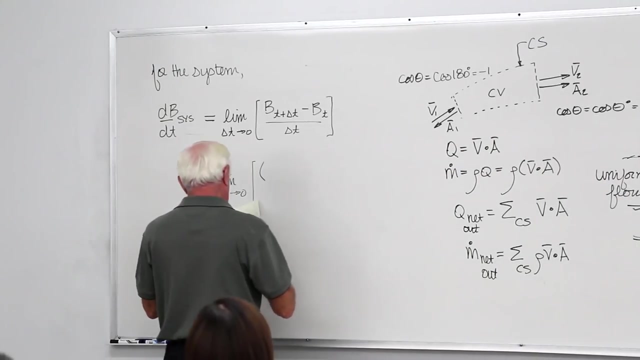 I'm going to call this region one, This region two, This region three. At time T equals zero. There's the system Black line: The amount of B in region one plus the amount of B in region two. Let's put that here. 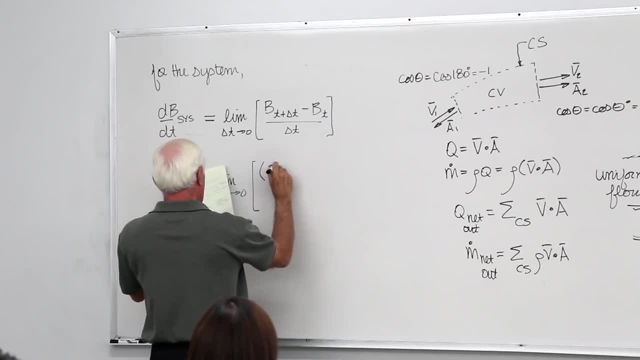 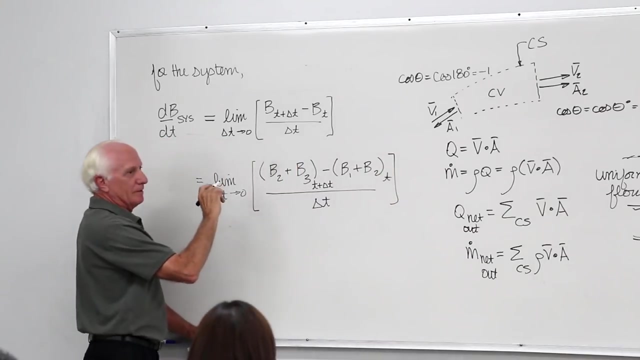 Let's do it this way. I'll put this down first and explain it. I'm going to keep this in the right order. Okay, The amount of B in region T was the amount of B1 plus B2.. Okay, T plus DT. 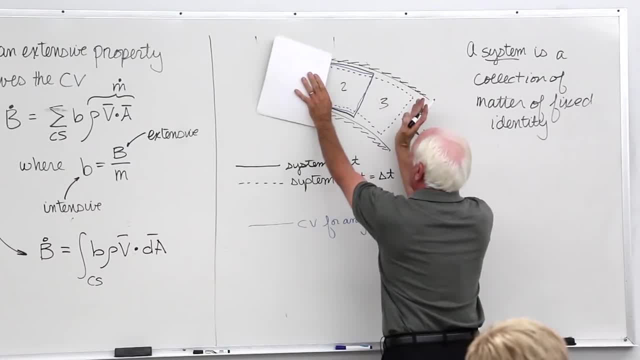 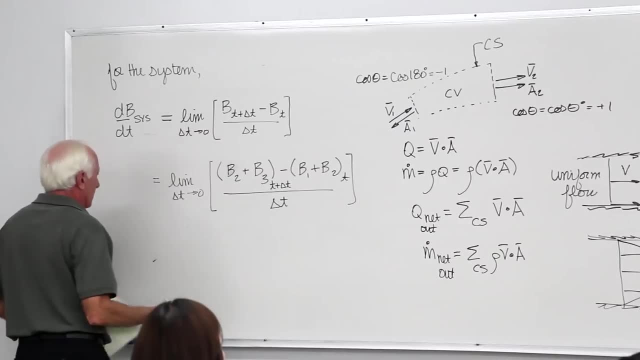 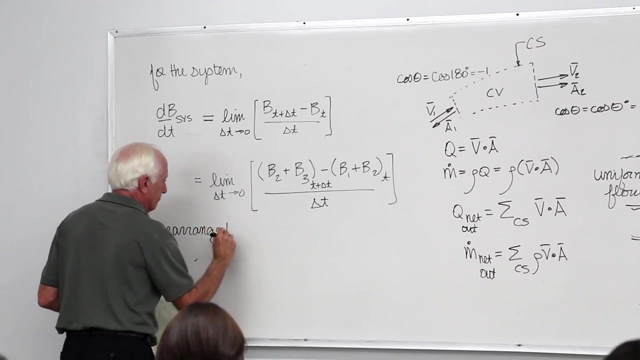 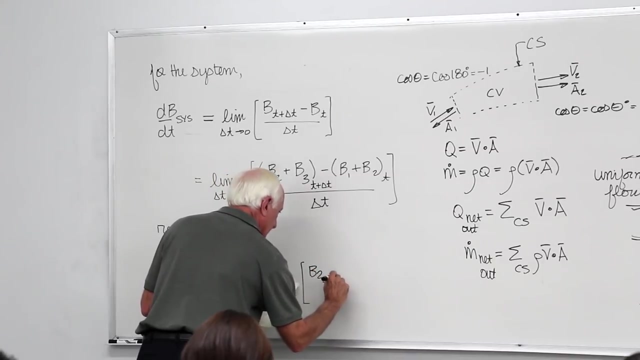 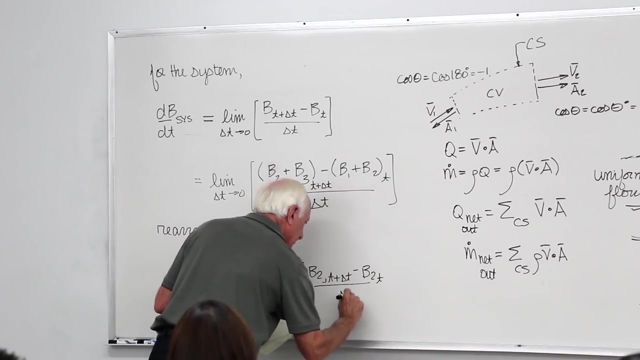 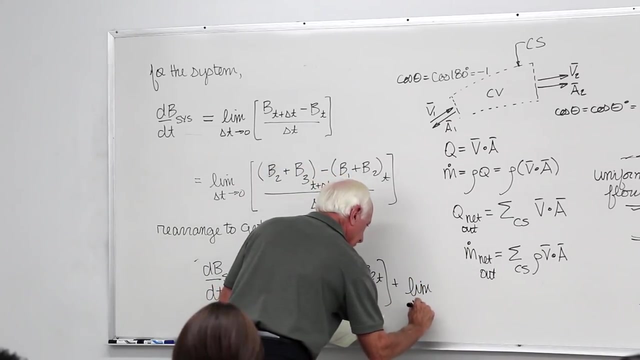 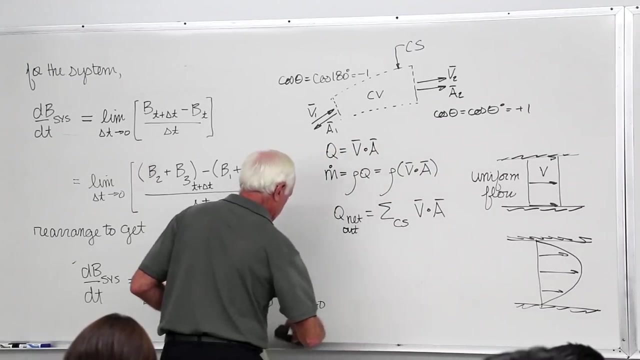 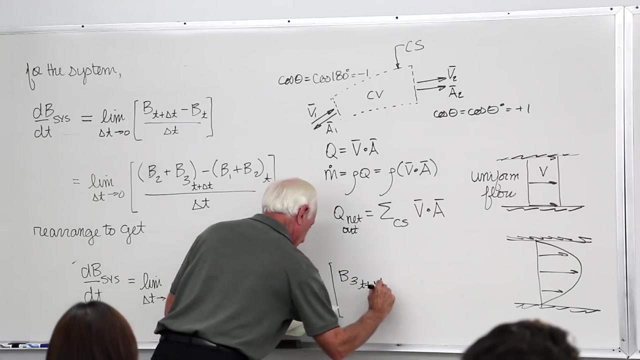 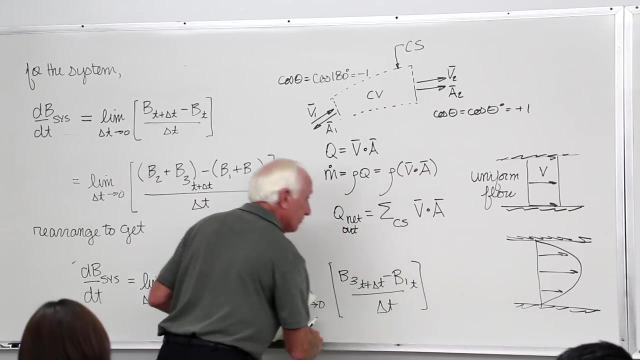 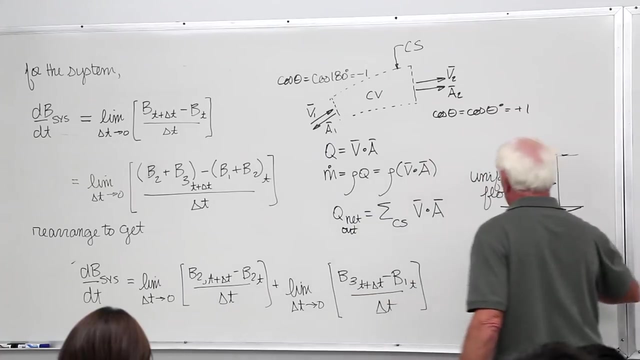 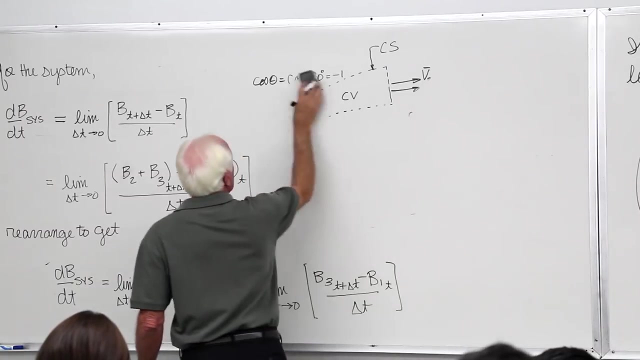 System at T plus DT Dash lines. Two plus three. Two plus three. Okay, Keep going. Rearrange DB DT System System. Thank you, You can see where the terms came from. Nothing new was added, It was just moving the terms around. 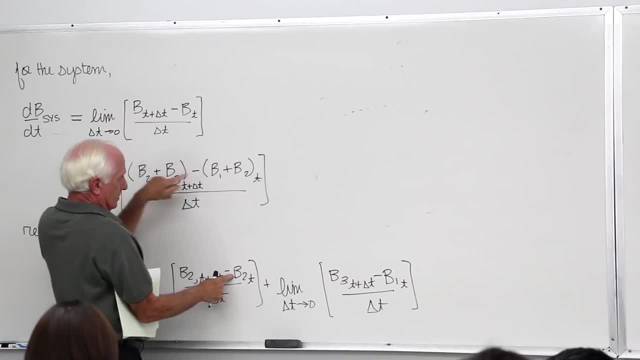 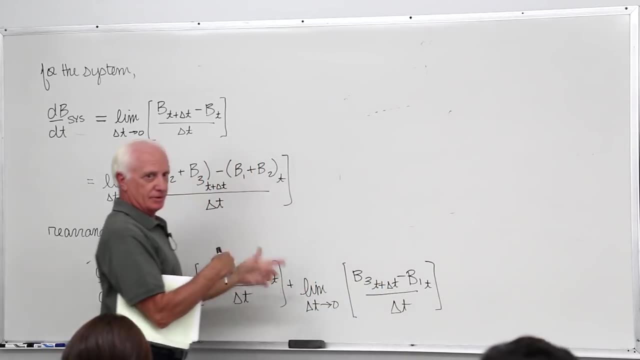 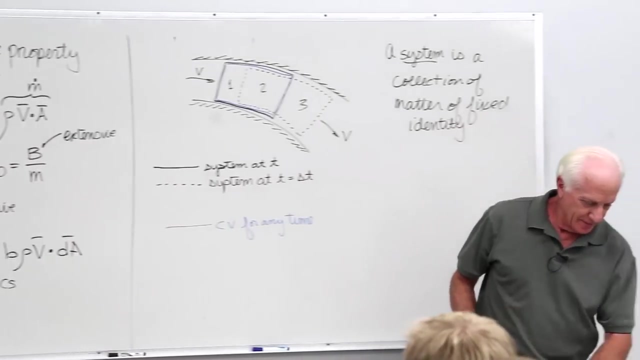 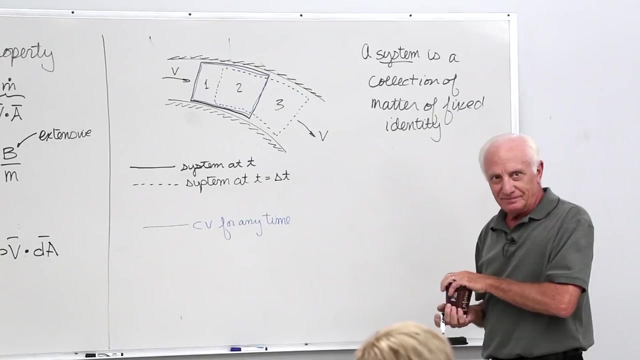 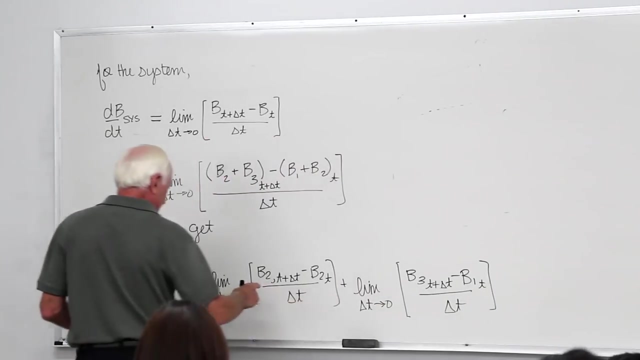 This term is this term. This term is that term. This term is that term. This term is that term. Yeah, Just rearranging the two. Okay, Let's look at this term first. The amount of B in region 2.. 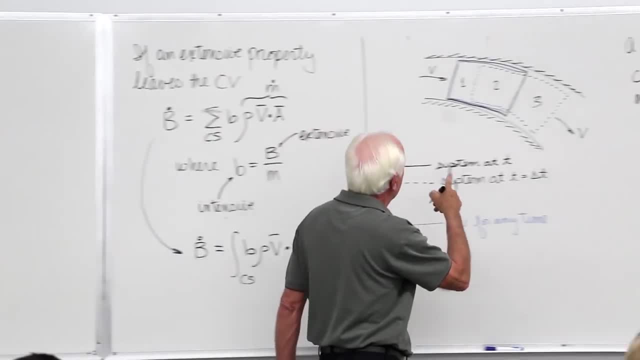 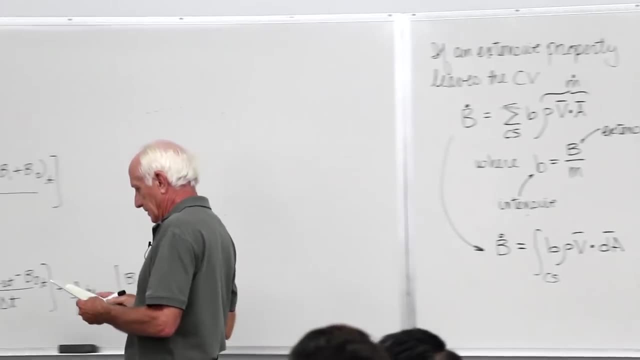 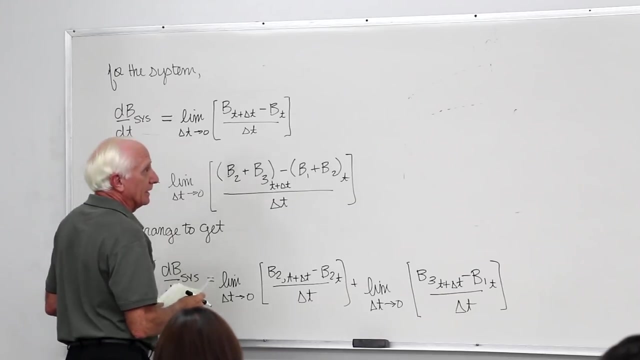 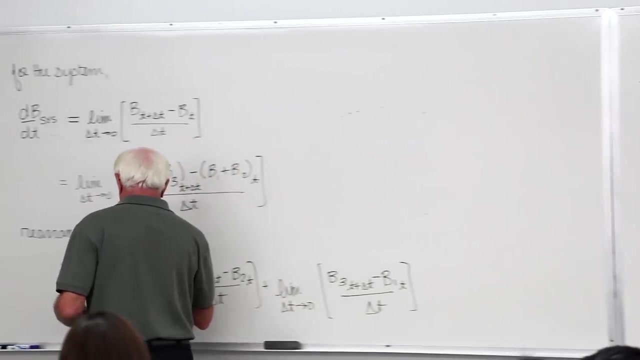 Okay, What's region 2? That's right here. Okay, In the middle, here In region 2 at time t plus bt at time t. Okay, All right. So this guy right here in the limit. db, cb, dt. 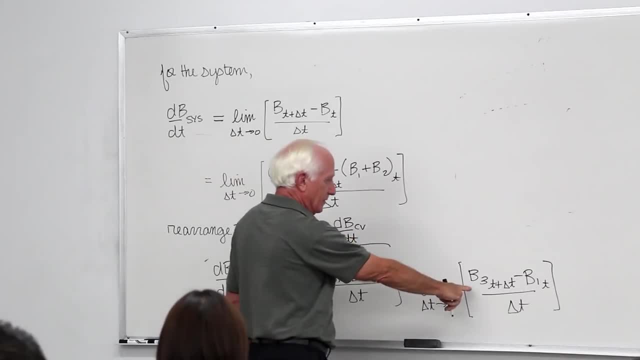 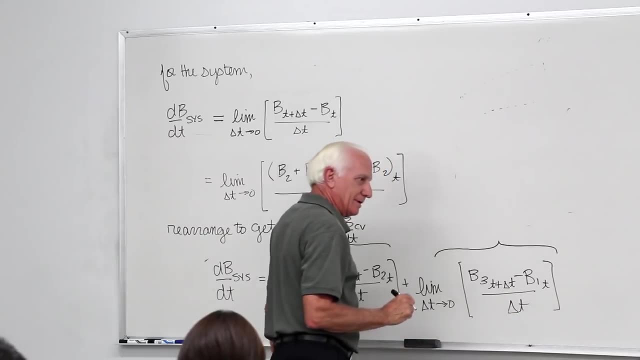 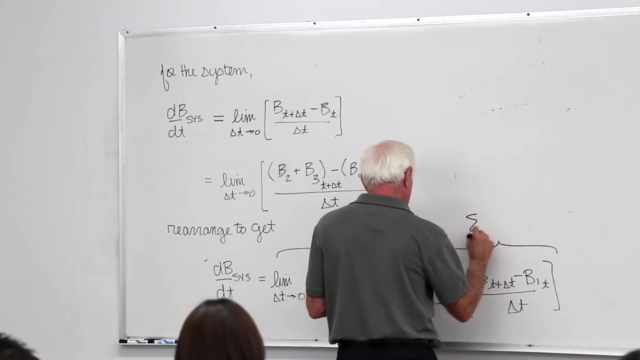 This guy right here: what went out minus what came in, What went out minus what came, The amount of B that went out minus the amount of B that came in. Okay, So this term right here, Right And here So. 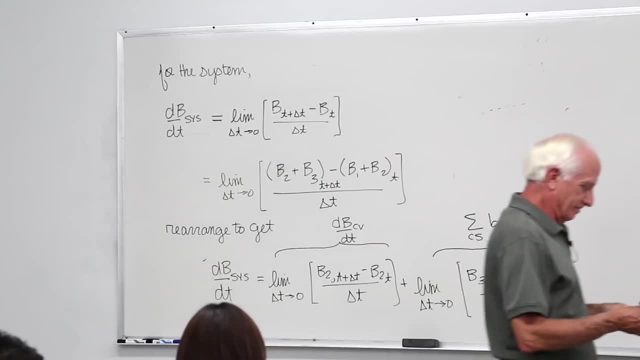 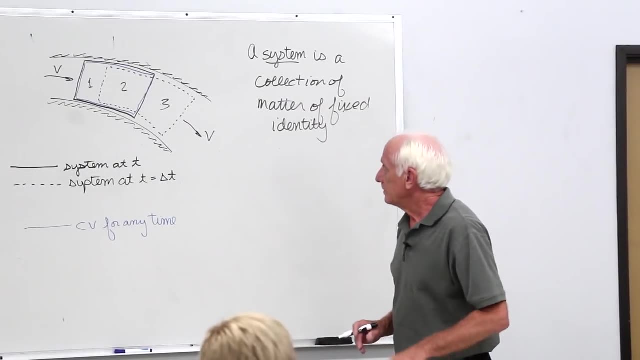 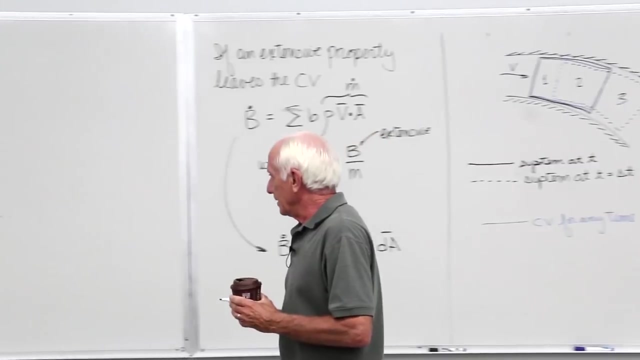 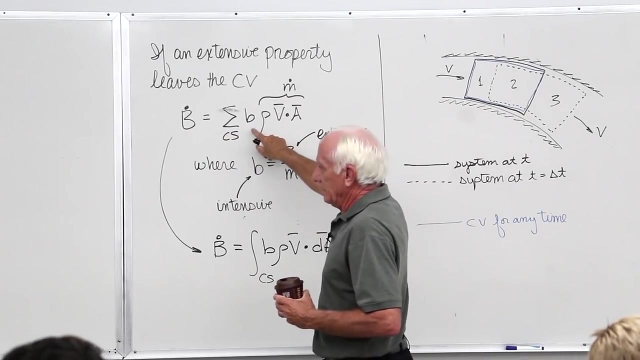 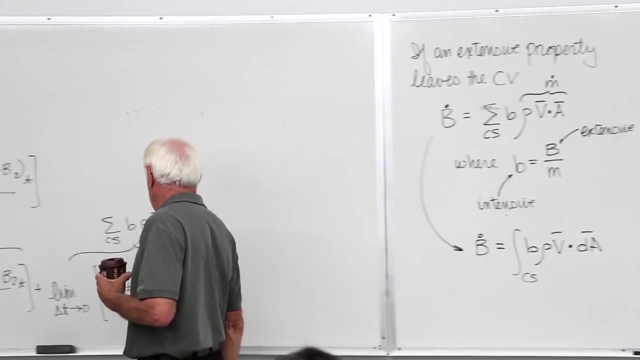 Okay, So we've got now. where did this guy here come from? I just erased it. unfortunately, Maybe it's still up here. Yeah, okay, here, it is right here. B dot A is what came out minus what came in. So that's what that term is. Let's. 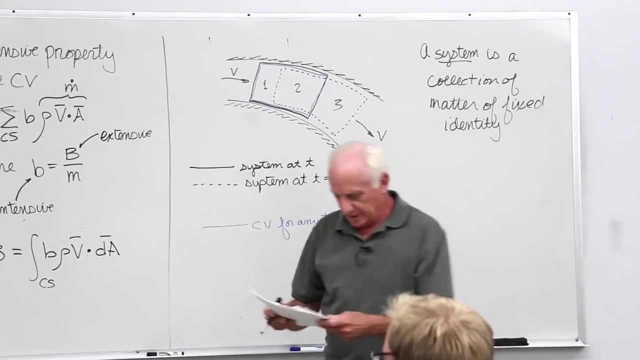 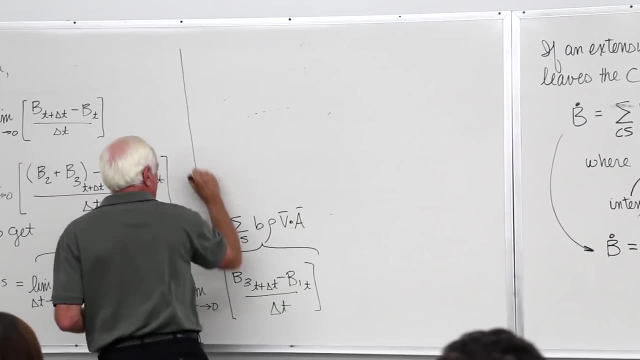 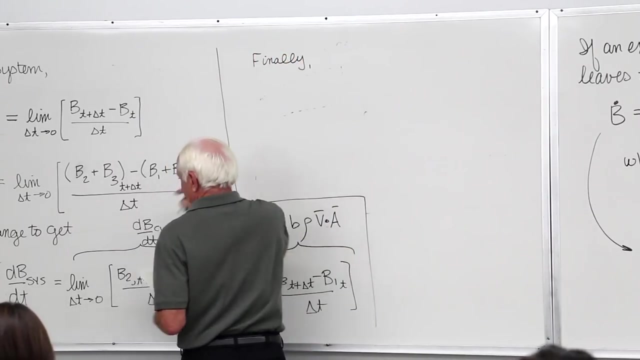 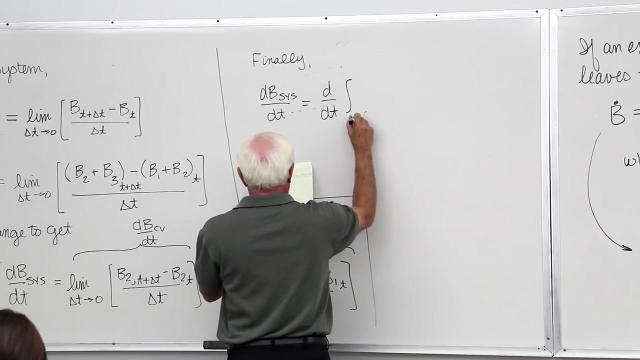 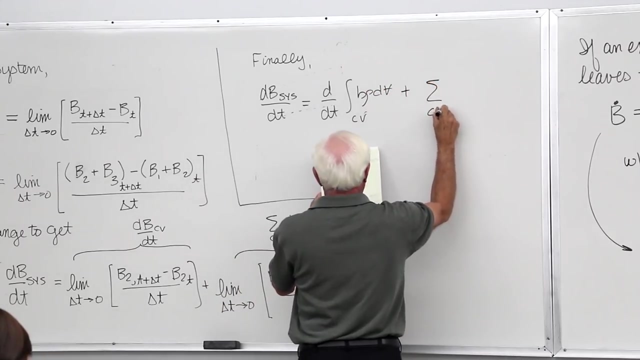 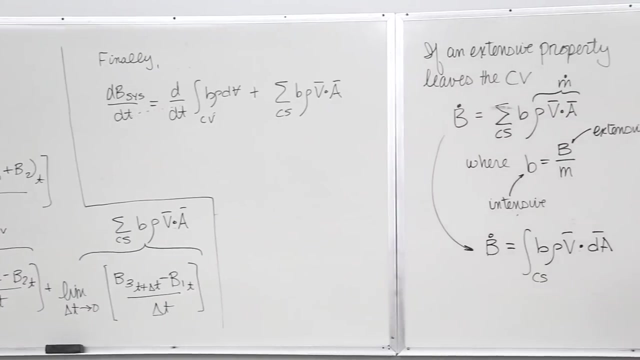 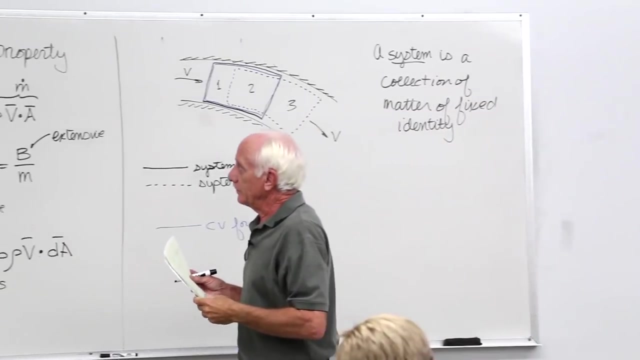 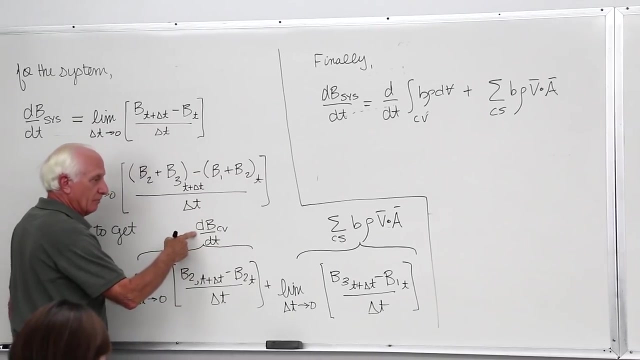 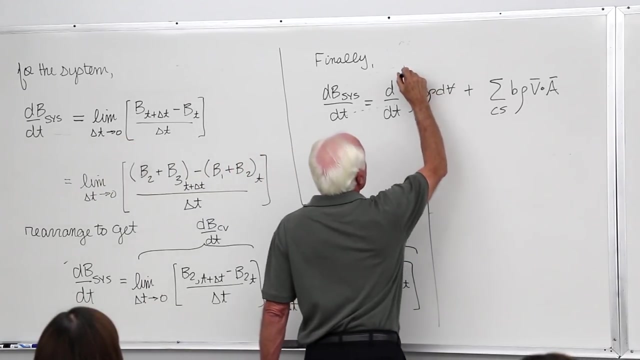 then combine these two into one equation. We'll put that up here, I think. Okay, DB system, DT, DDT. Okay, Now we did this guy right here. This is the amount of B in the control volume, the change of it with respect to time. This is the amount of B in the. 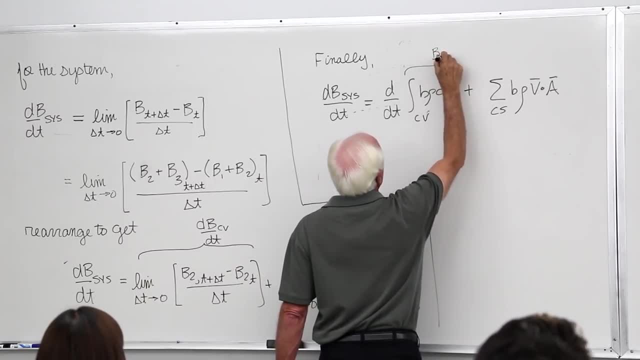 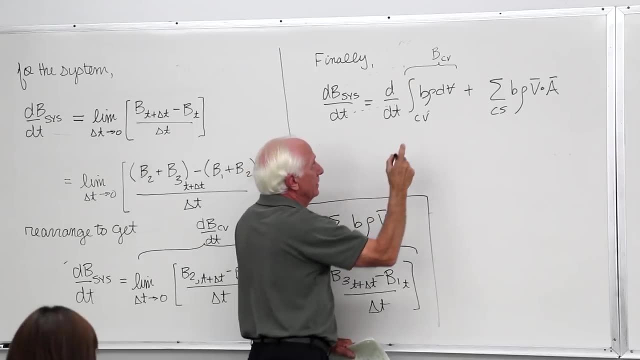 control volume. So this is the amount of B in the control volume. So this is the amount of B in the control volume Integrate over the control volume. Let's see what the integration is. What is? I'll just pretend it's SI. What is B? Okay, 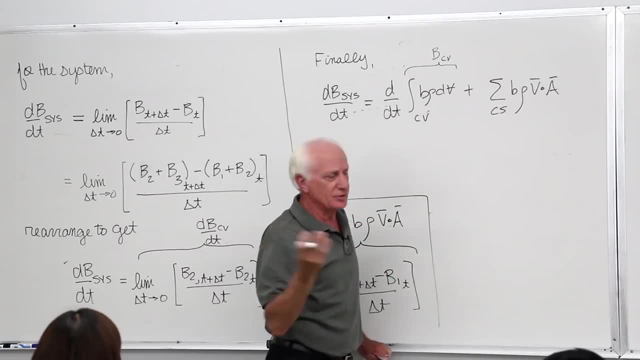 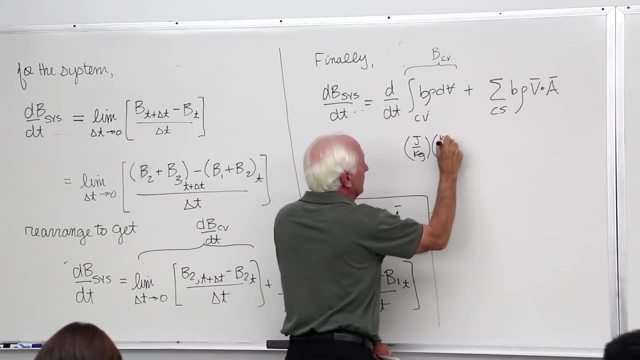 let's just say B is joules, again just to make something up Energy in joules. So B is joules per kilogram. What is rho? Kilograms per cubic meter? What's the volume? Cubic meters? When you're done, what do you have? Joules, That's the. 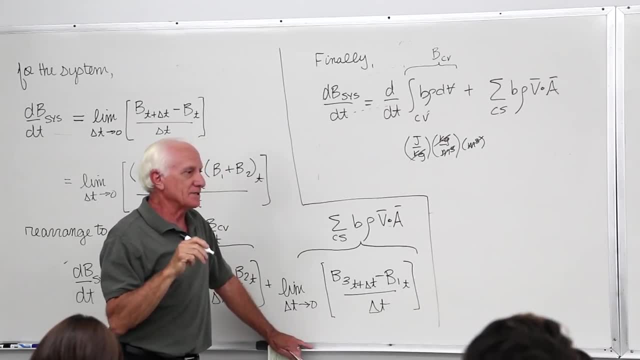 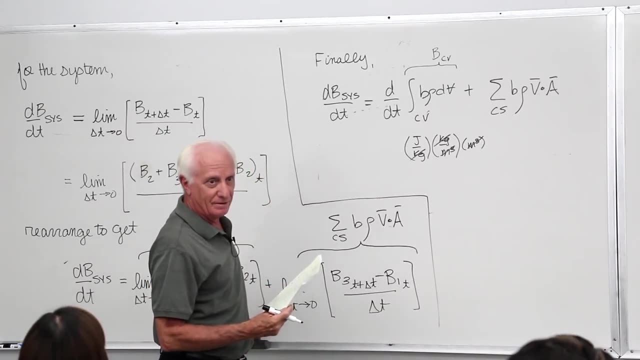 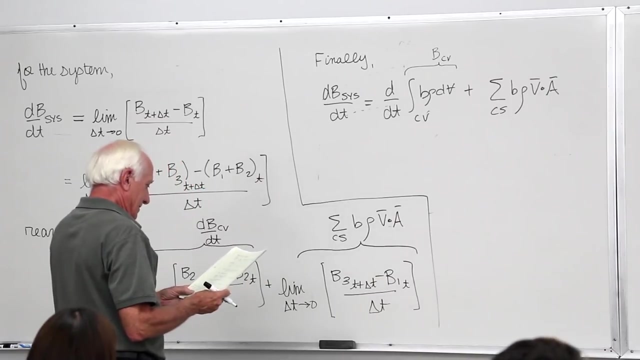 amount of B in the control volume as a function of time. That's what the interval represents. If it's steady state, of course, goodbye. Nothing compared to time. That term goes out for steady state. Okay, we're almost there, This one Time rate. 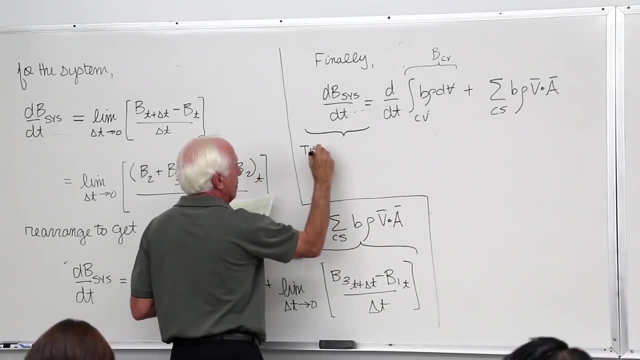 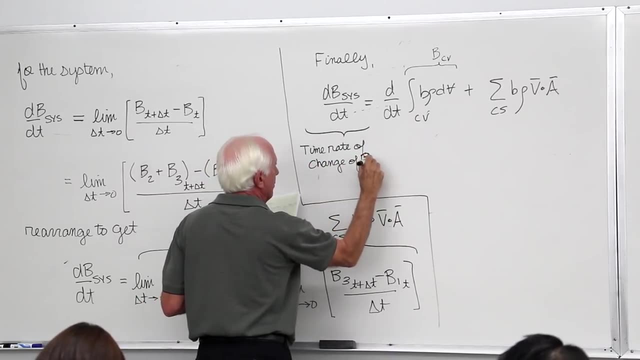 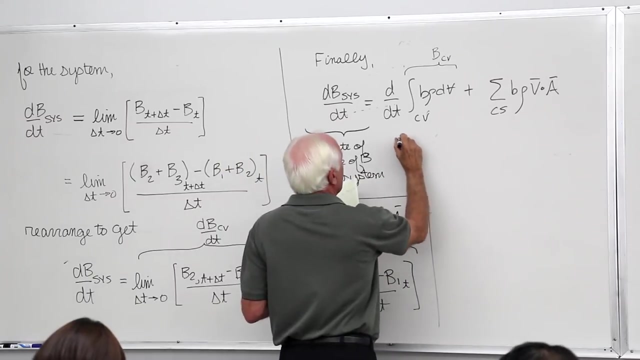 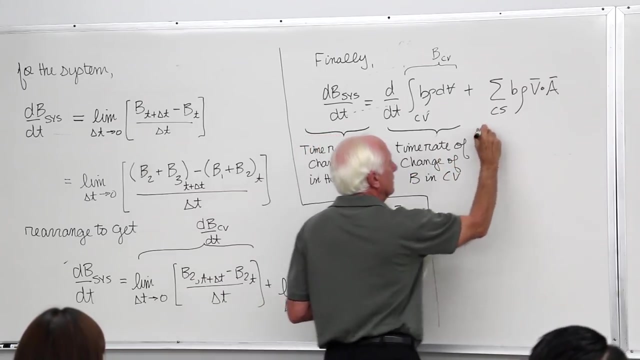 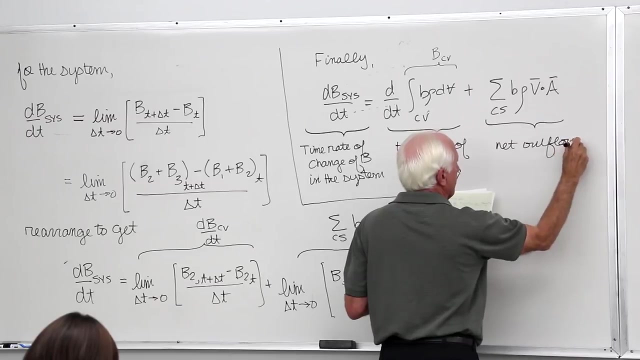 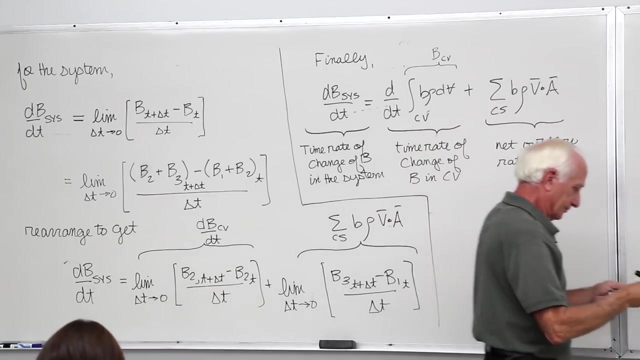 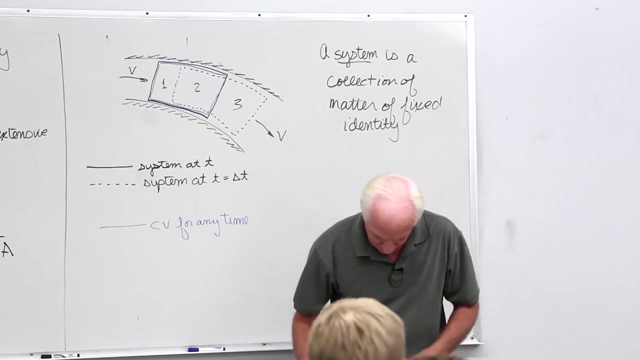 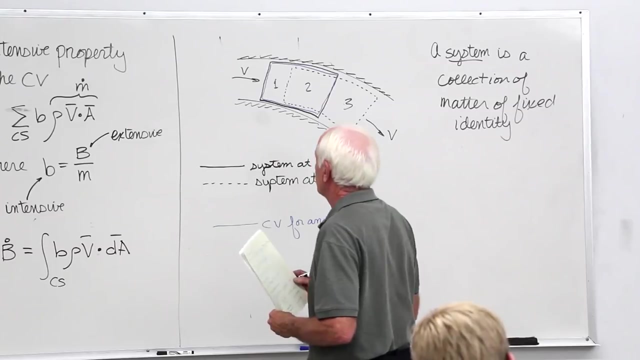 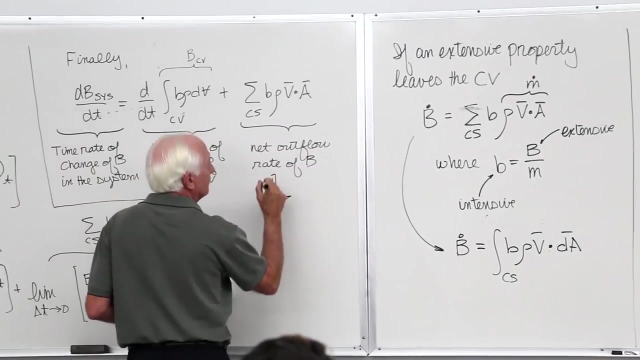 of change of B in the system. This one Time rate of change of B in the control volume, This one Net outflow rate of B. Okay, This guy here, if you want to. if it's not uniform flow, okay, remember. 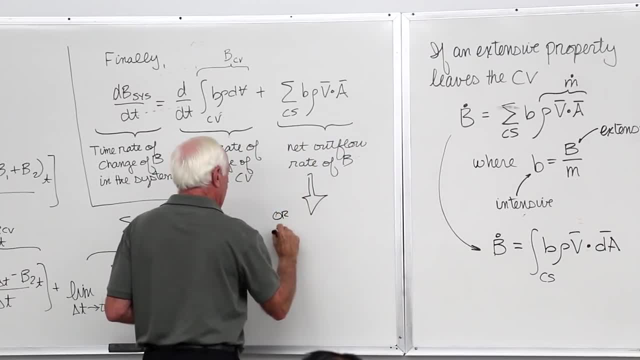 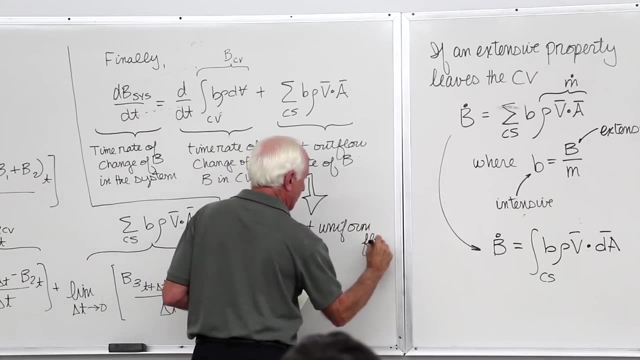 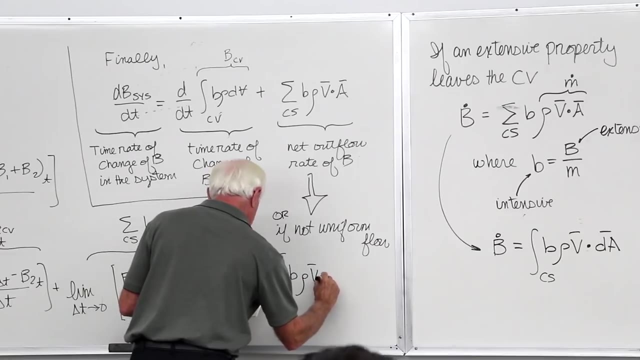 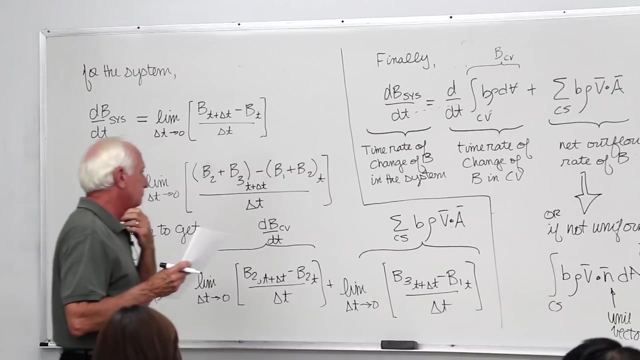 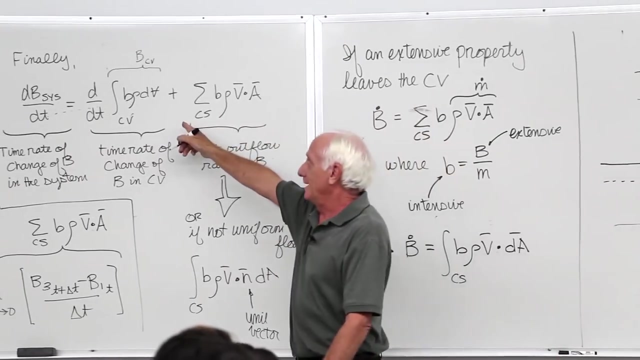 if not uniform flow, or if not uniform flow, then we have the integral of B, Rho, B dot, N, dA. This guy unit vector in the N direction. Okay, I can't box it in, There's too much up there. That final equation, right. 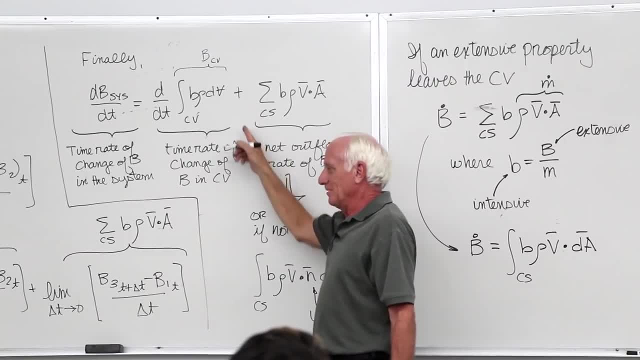 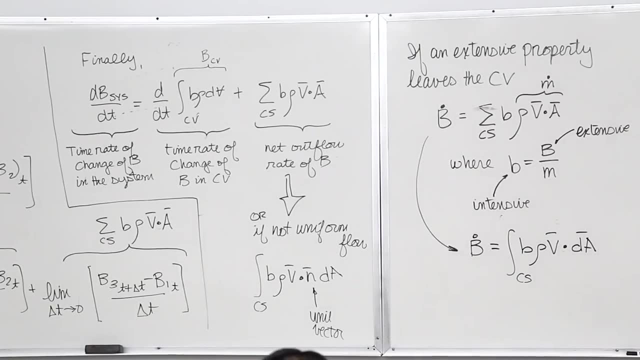 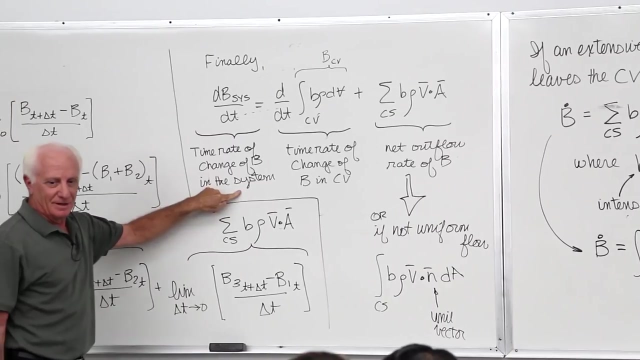 there, in symbolic terms and word terms. that is the transport theorem, Reynolds transport theorem. What does it relate? Well, it relates to the left-hand side, And there's the word, of course, Changes in the system, as the basic laws of science are generally expressed in. We engineers want it. 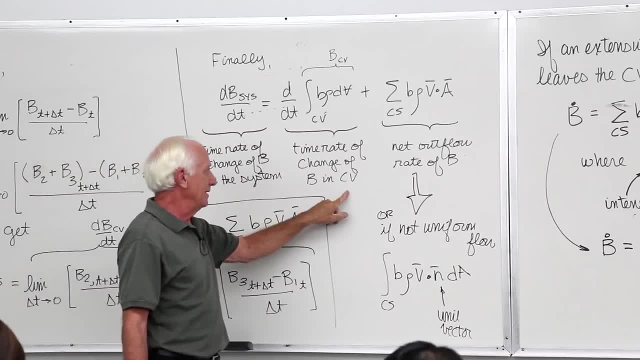 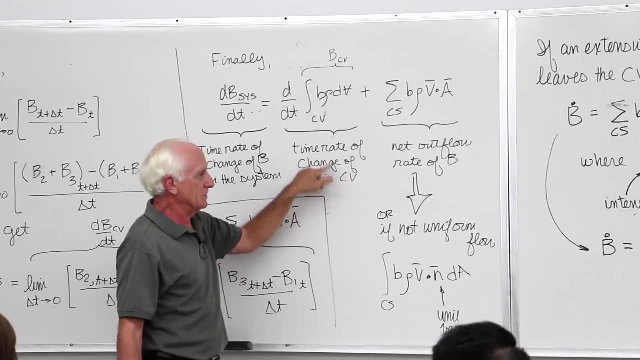 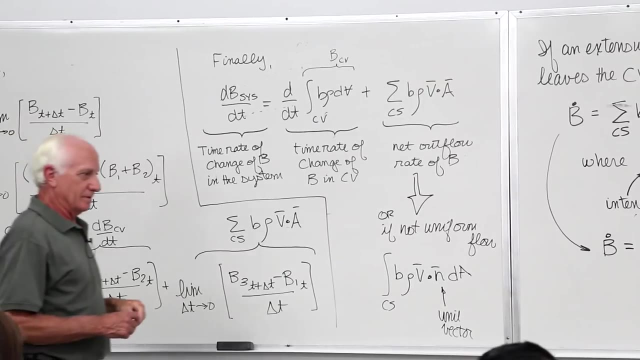 expressed in control volume terms. So the right-hand side is the control volume terms. Control surface there, control volume here. If it's steady state, that term goes out. Okay, So that's what we're going to use for mass momentum and energy in Chapter 5.. 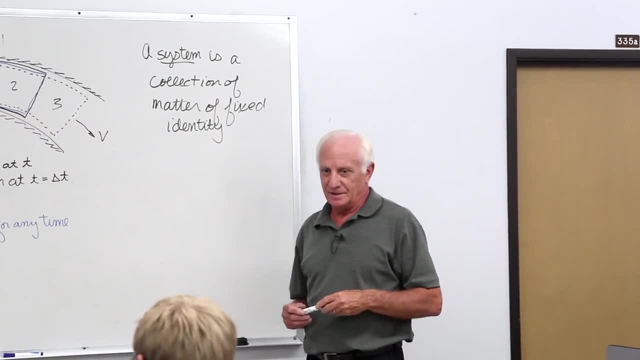 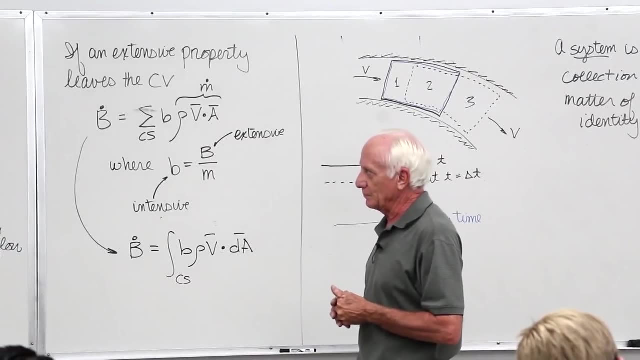 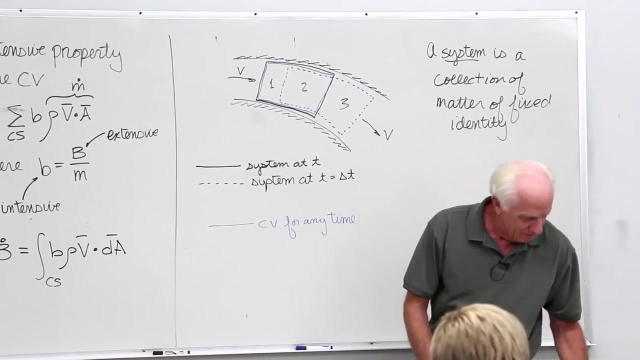 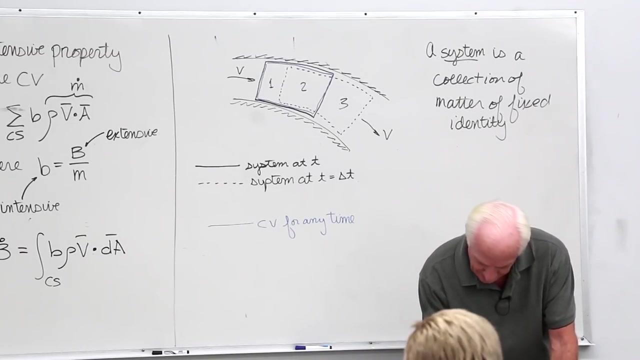 We'll let capital B be mass first of all, then momentum and finally energy, And develop three equations from that Reynolds transport theorem. Okay, So you have an example for homework. Let me see which one has sign. Yeah, You have 68 and 69. I'm going to work problem 7.. It's somewhat similar to 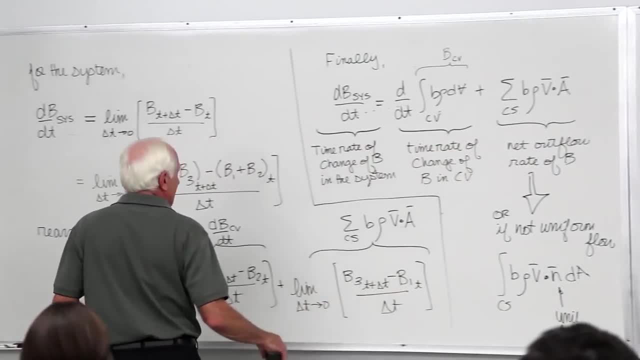 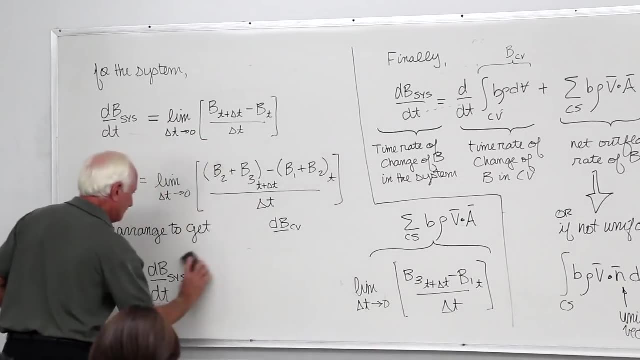 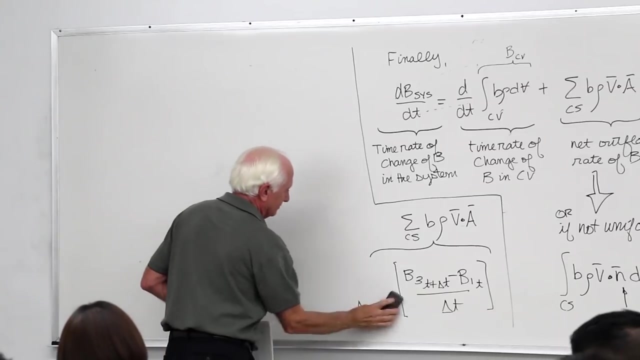 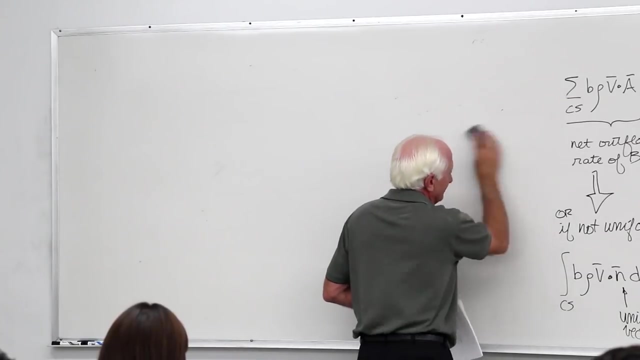 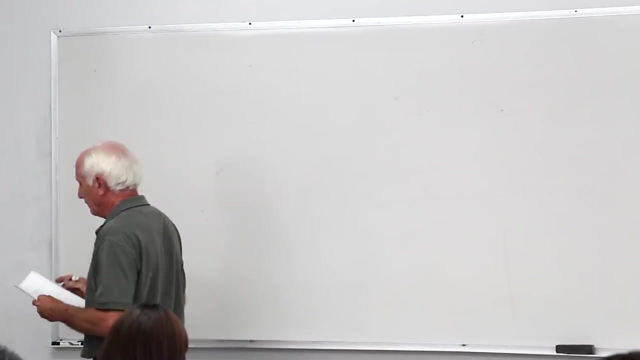 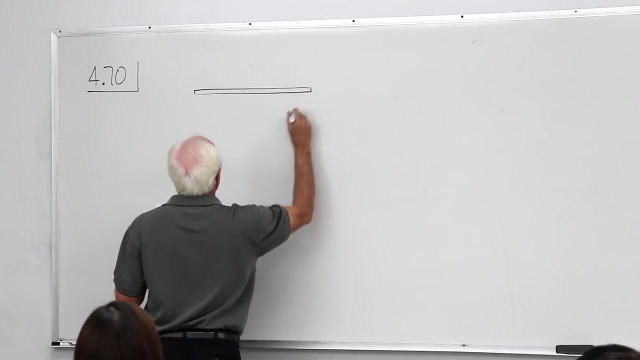 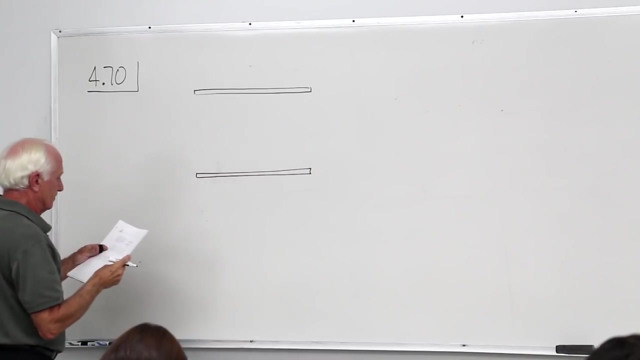 us 69.. So, let me, I don't need this, I need that over there, maybe We'll see. Okay, Let's see what problem 470.. Let me draw a picture first. Here's a picture given in a textbook. There's two plates folded in opposite directions. 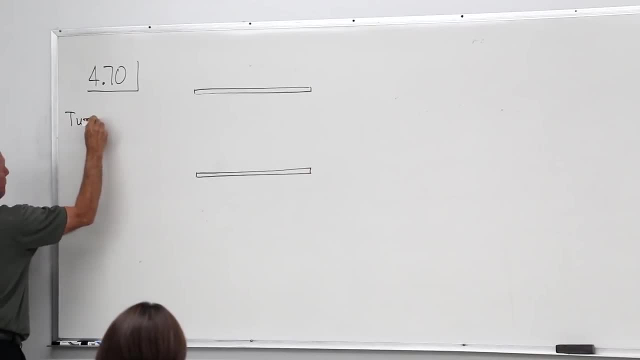 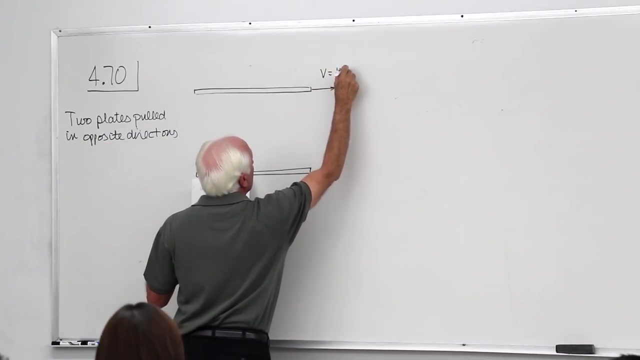 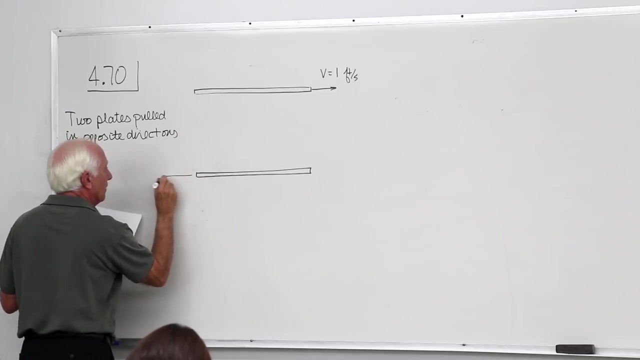 Folded in opposite directions. And let's see here: The speed of the plates are 1 foot per second. So this plate is being pulled this way, Velocity equal 1 foot per second, And the other one is being pulled to the left at 1 foot per second. Okay, Oil is between the two plates. 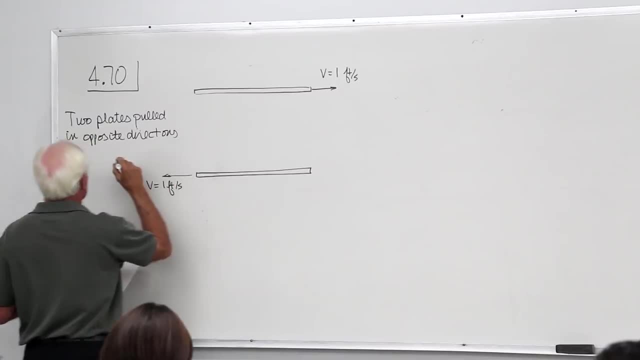 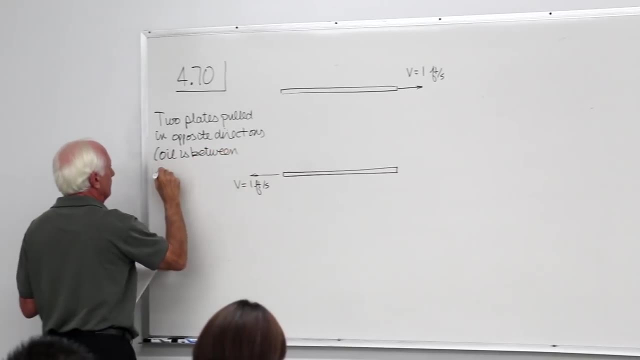 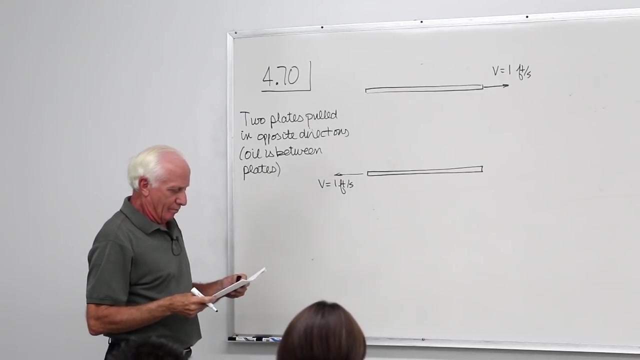 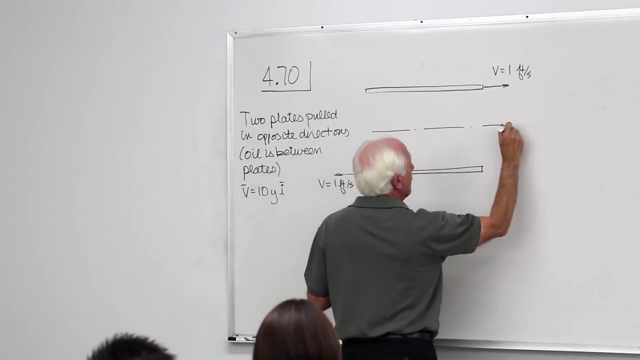 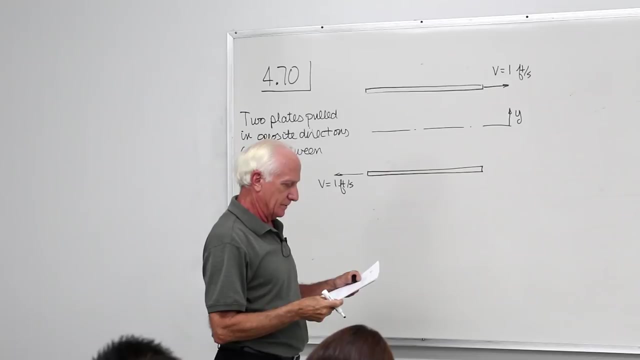 I'll just put it here, Okay, Velocity is 10y times i, 10y times i. y is measured from the middle And the distances are, let's see, 0.1 feet, I'm sorry, 0.2 feet. 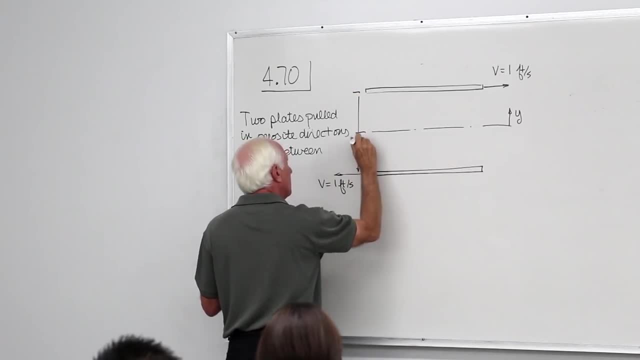 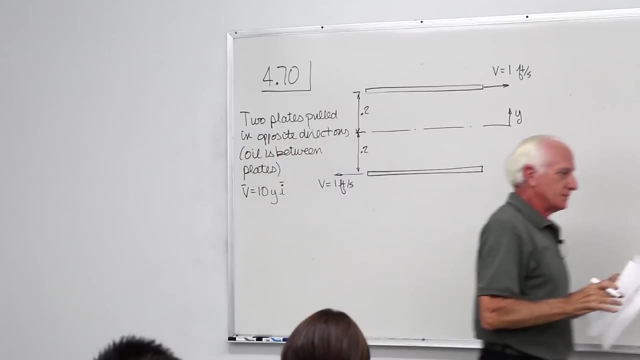 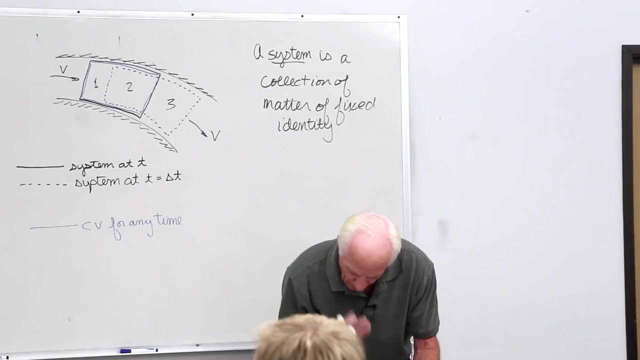 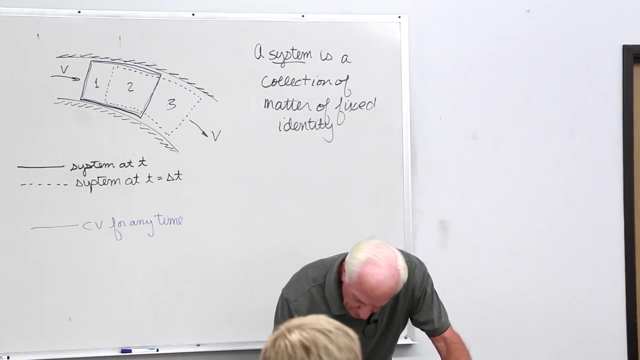 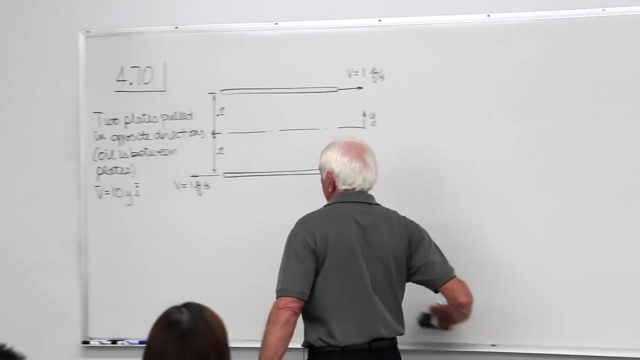 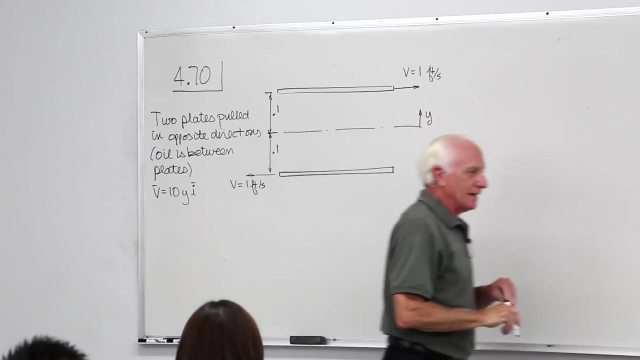 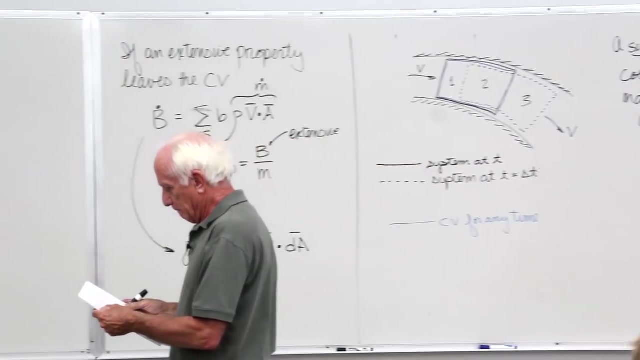 Let's see, Let's just make sure that's what it is: 470.. I don't understand. No, it is 1. 110.. 110.. Okay, Now let's see what else to find. Okay, Fixed control. volume A, B, C, D. 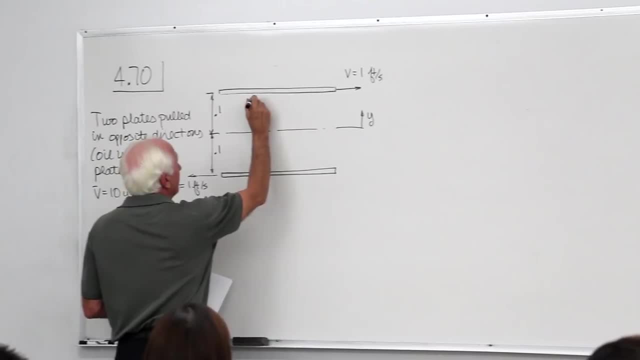 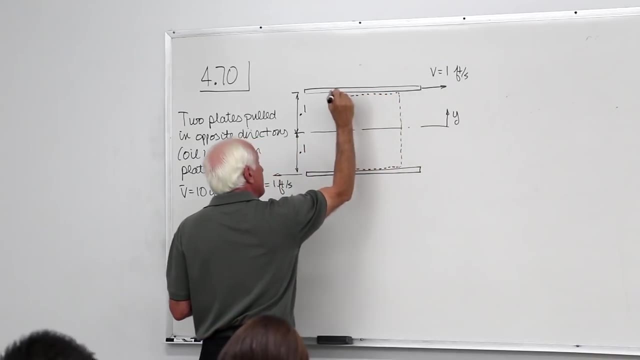 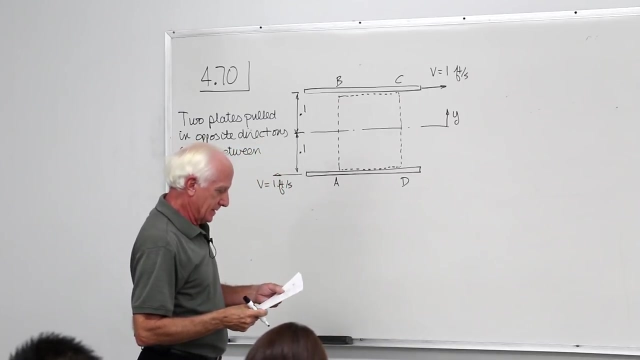 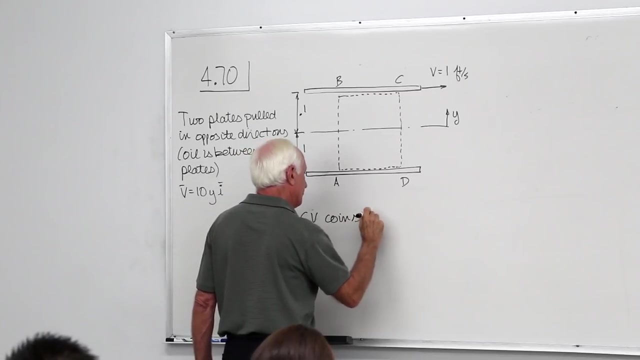 2 tenths, 2 tenths, Okay. Fixed control volume: Okay, Let's see A, B, C, D Got it. That is showing this coincides C, V coincides With system at t equals 0.. 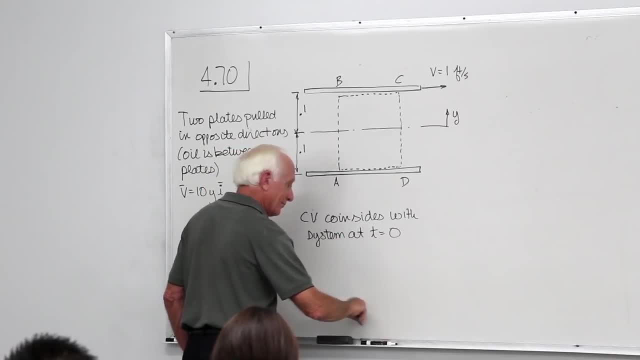 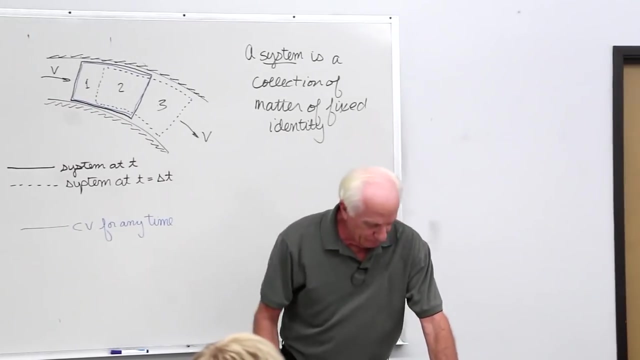 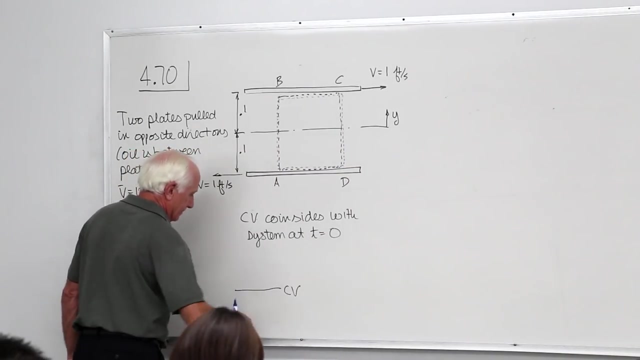 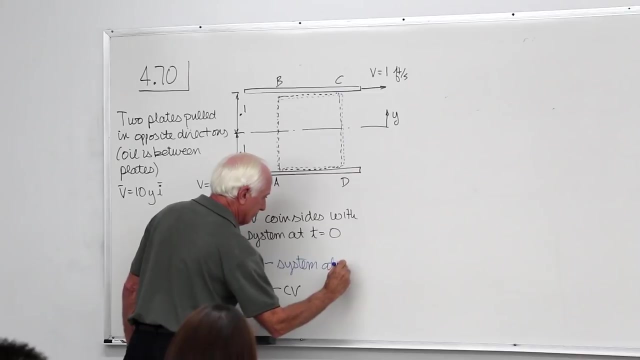 So here's the system at time 0.. Okay, The system at time And the control volume for any time. Control volume is not moving. This is the fixed control volume. Okay, Okay, Let's see now That's still given. 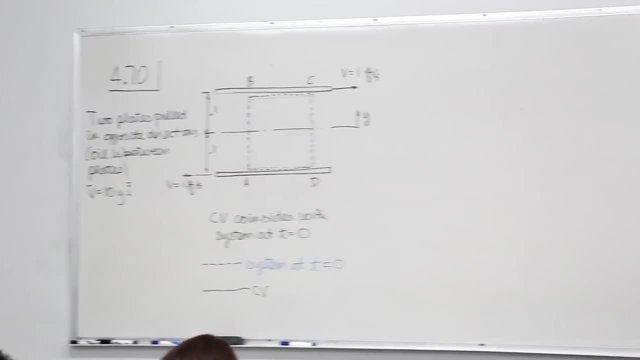 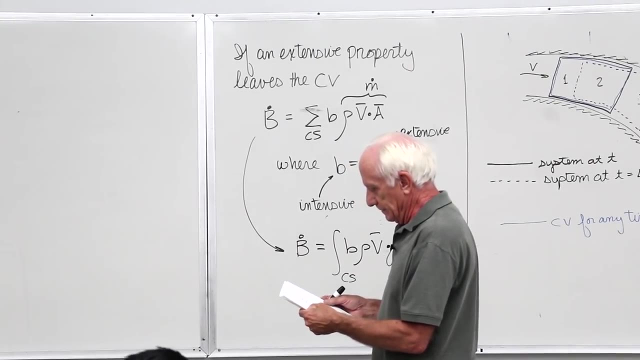 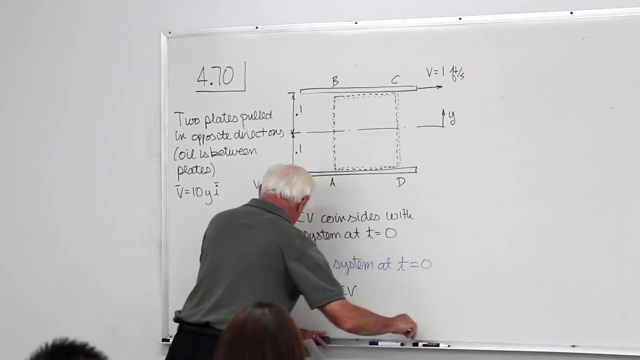 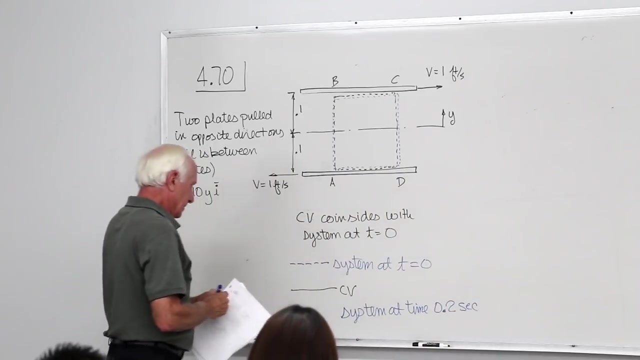 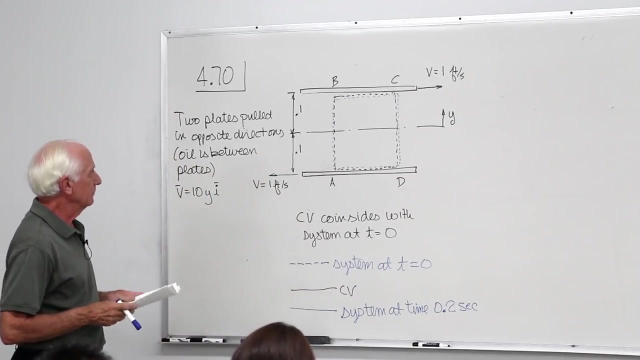 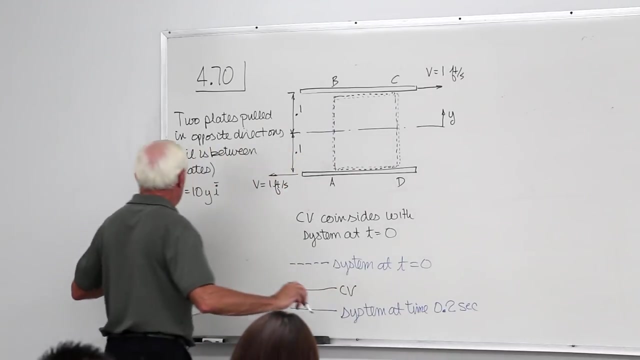 Okay, Let's see now That's still given. Keep reading. Indicate the system at time: t equal 0.2 seconds. So system at time: 0.2 seconds. It's going to be a solid blue line. The velocity: Okay, Let's draw the velocity. 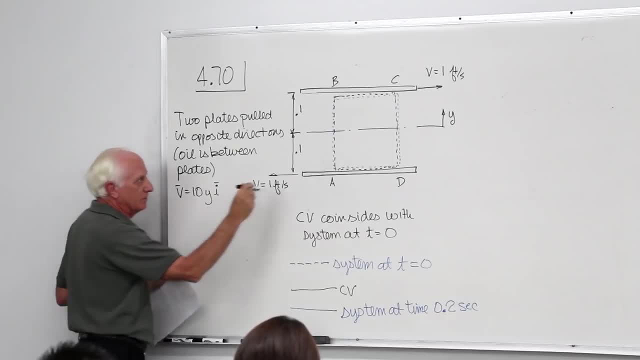 At the center, y equals 0.. Velocity equals 0.. Okay, At the top, y equals 1 tenth. V equals 1.. At the bottom, y equals minus 1.. Yeah, V is 1.. Between the two, v is a function of y, only Linear. 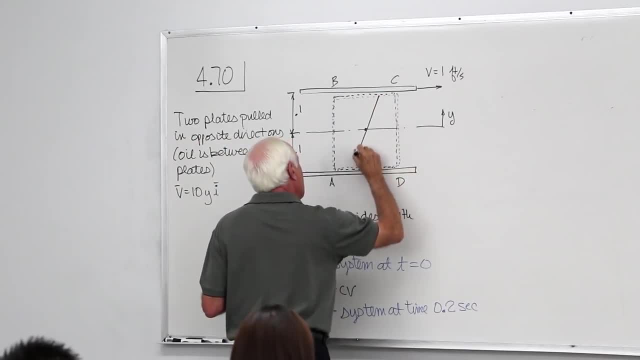 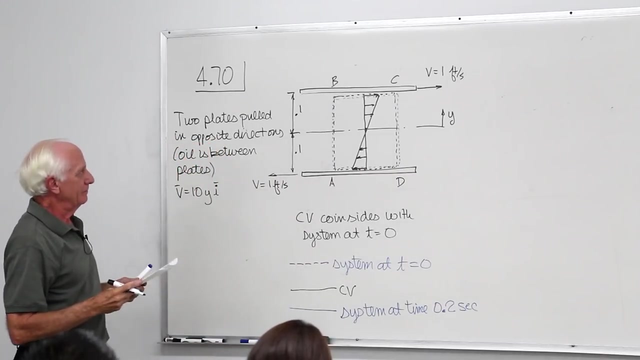 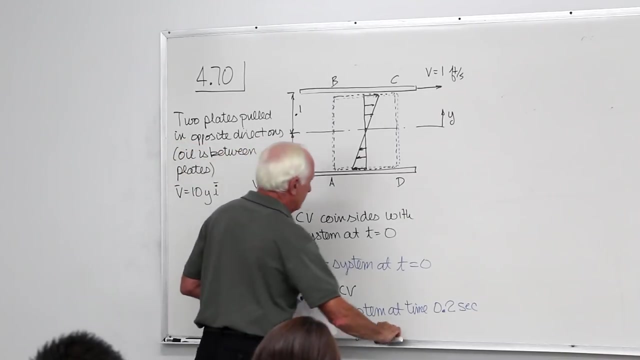 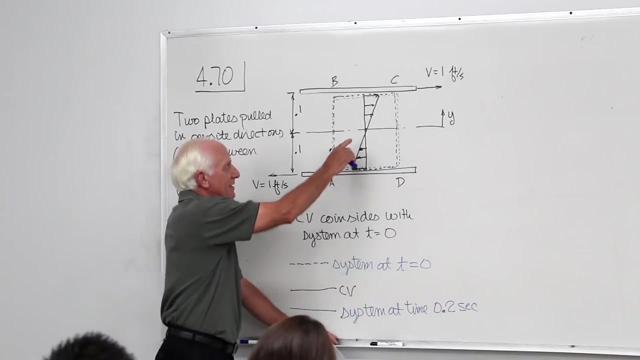 Linear. So it looks something like this. There's the velocity field for the oil. After 2 tenths of a second, did the oil molecule in the middle between the plates move? No, because the velocity is 0.. Did the oil particle at the very top move? 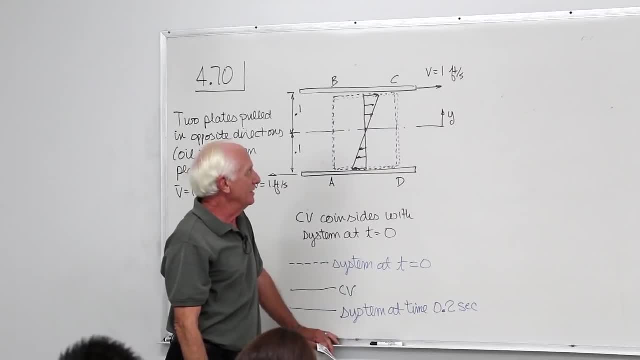 Yes, Which way To the right? How much It's going at 1 foot per second For how long? 2 tenths of a second. 1 times 2 tenths. It moved over 2 tenths of a foot. 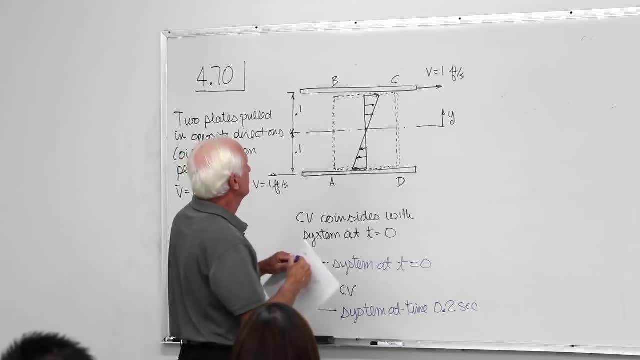 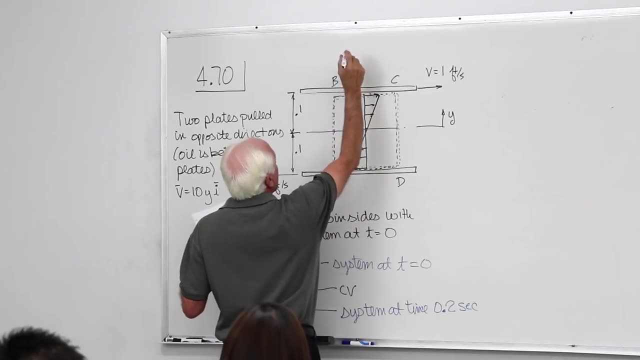 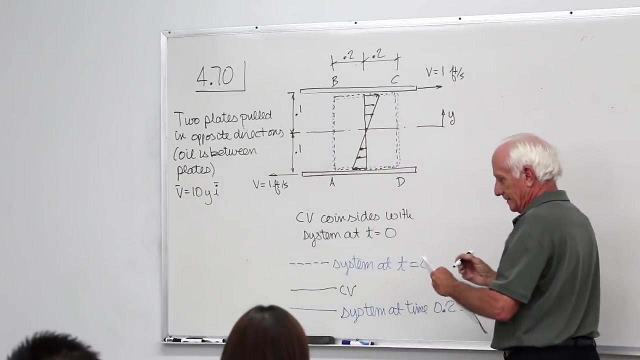 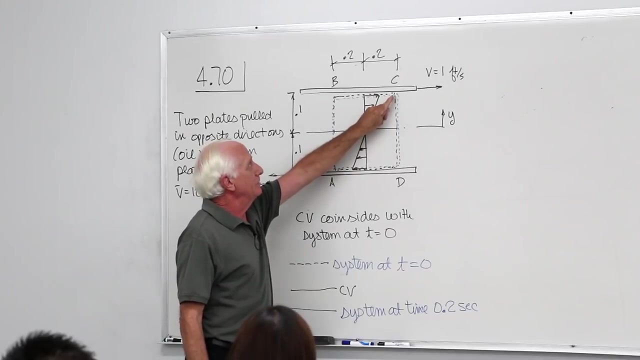 By the way, I didn't put this on here, but it started out at 2 tenths and 2 tenths here. This was given. I'll leave it like that. It's okay. Okay, So that top oil molecule was right there at time 0.. 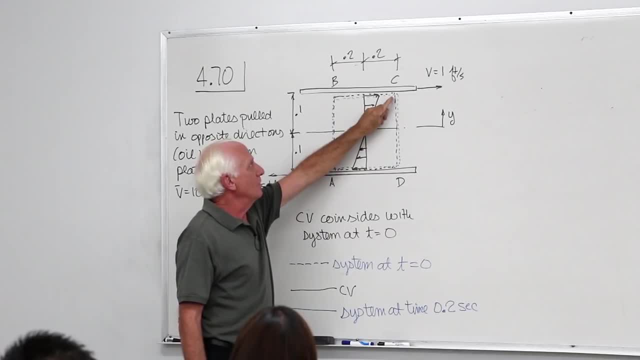 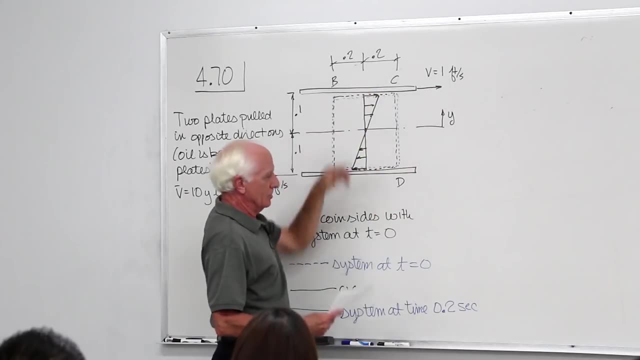 2 tenths of a second. It moved over 2 tenths times 1.. 2 tenths second times 1 foot per second. 2 tenths of a foot. Where did it start out? 2 tenths of a foot. 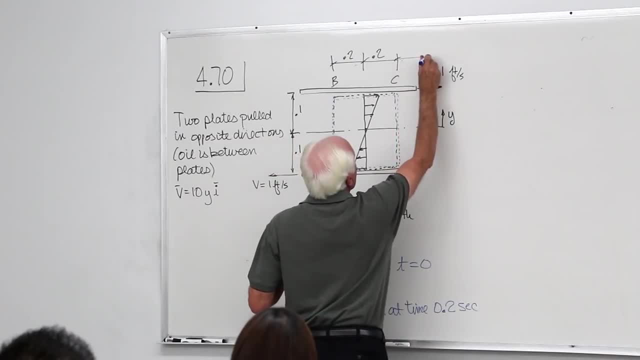 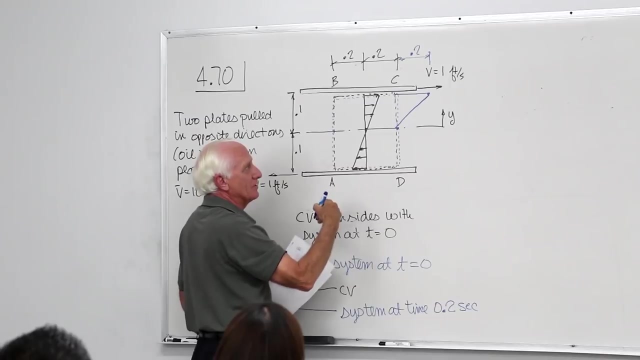 Where did it end up? Another 2 tenths out. This particle moved out here to there. Where did the middle particle move? It didn't move. How about the one down here? It went the other direction. This guy right here. 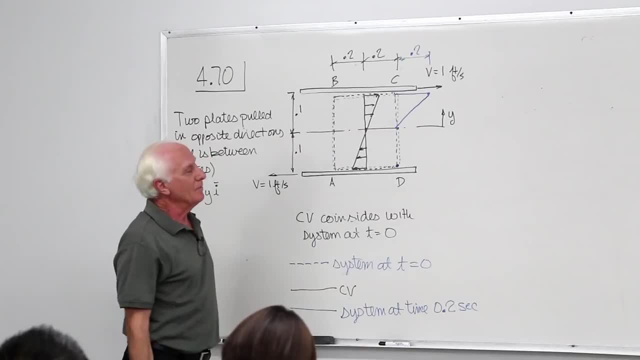 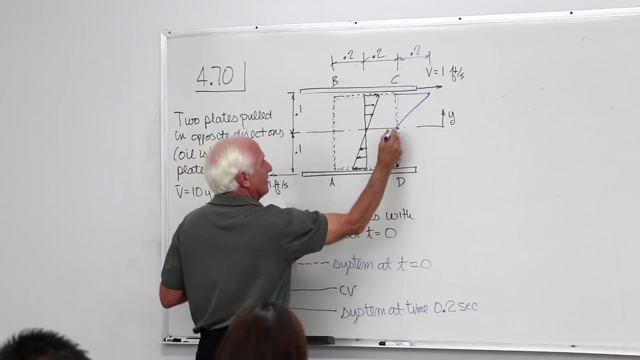 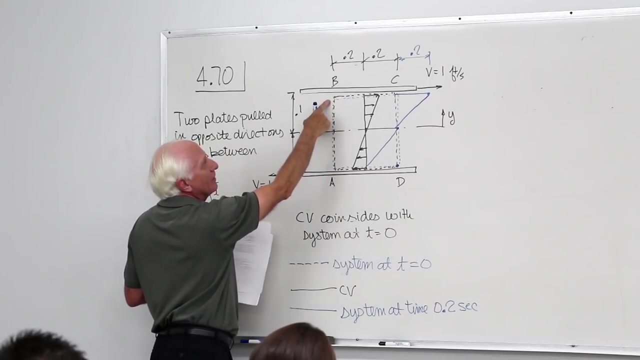 See The blue point is He went to the left. How much: 1 foot per second times. how long: 2 tenths of a second. He went 2 tenths that way. He's back here Now, the guy up here. 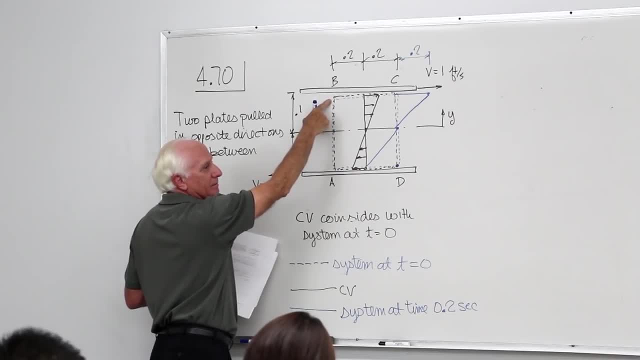 Oil molecule. Which way is he going To the right? At what rate? 1 foot per second. For how long? 2 tenths of a second. He moved 2 tenths of a foot. That way He's up here. The guy in the middle Did he move? 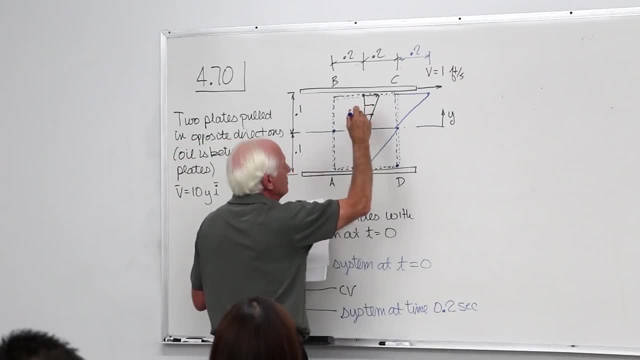 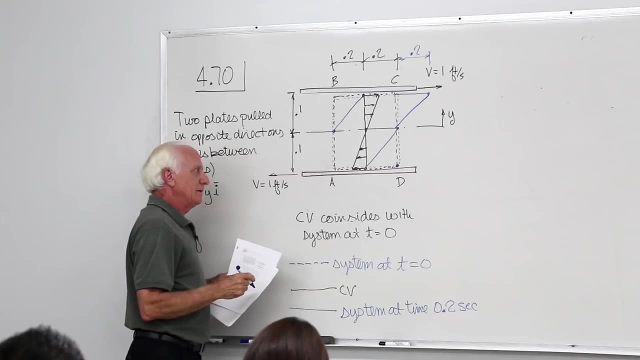 No, It's linear, of course. The guy at the bottom, At point A, The oil molecule on that plate, Did he move? Yes, he did. What's his velocity? 1 foot per second. Which way To the left? For how long? 2 tenths of a second, 2 tenths times 1.. 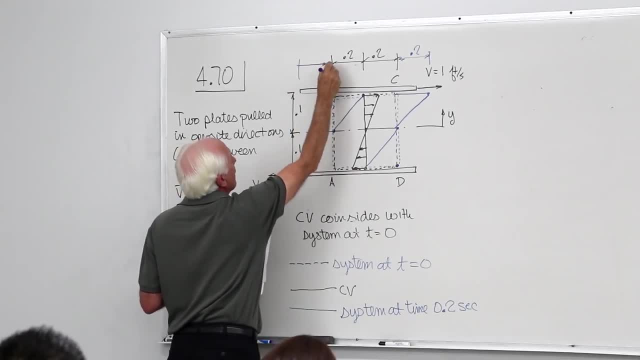 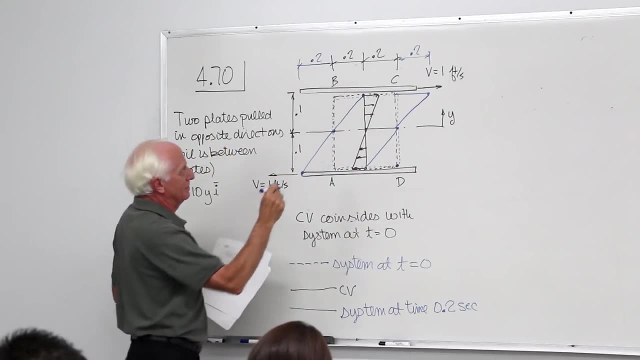 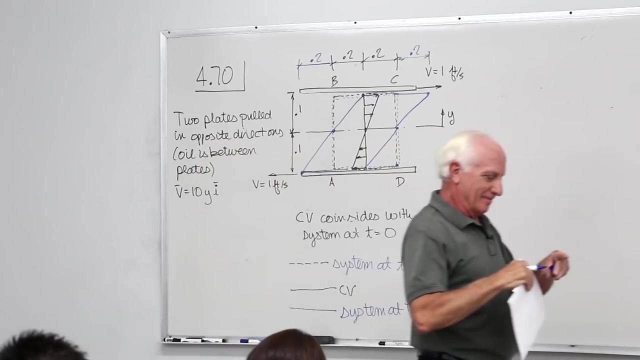 Okay, He's out here. now 2 tenths- He's right. here Now the blue In this chapter. here you better have multi-colored pens and good sketching techniques, because you're going to need it. This is nuts. 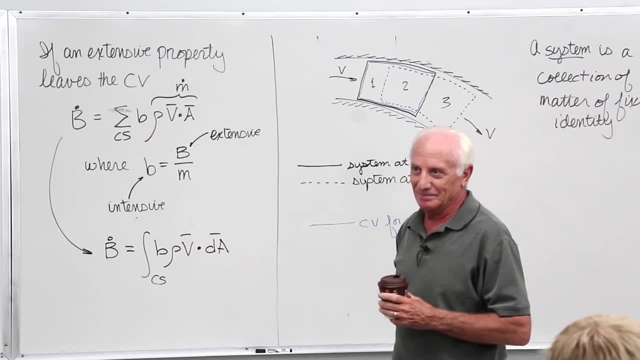 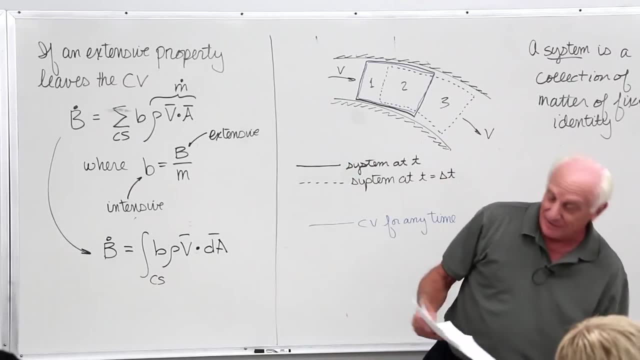 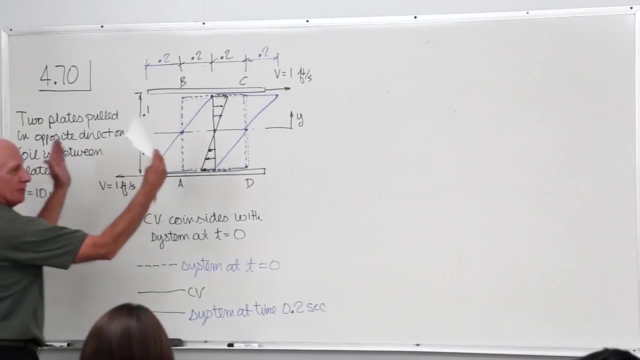 And don't make these things postage stamp size. You're crazy. Make them big. That's the answer. Where is the system? after 2 tenths of a second In the blue boundaries It got skewed like this. The last part. 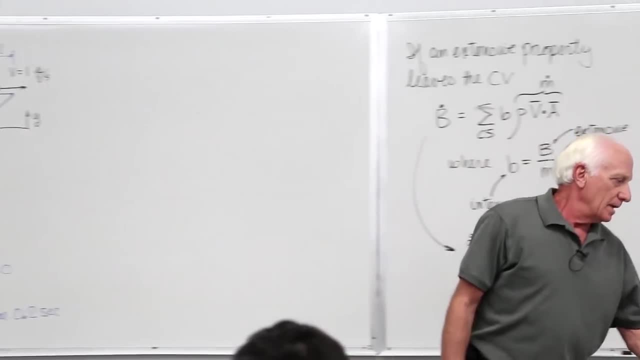 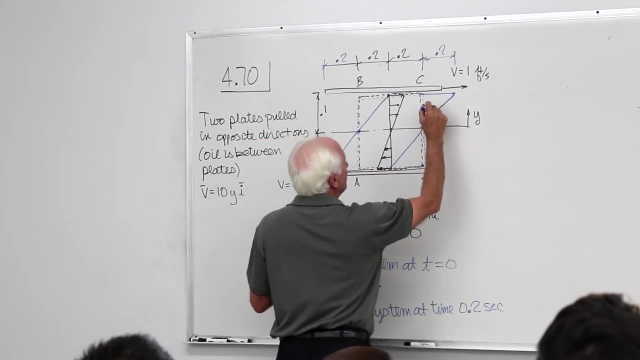 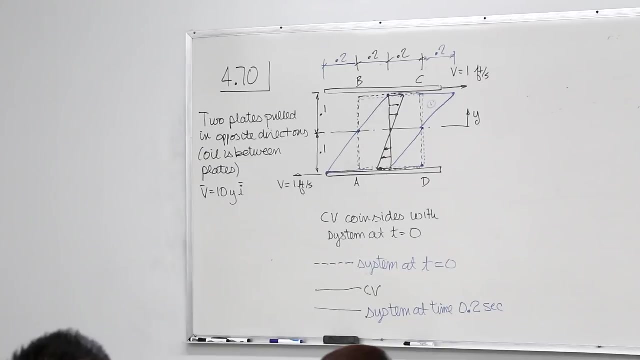 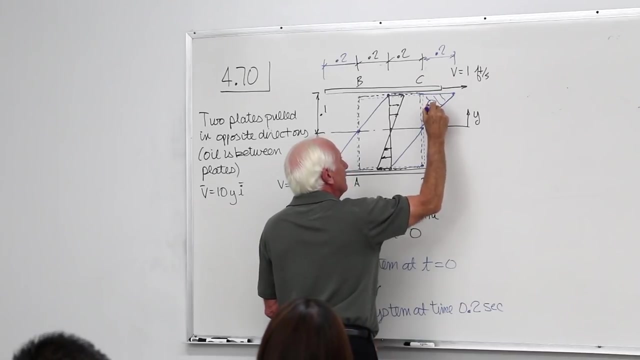 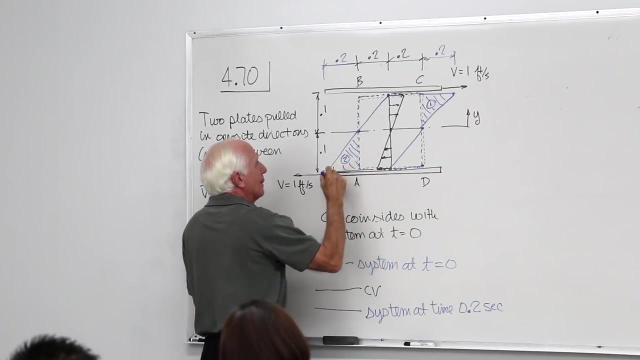 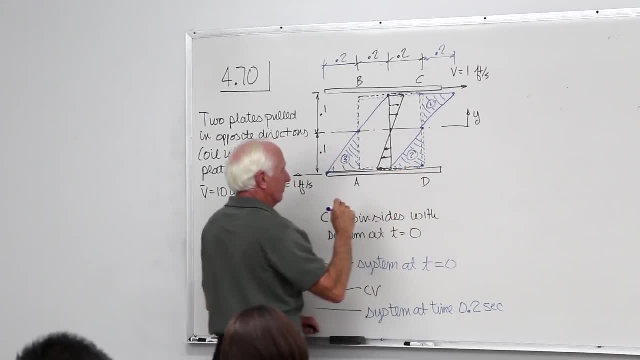 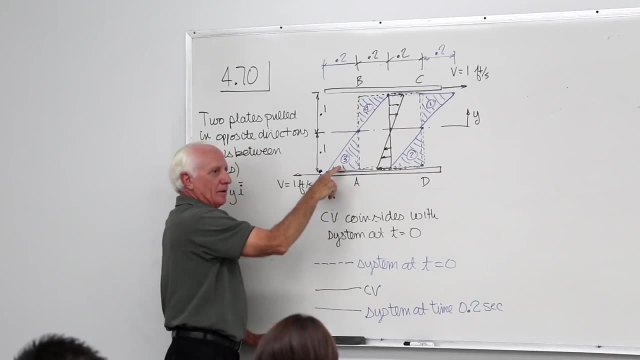 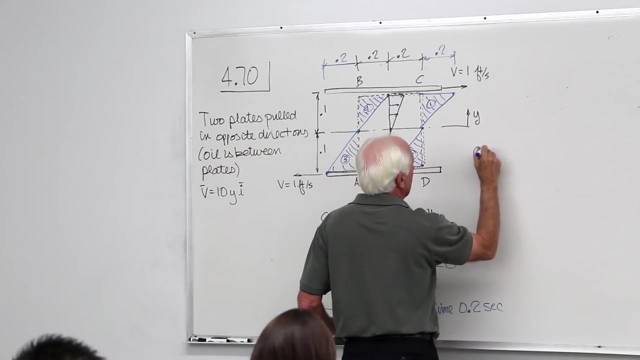 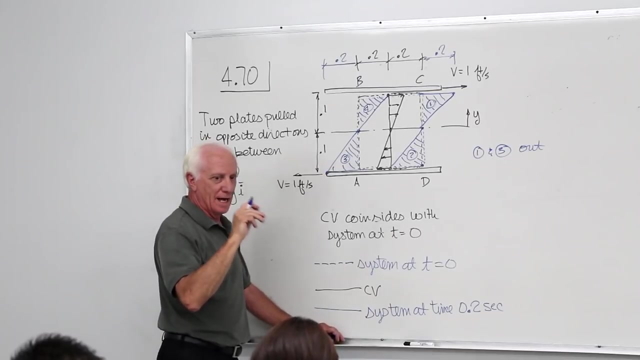 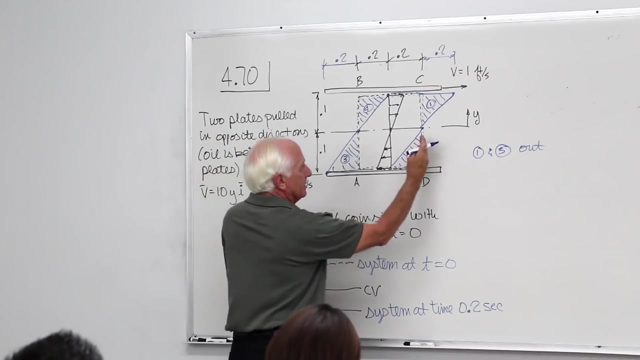 This is four. This is four, This is five. Three left, Two out, So one and three out. All those fluid molecules moved out of the control line. What came into the control line? these guys that were on the edge, they came in. 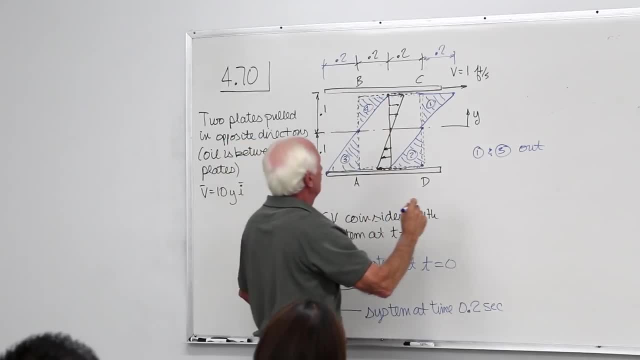 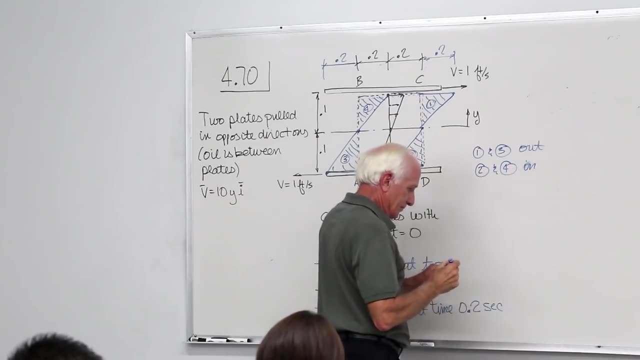 These guys that were on the edge. they came in. Two and four came in, So some fluid came in, Some fluid went out, Carrying the property, capital B. So again, what did we start out with? The control volume and the system. 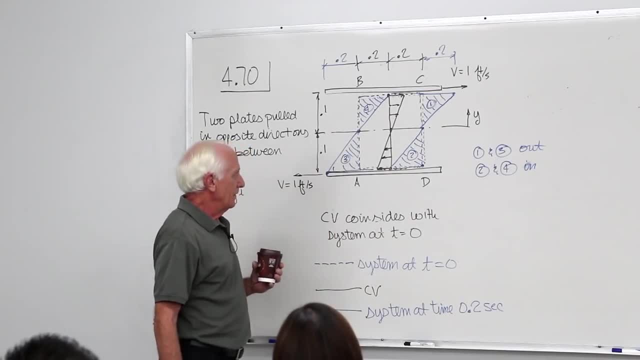 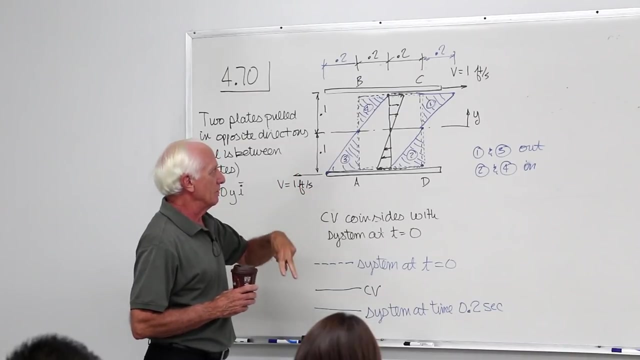 were coincident. Then what happened? You weighed 2 tenths of a second Draw the new system System boundaries. I did The solid blue line, Third part, Identify the amount of material that came in and went out of the control volume. 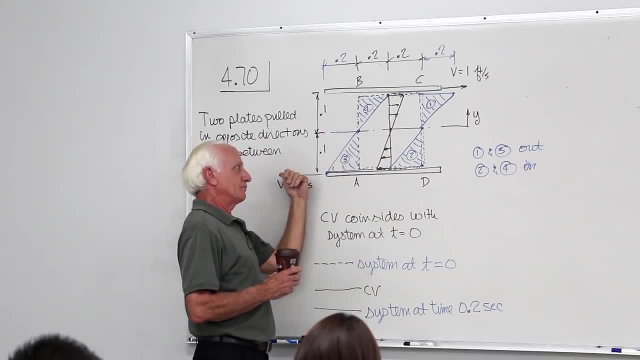 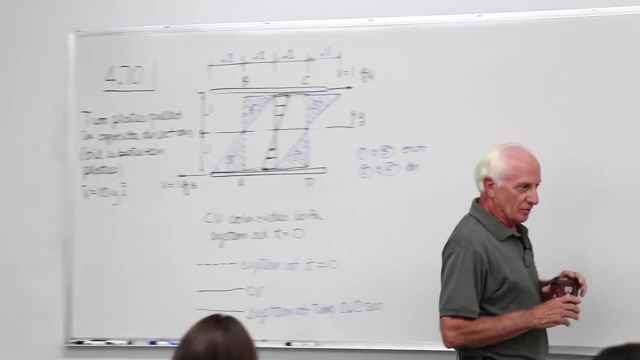 One came out of the control volume. Three came out of the control volume. Two came into the control volume. Four came into the control volume. Your problem homework is just a bump like that, but a different geometry. Identify the system after a certain 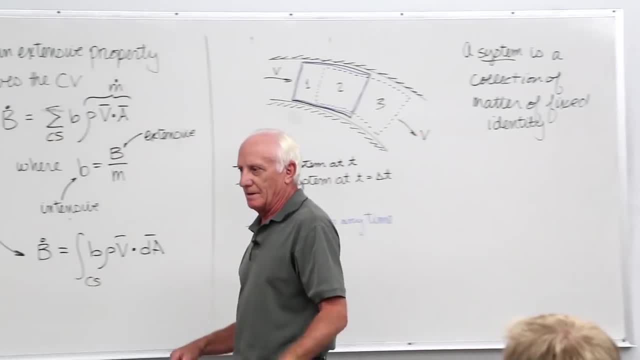 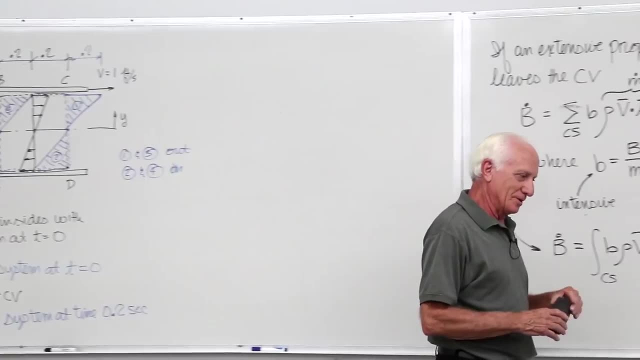 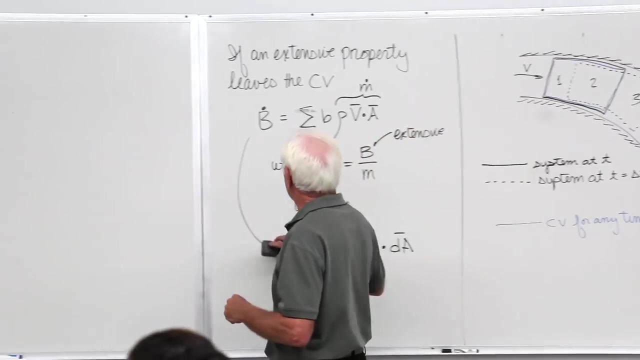 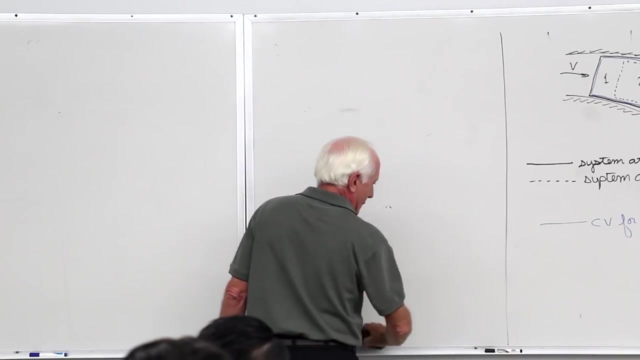 time. Show the stuff that came in and the stuff that left. Sketch it. It's just trying to explain to you about the Reynolds transport theorem, What it means. Our last step today, Our last step, is we're going to start with number one. 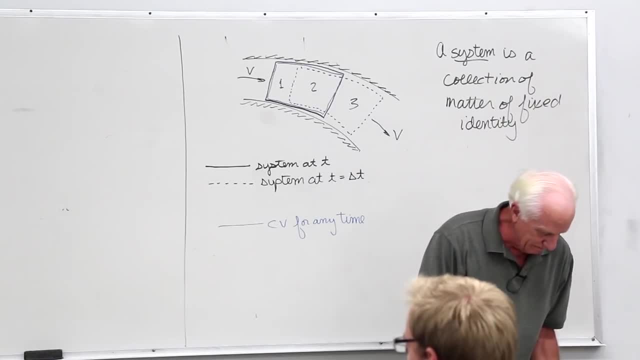 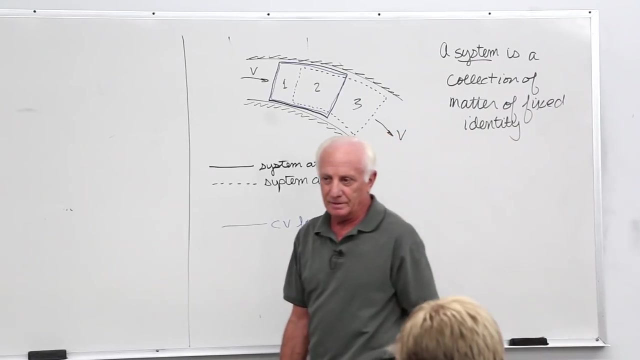 We're going to let B be a certain quantity Towards those three. it can be mass, momentum and energy. We're going to do all three Today. we'll take the easy one, Mass. Pretty easy for your hot water heater If you've got a gallon of cold water coming in. 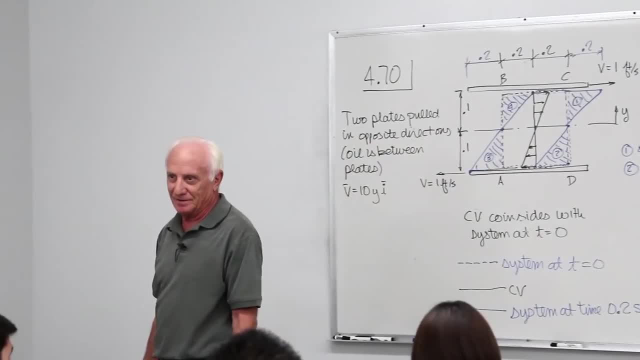 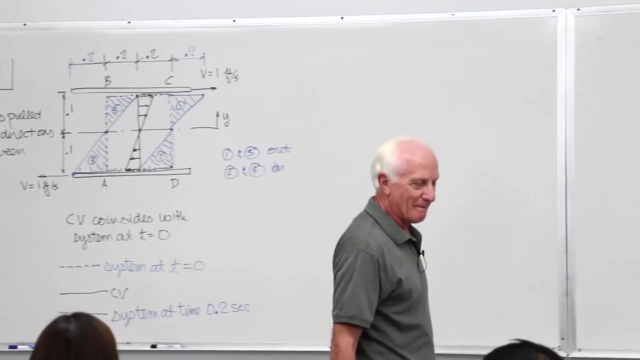 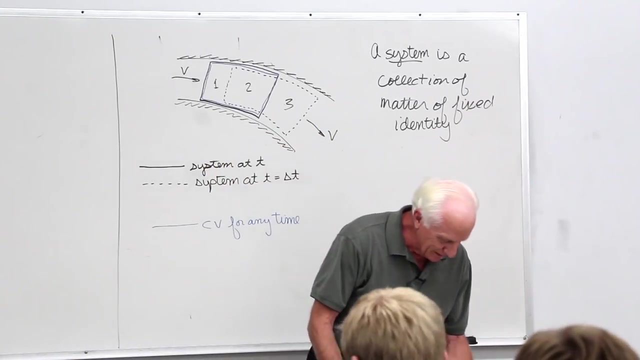 from the city. Guess what's going on. It's coming out to your dishwasher in the kitchen A gallon. Why It's steady state: What comes in equals what goes out. Some ways are pretty straight forward. Let's look at our mass, then. 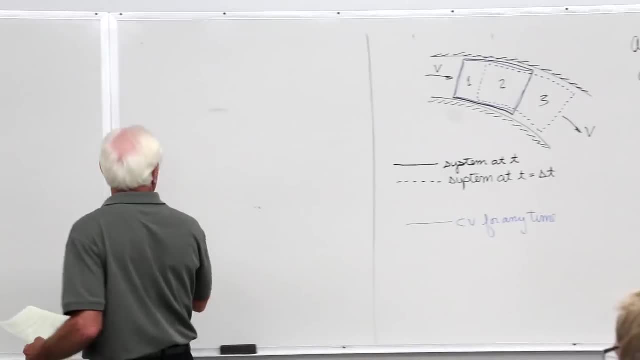 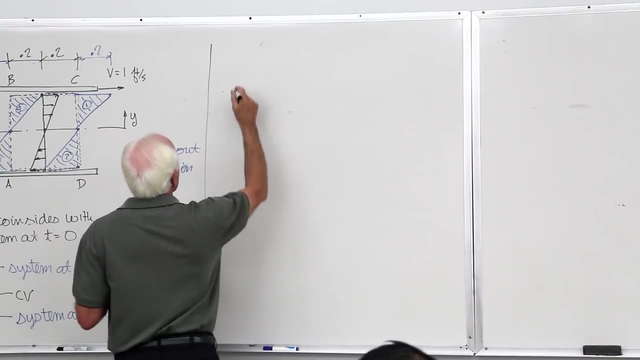 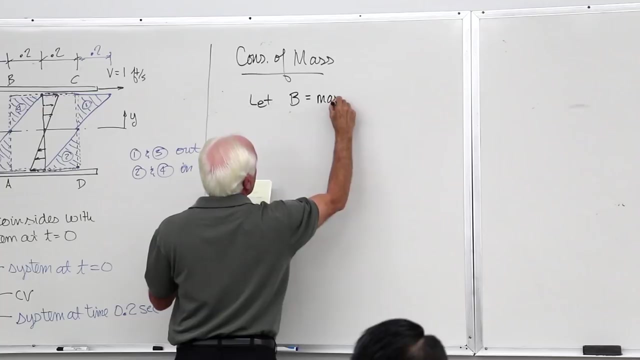 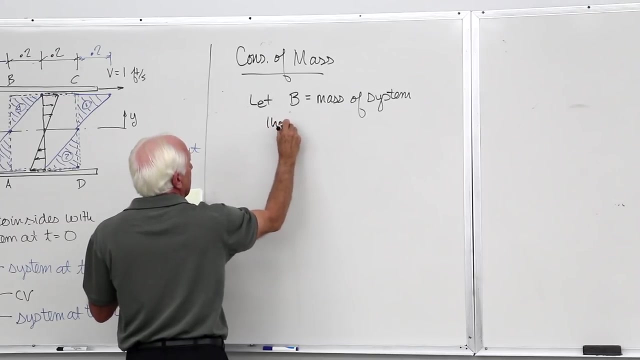 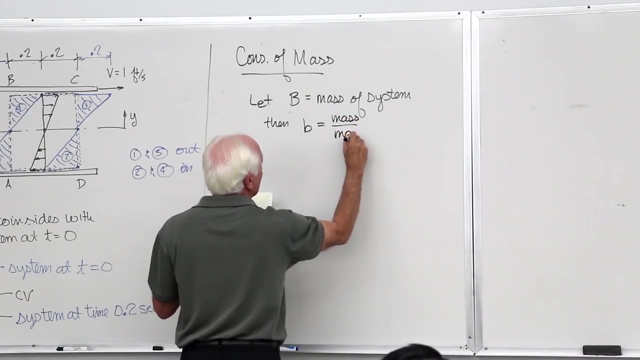 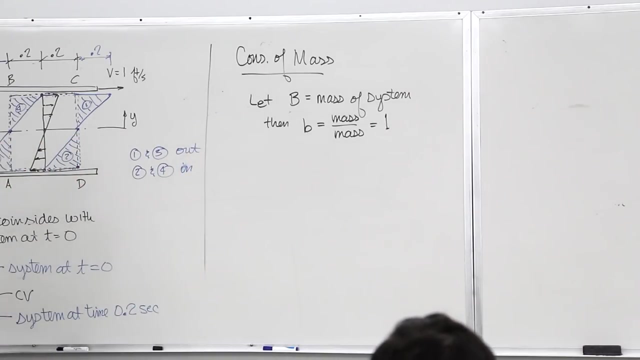 We'll call this continuity equation of conservation mass. Let capital B equal the mass of the system, Then little b equal mass of the system divided by mass. So of course little b just becomes one Kilograms per kilogram is one Dimensions, in other words. 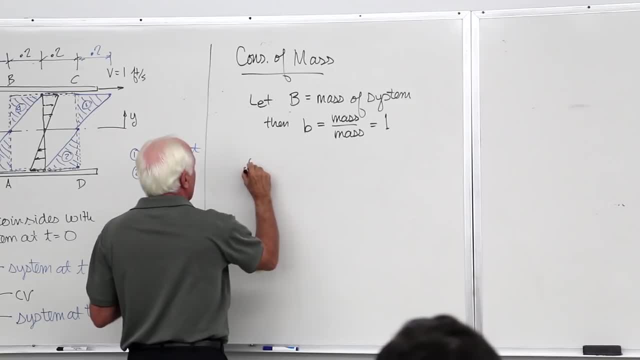 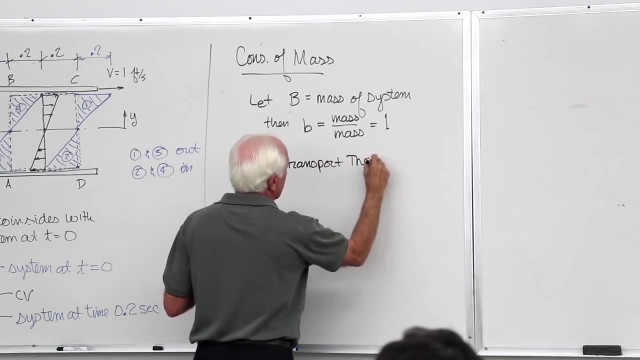 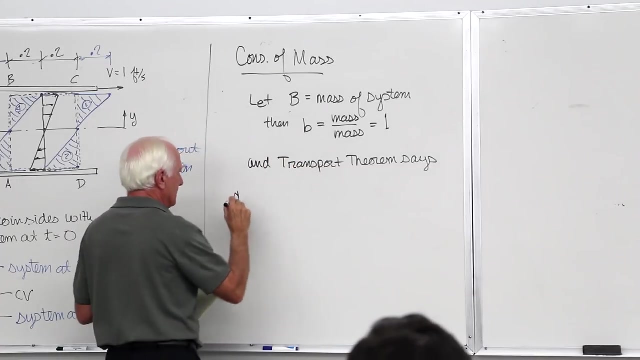 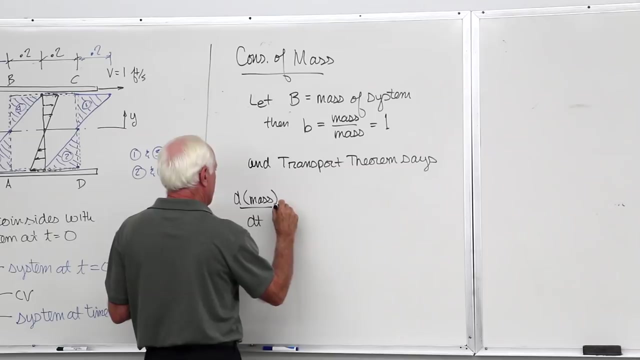 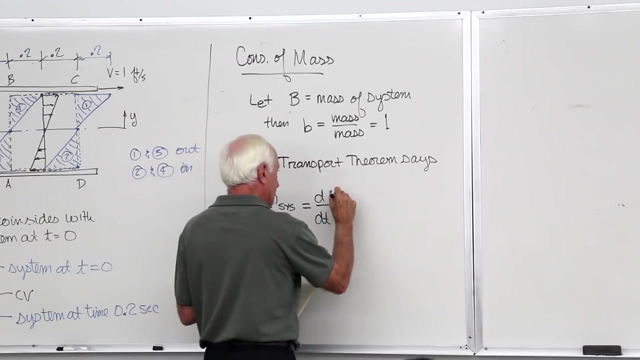 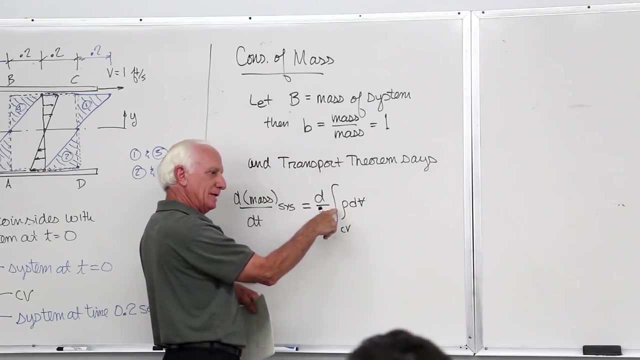 And the transport theorem says the following: Don't forget now: Capital B is the mass D, mass Dt Of the system, Equal d dt. This is the control volume. Don't forget: little b is one. So there was a little b in there, But little b was one. 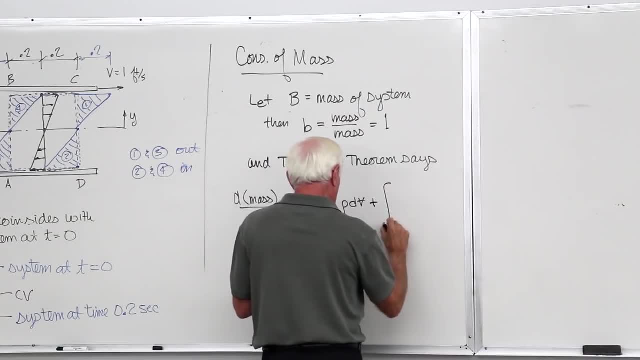 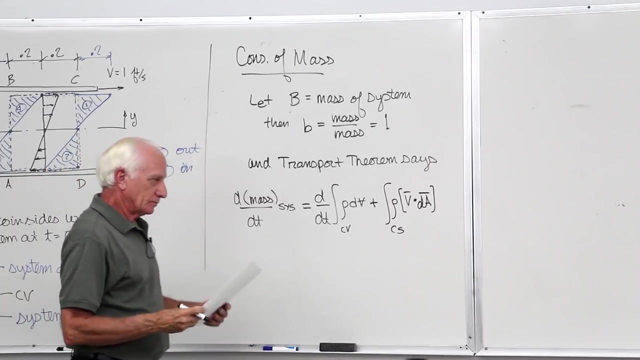 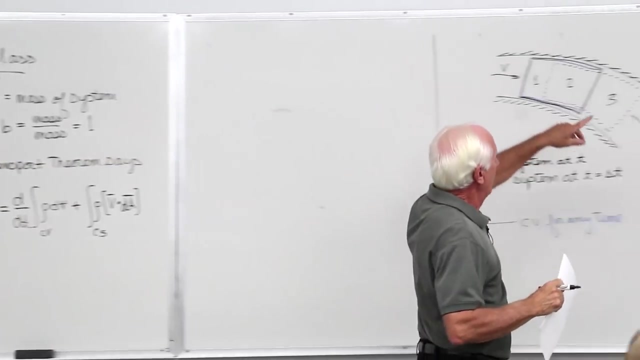 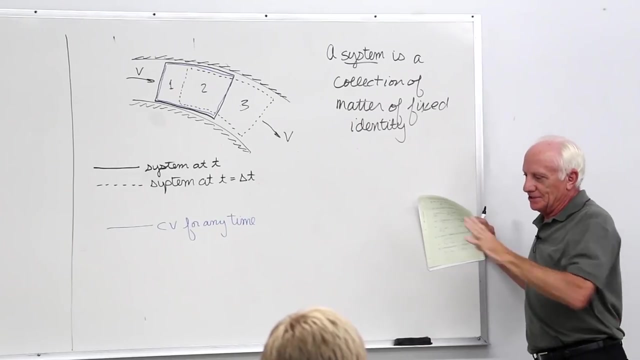 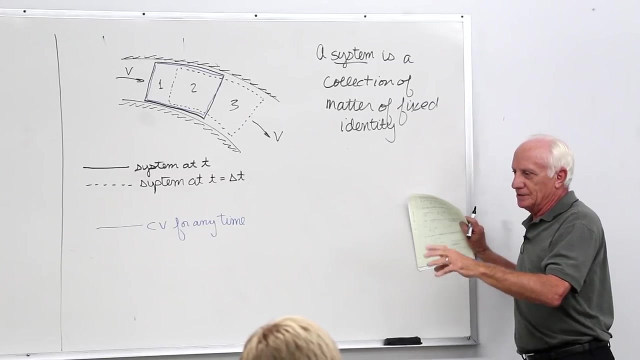 Plus integral over the control surface. Rho b, dot, da, d, a On a board. A system is a collection of a fixed identity. I showed you the pipe. If there is one pound of water at one minute and you tag them with some kind of spray paint. 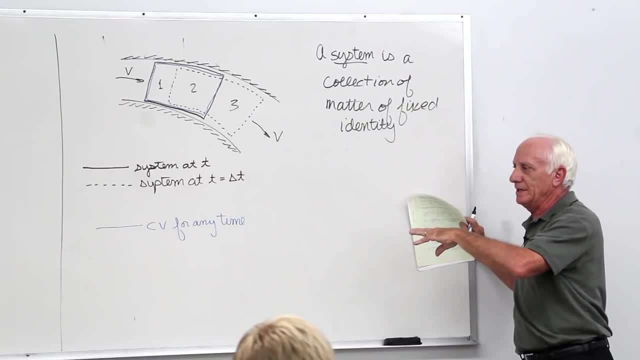 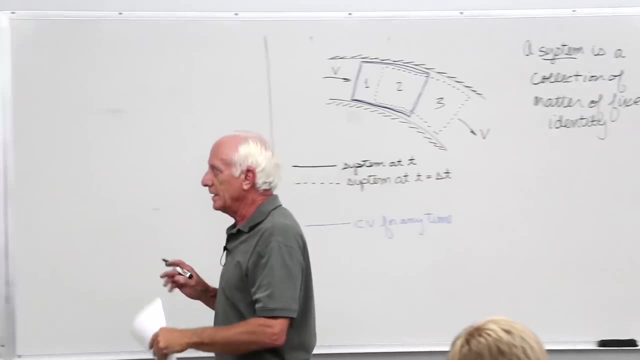 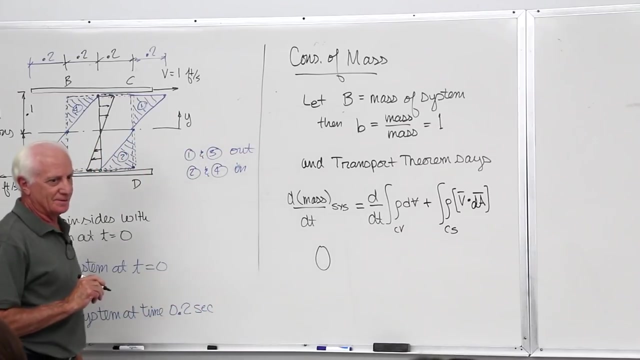 or something. After another two minutes did their mass change? No, Because you're following the same particles, So the mass is not changing. for what A system? So this term here is zero. That's the system. That's the system approach. It says conservation of mass. 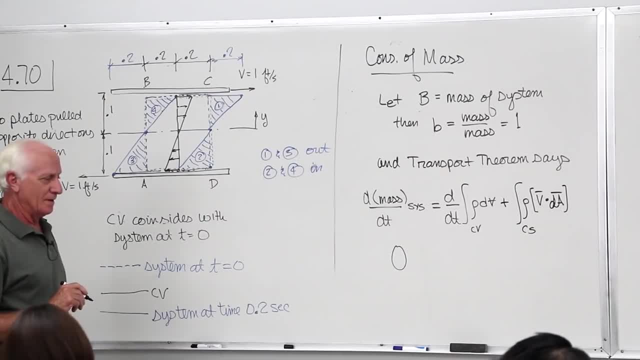 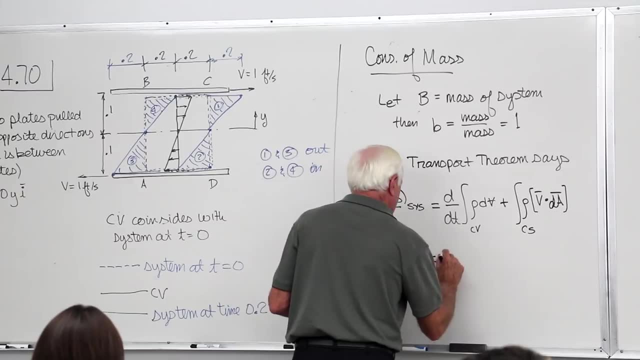 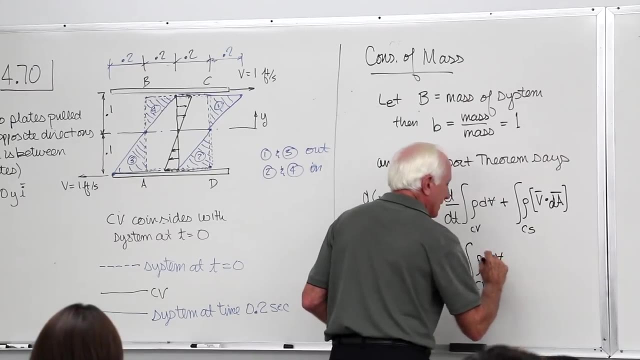 If we don't lose particles or gain particles, We have the same particles, Then their mass didn't change of the system. Okay, So now this becomes d, dt, Integral control volume. Rho, d, b- Don't forget, B slash is volume. 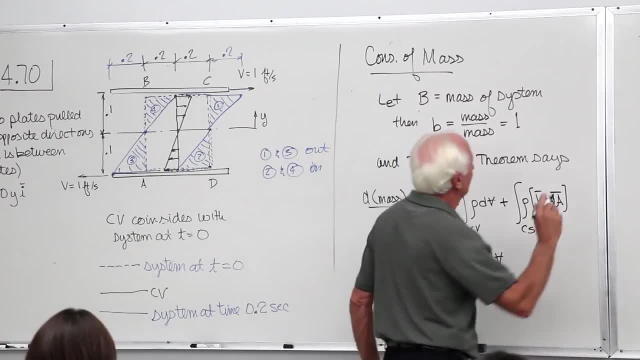 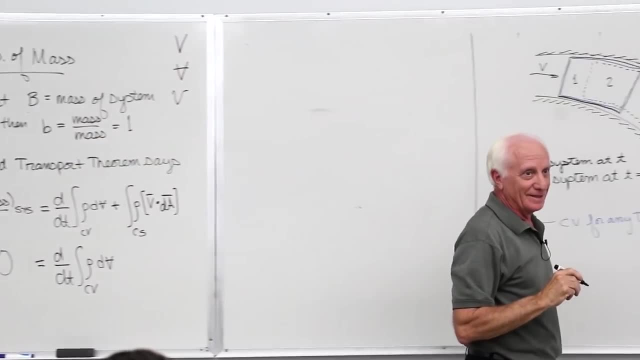 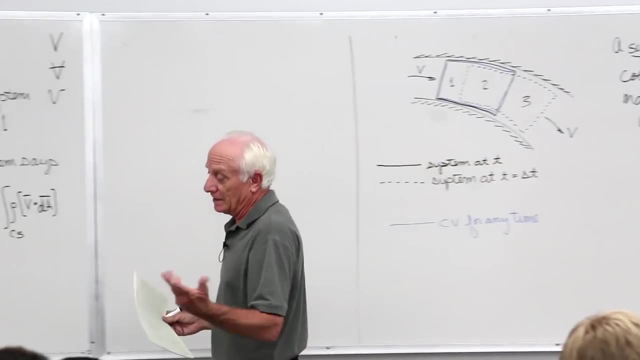 B- no slash- is velocity. Some people aren't too good about that And they don't make a little b very good. with a big B There's a difference. Little b is the velocity in the component velocity vector. It's in the y direction. What's big b? It's a velocity. 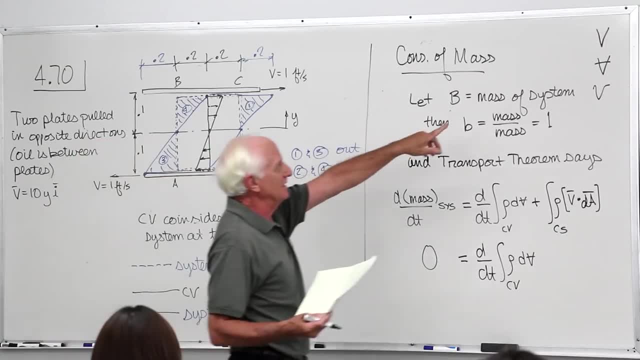 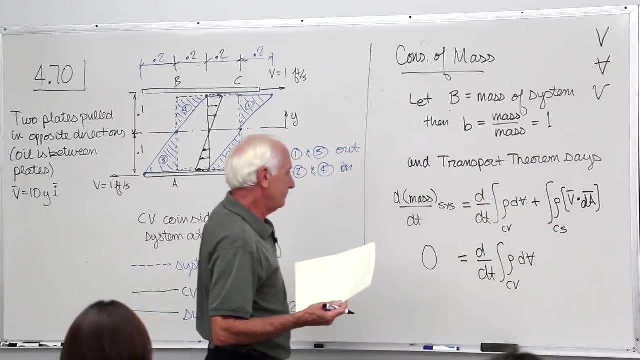 It might be the average velocity, We don't know. It's a velocity, But this guy is a specific velocity in the y direction And the b slash is a volume. Okay, Anyway, Back to here. I'm going to assume uniform flow again, to make things simple. 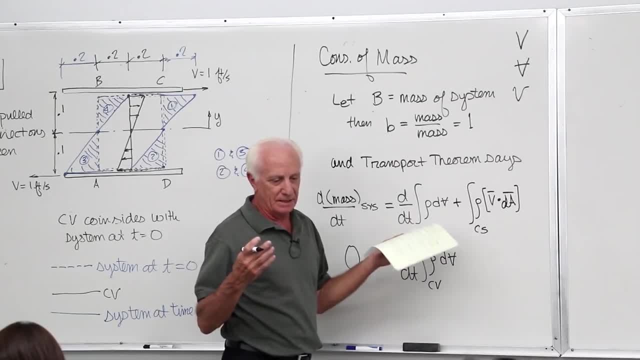 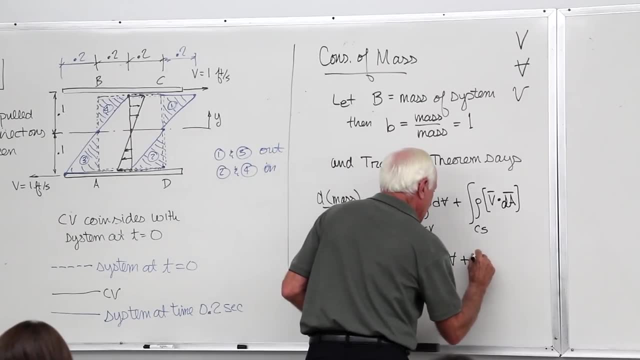 as we go through this. So our flow in whatever it is In pipes or whatever it is- Is assumed to be uniform. It doesn't change with the cross section area. So get rid of the integral and make it the summation over the control surface. 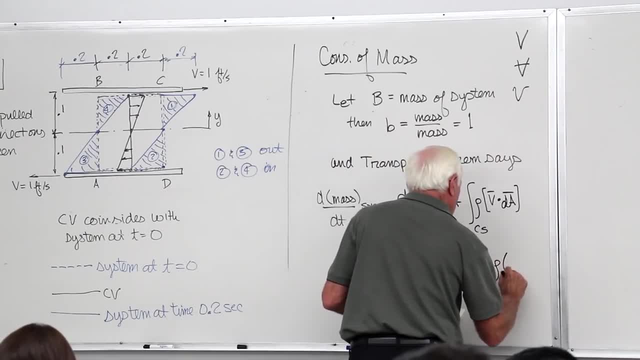 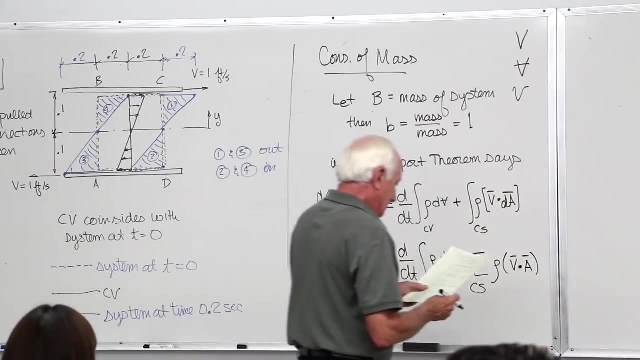 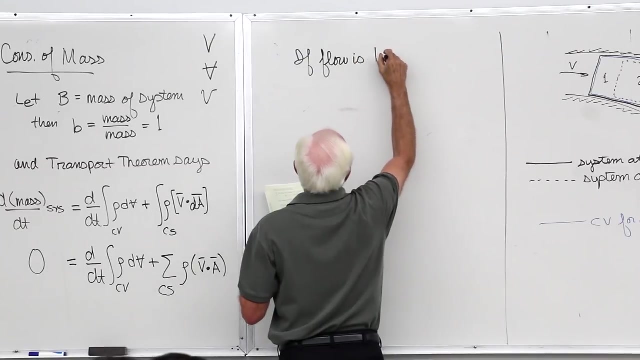 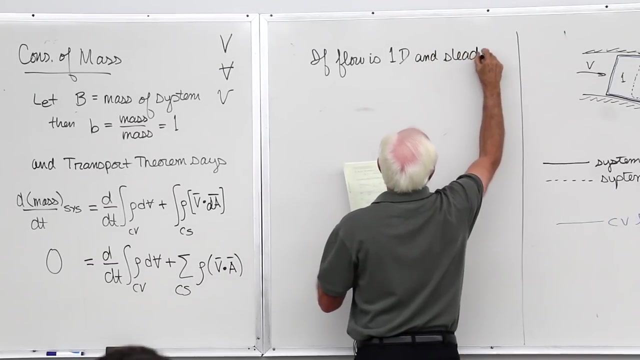 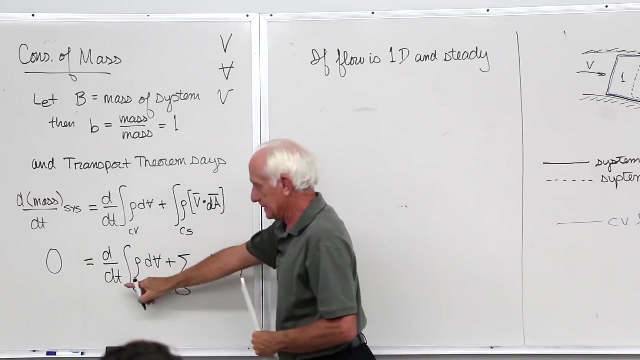 Rho b dot a. Rho b dot a. Okay, Now, If the flow is one dimensional and steady state, Okay Then, if that's the case, the steady state of this guy is zero. So this term here is zero. 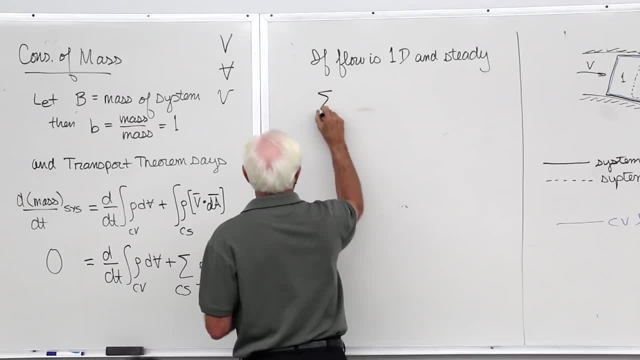 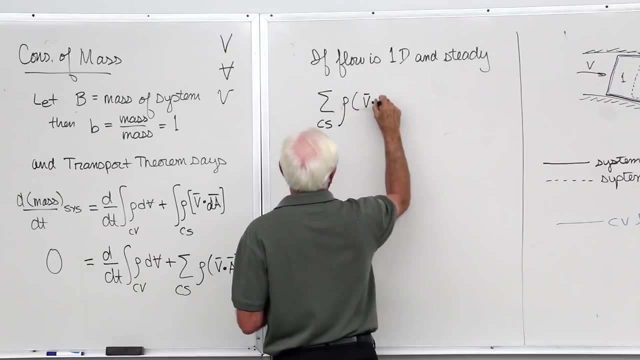 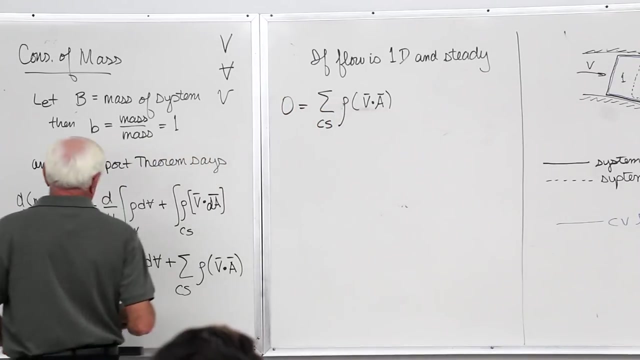 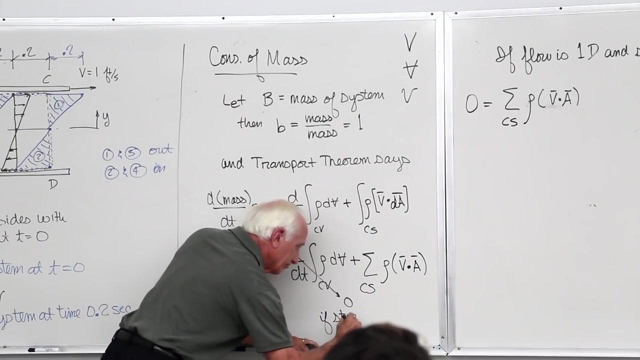 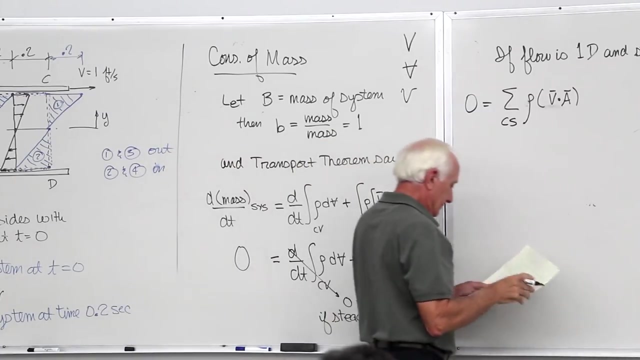 Okay, Rho b dot a, Rho b dot a. Don't forget, Those two terms are zero. I'll put it down here. So If it's steady and uniform, flow, one dimensional, Then we got this guy right here. 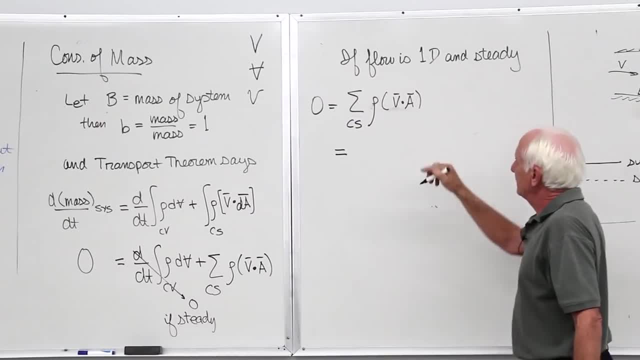 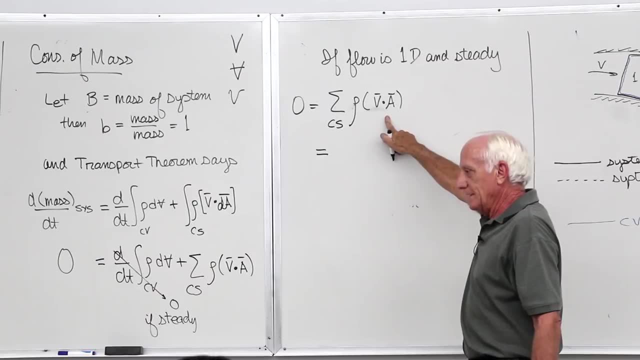 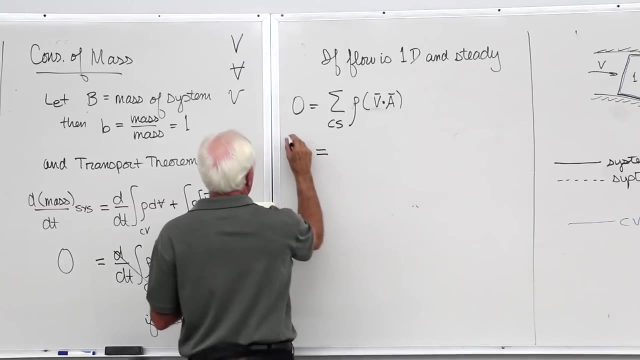 Well, don't forget what that is. I had it before. It's in your notes. This guy here is a mass flow rate, Don't forget. If it leaves, it's positive, If it comes in, it's negative. So this is m dot. 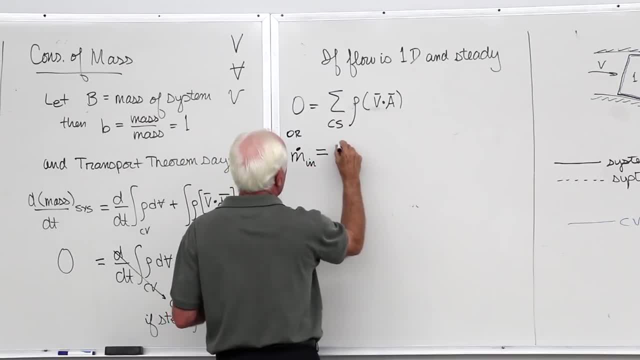 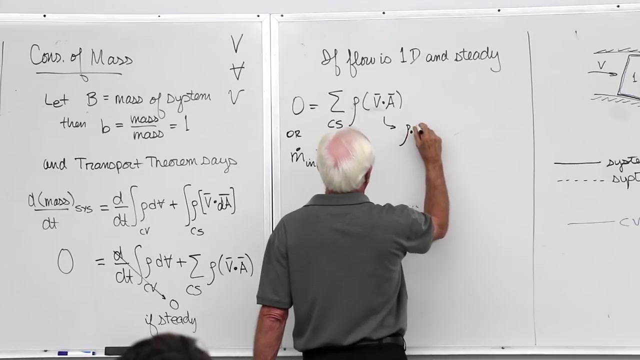 n equal m dot out. If you want to do it officially, then it looks like this Outflow is positive. So rho out Rho out b out a out, Minus. If it comes in, it's negative sign. 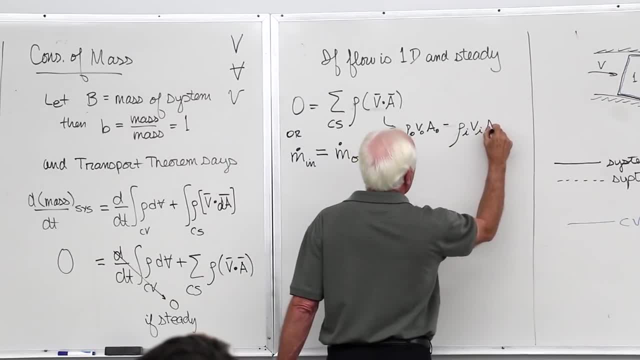 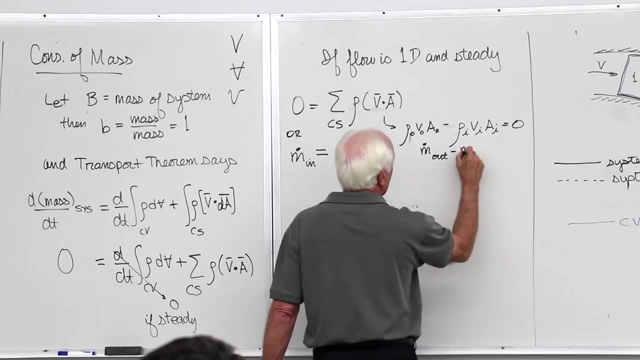 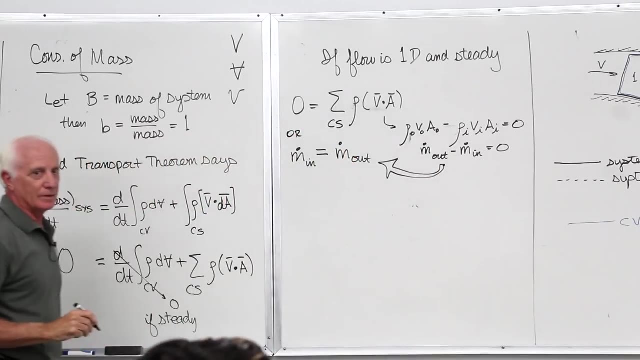 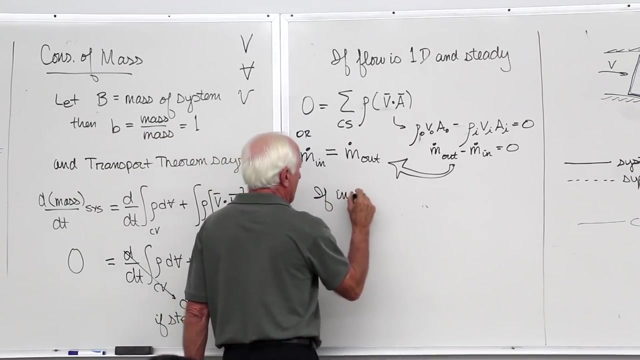 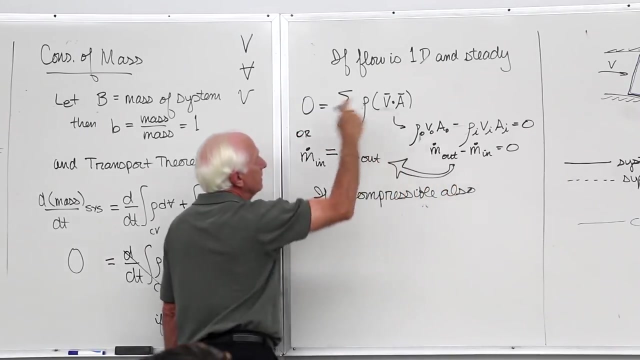 Rho in b in a in Equals zero. m dot out minus m dot in equals zero, Which gives that guy right there. Okay, Next step, If it's incompressible, also Besides b: 1b instead. 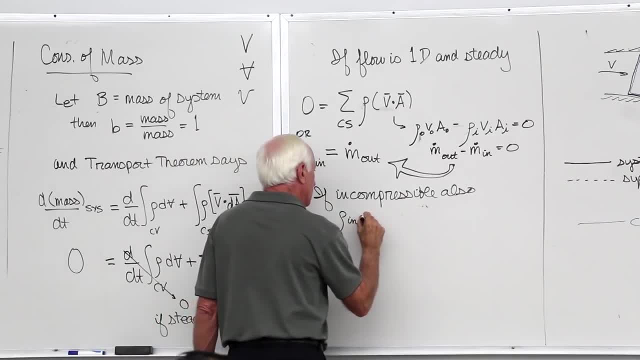 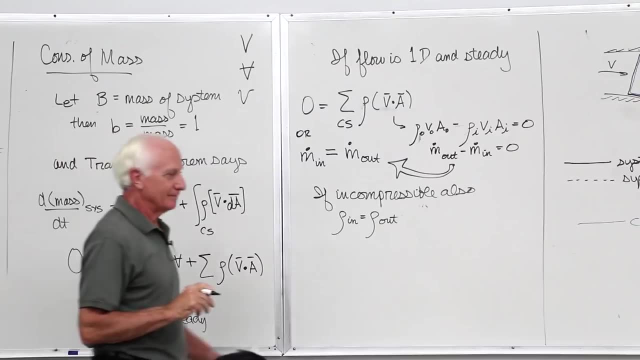 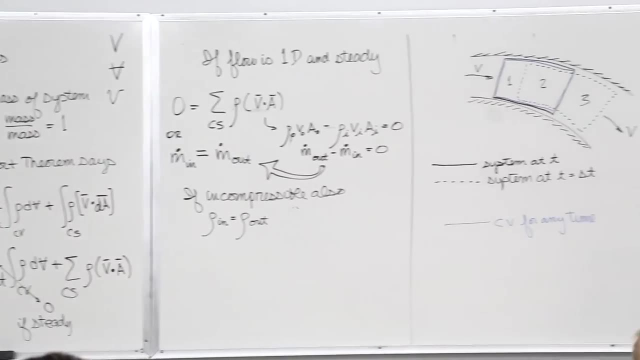 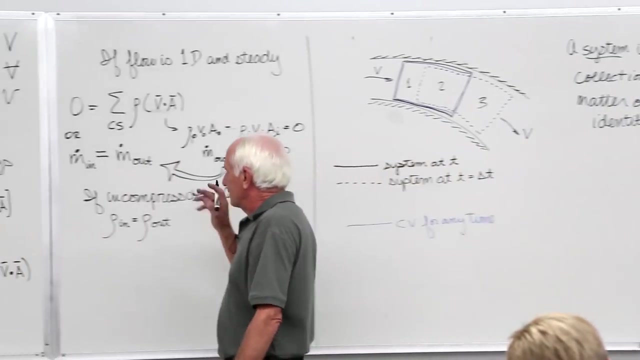 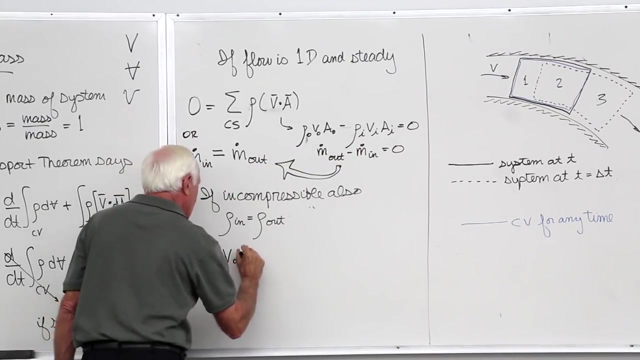 Okay, Rho in equals, rho out For steady flow. Okay, So here we go. Cancel out the rows. Cancel out the rows. So: b out, a Out, A out Equal. b in a in Rq out. 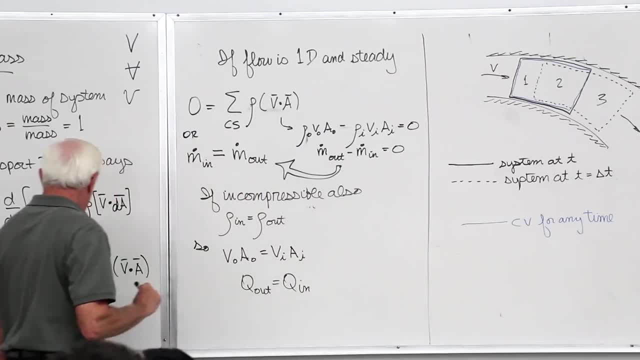 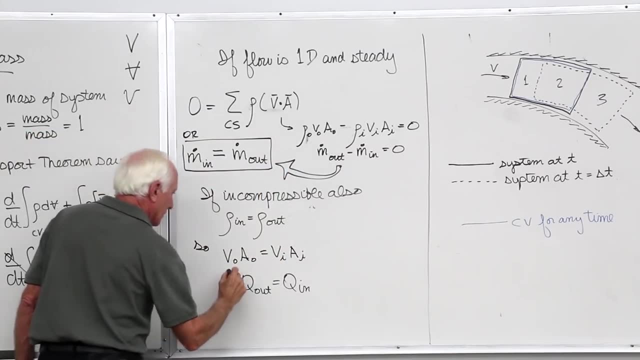 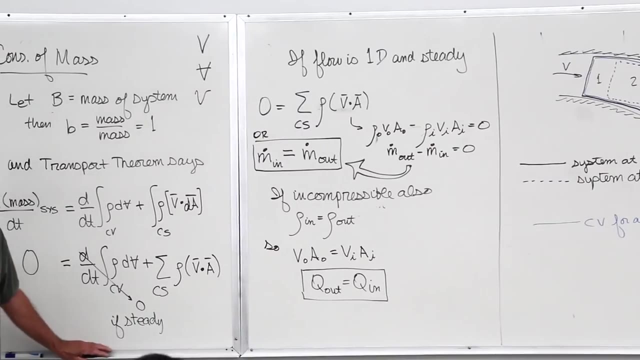 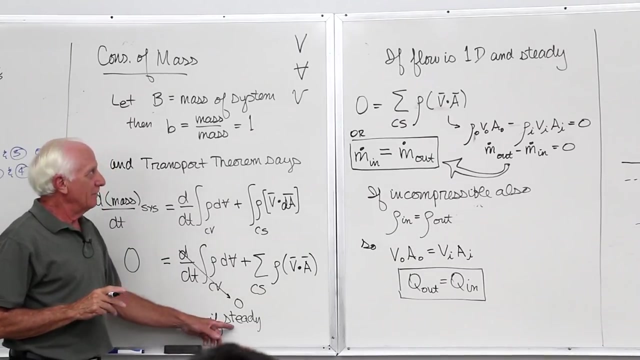 Equal q in: Okay, Approximately. Okay, Those equations carry with them some assumptions, And they better be true. Okay, Those equations carry with them some assumptions, And they better be true, Or don't use them. Number one: Steady flow. 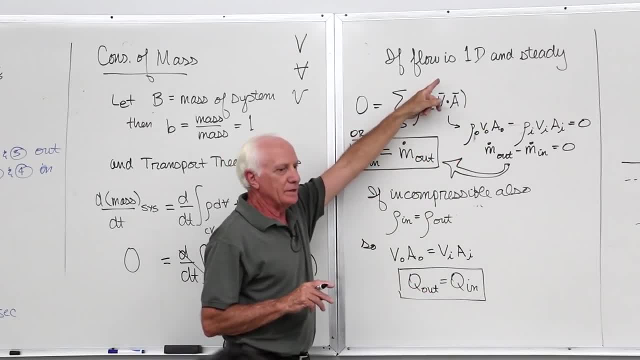 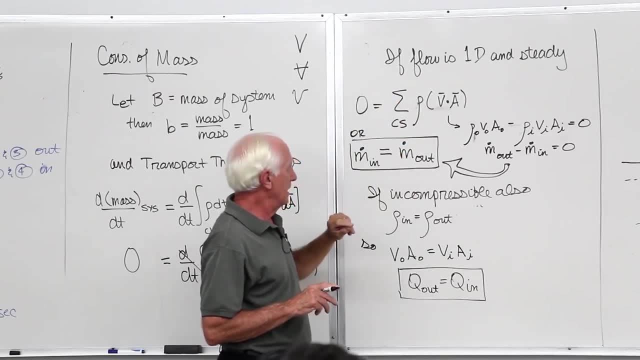 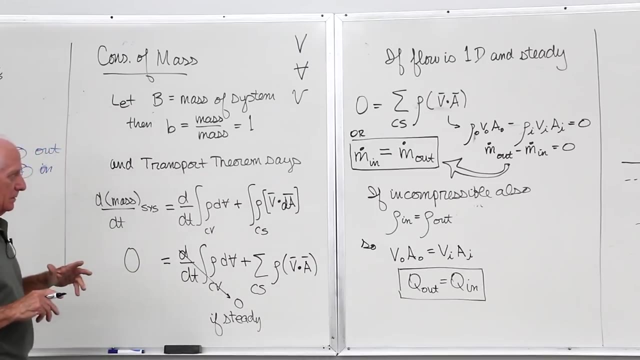 Number two: Uniform flow, 1b flow. If those two are the assumptions you can make, then m dot in equals m dot. out Of what? The control volume? If the flow is incompressible or it can be treated as incompressible? 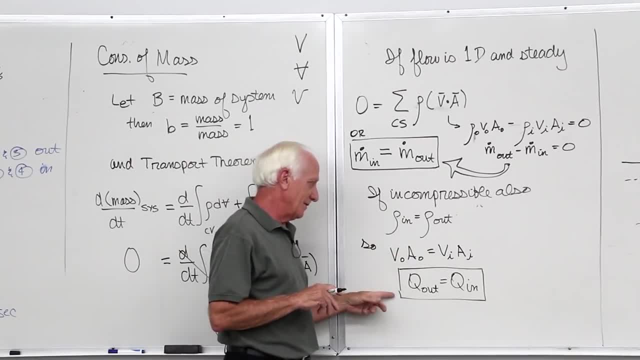 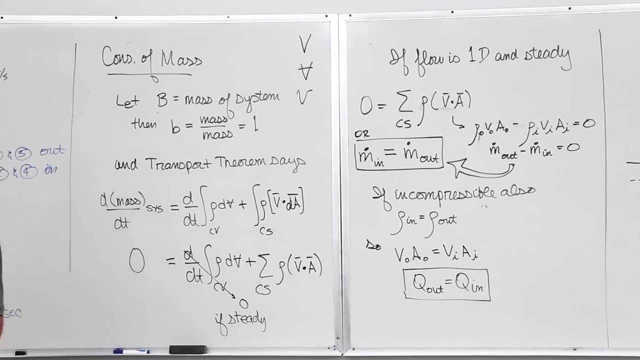 then the densities are the same in and out. Then you can say the volumetric flow rate in equals the volumetric flow rate out. That's what I said. If one gallon of water goes into your hot water meter- cold water- guess what happens? 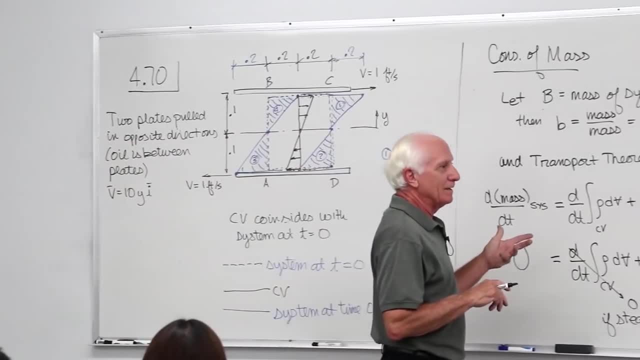 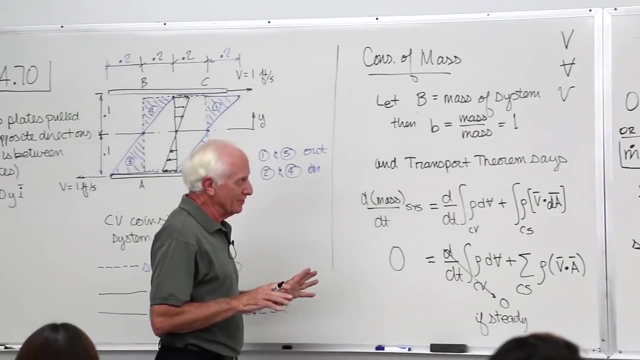 One gallon of hot water is out the other end. Why? Because in your hot water meter the flow is steady, 1d and the fluid is incompressible. But if those aren't true, you have to go back to the basics, like this: